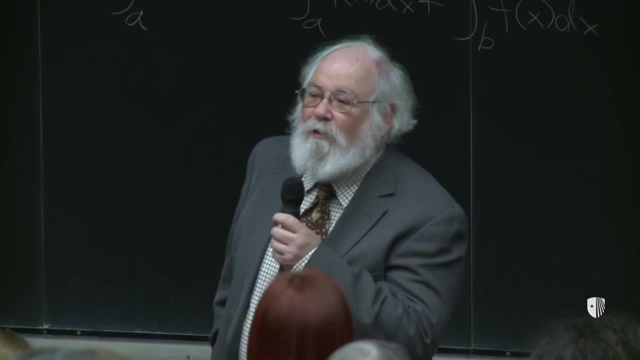 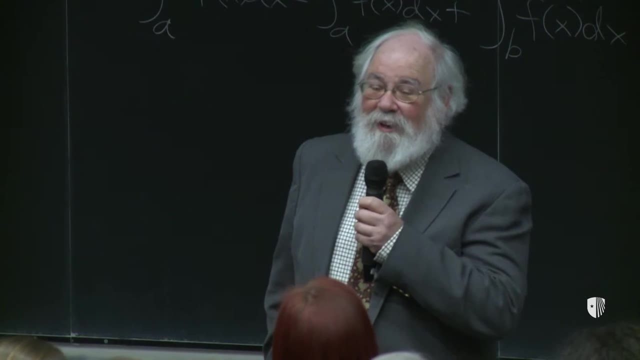 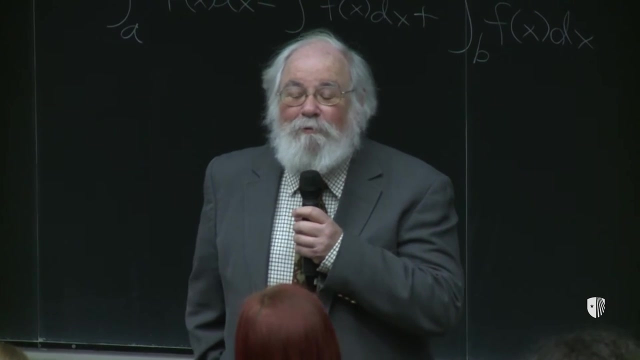 by the Department of Ecology and Evolution, and also the Science Open Nights System, which has been in operation for, I think, over 35 years, when an astronomy series started a long time ago And I think the Living World series has been going for about 15 years. 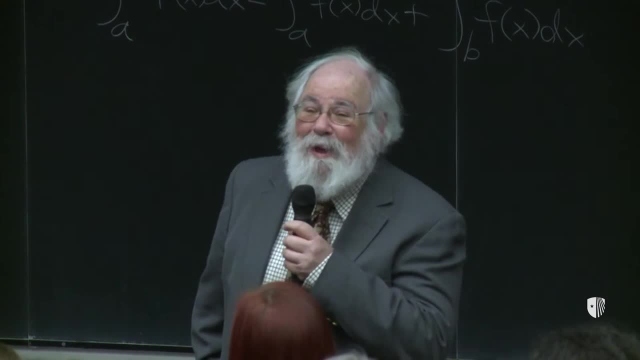 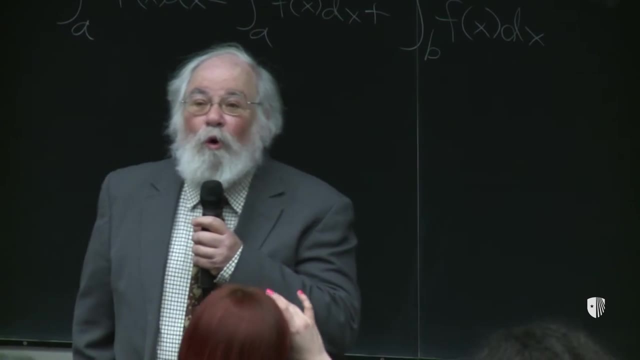 So it's amazing how none of you have nothing to do on a Friday night, but we welcome you here And all I want to do is to tell you about the only other Living World talk that's going to occur. We only have one other. 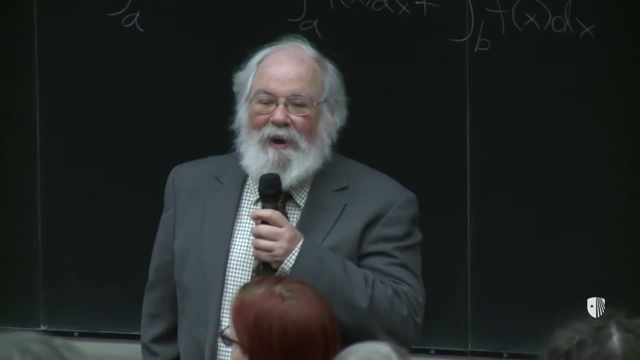 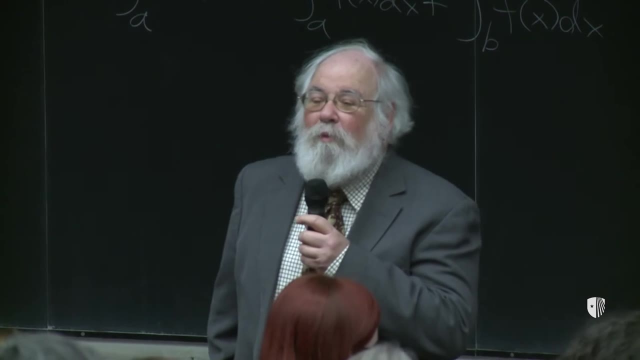 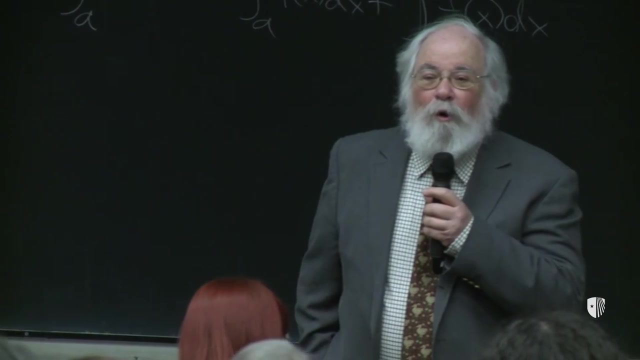 this spring and it will coincide with Earth Day, which is April 22nd, which is a Friday, and will be 7.30.. It will most likely be over in the Wang Center auditorium, But if you Google Living World and Stony Brook, you will find out the information very soon And we're going. 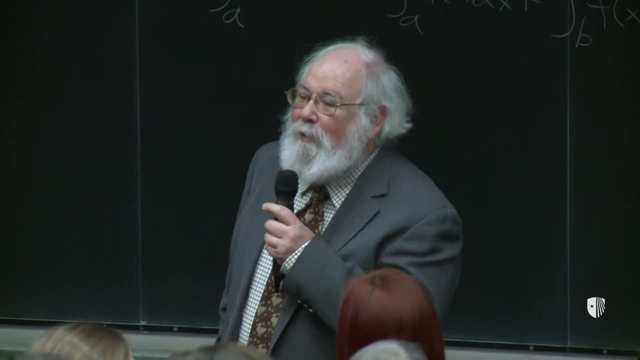 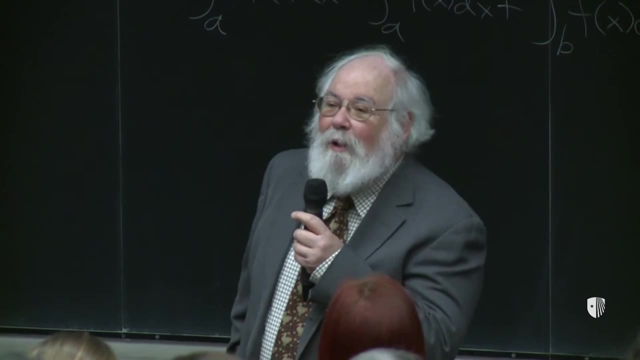 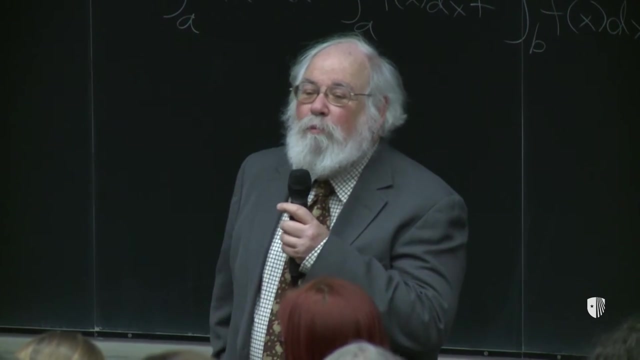 to have John Warner, a real wizard, a genuine certifiable wizard, a green chemist, the principal of the Warner Babcock Institute, And what they do and what he has accomplished is really remarkable for both the quality and the breadth of different types of green chemistry initiatives. 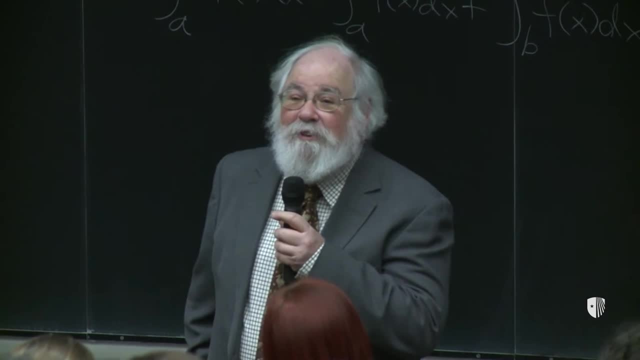 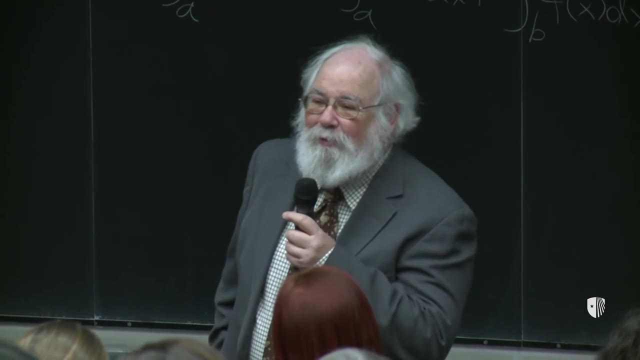 he has undertaken and succeeded at. He's a remarkable person, Thank you. If you want to learn a little bit about him, just Google John Warner, green chemist, and you'll learn an awful lot about this wonderful person who will be speaking Friday evening. 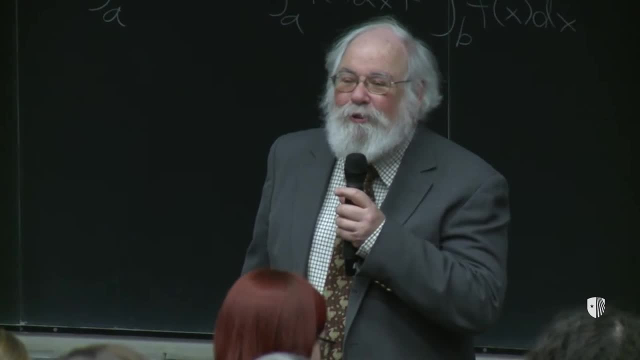 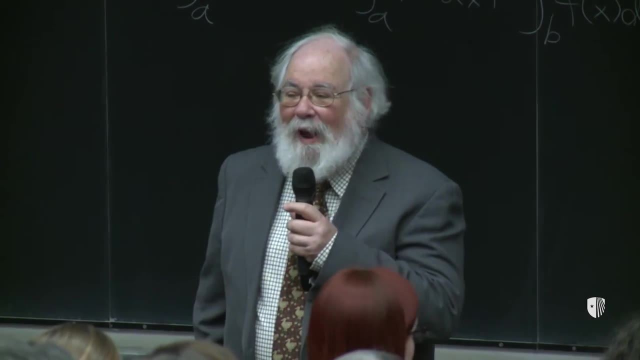 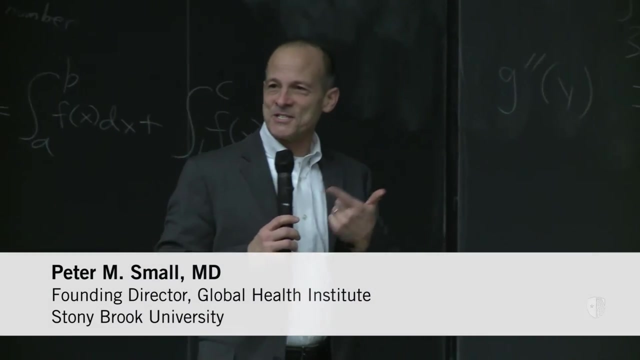 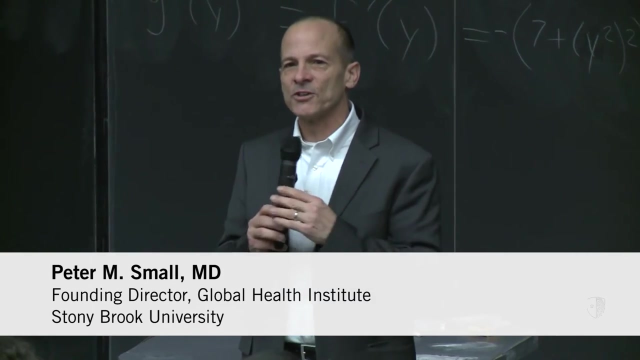 So that's all I want to say, except I'm now going to introduce Dr Peter Small, who is the head of the Global Health Institute at Stony Brook. Thank you, I will continue the microphone charade, And Provost Asanas has asked me to come and express his regret that he couldn't be here. 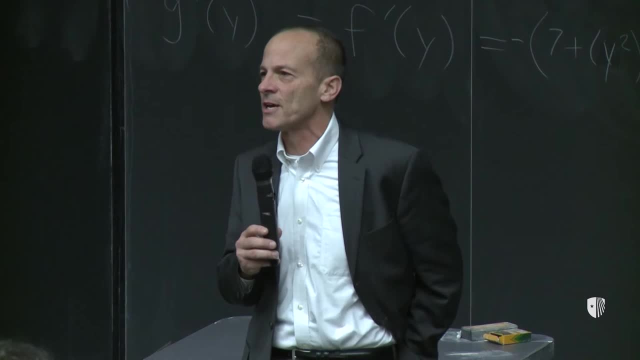 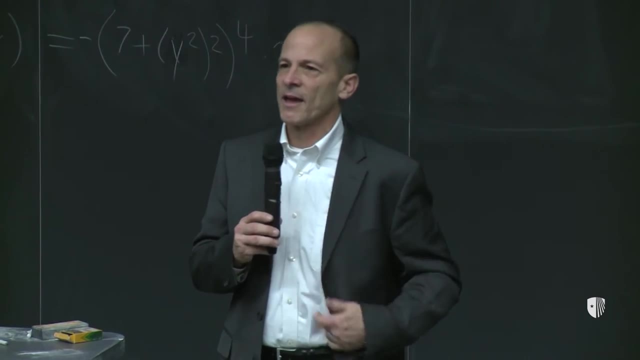 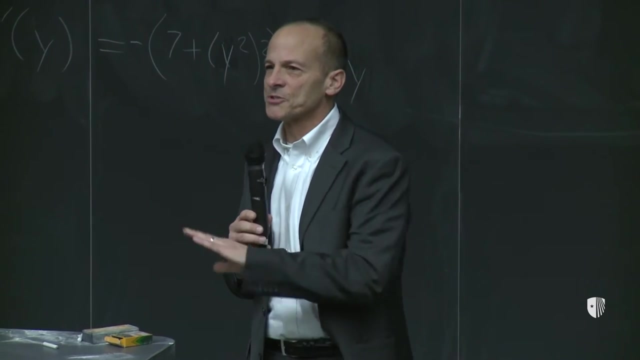 this evening and also to just say a couple of words about the history and the significance of Darwin Day. So today is the 207th birthday, or celebration anniversary, of Charles Darwin's birth, And he was a remarkable scientist, One of the few scientists who was actually Capitol Hill's. star, That's aもの. It's a remarkable scientist And he was actually very successful when he was an American scientist And he was an extraordinary scientist as well. He had an extraordinary career. He was one of the most prestigious scientists in the whole world and he had a history of my 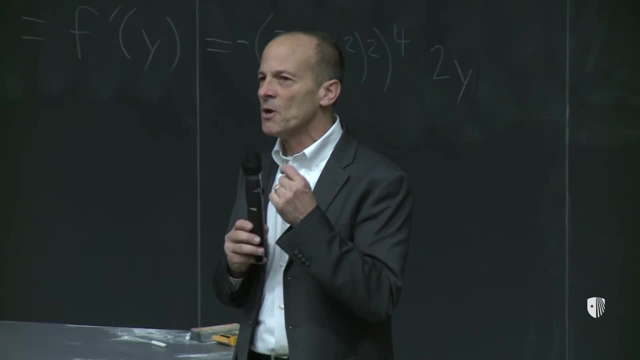 life, that is to say of all things, when you look at Darwin Day. And he was one of the few scientists who did the greatest science, the greatest science in the world, and scientists who really changed the paradigm who, like Copernicus before him, came up with 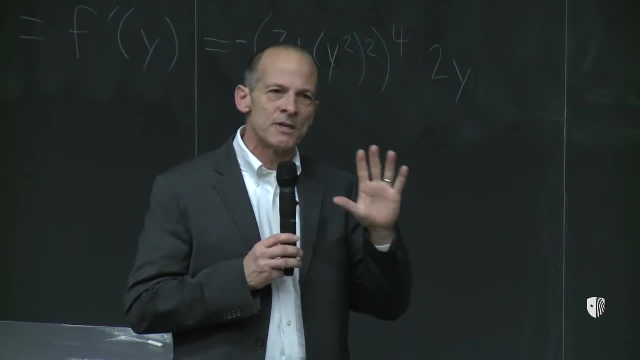 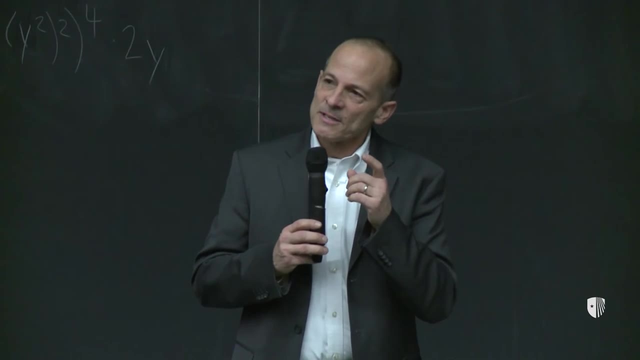 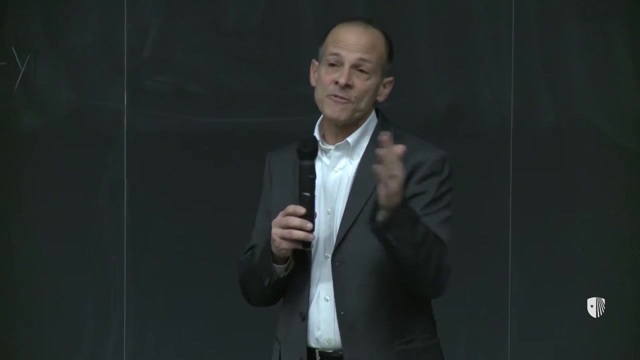 a simple concept that unified an incredibly complicated set of observations, And really one of the few people who have come up with ideas that truly permeate biology or any field, and, for example, in biology, I think nothing makes sense in the absence of evolution. 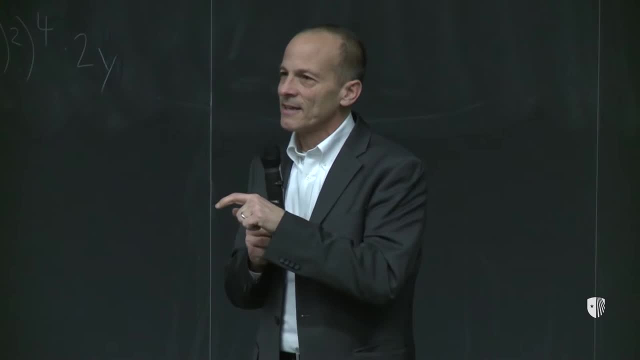 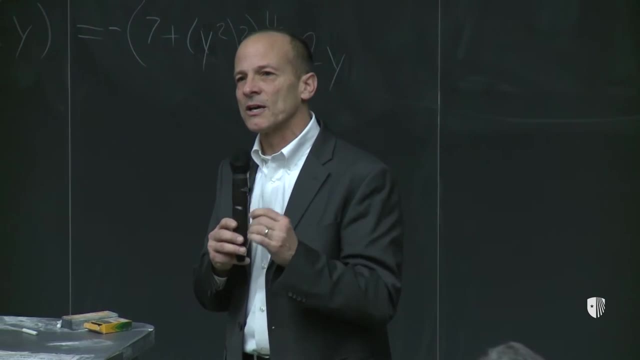 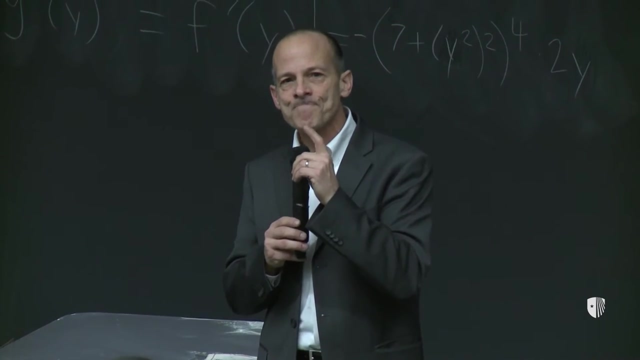 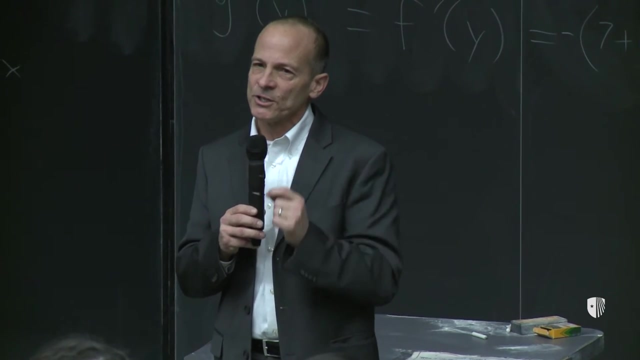 And yet evolution, like the idea that the Earth was at the center of the universe, was a concept that was hard for people to accept. And here we are, about 150 years since The Origin of Species was published, and half of America still does not believe in evolution. 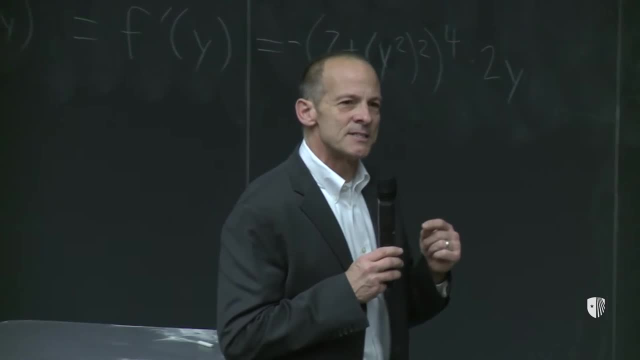 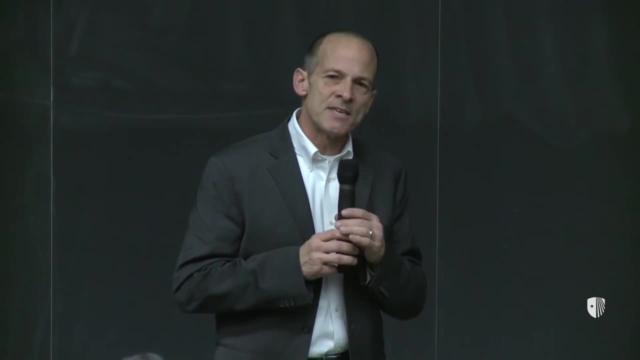 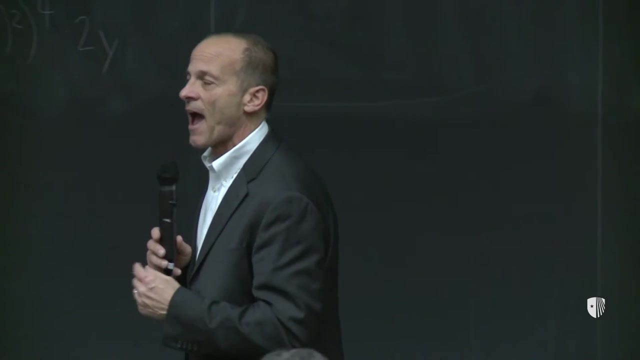 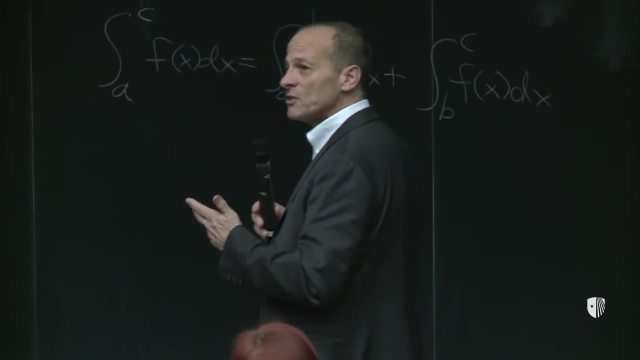 And I use the word believe intentionally, because it's actually really more about faith than science- and I think that if you look at the alternative models, like intelligent design, they actually simply don't fit the facts. And yet creationism is still believed and even taught in many schools across the United. 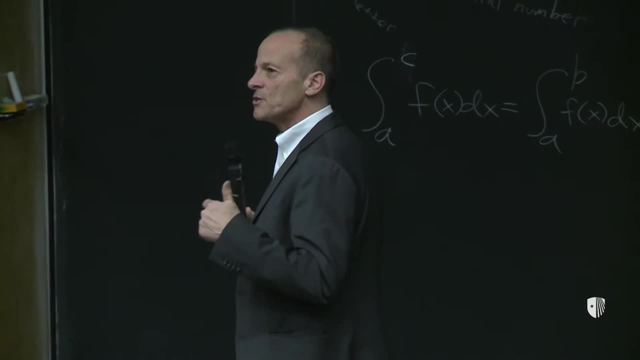 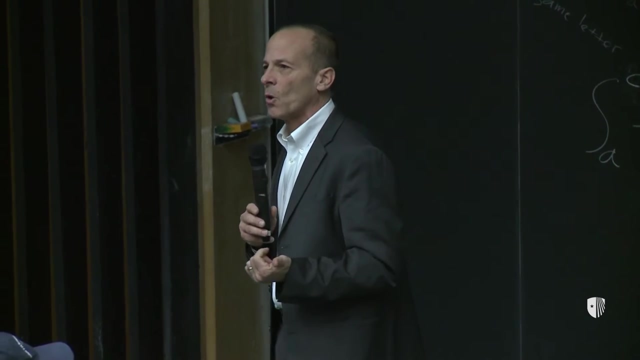 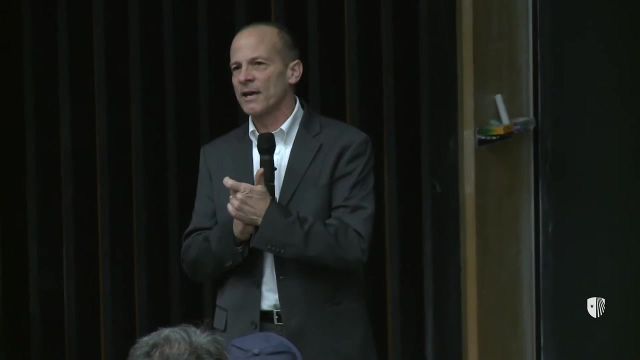 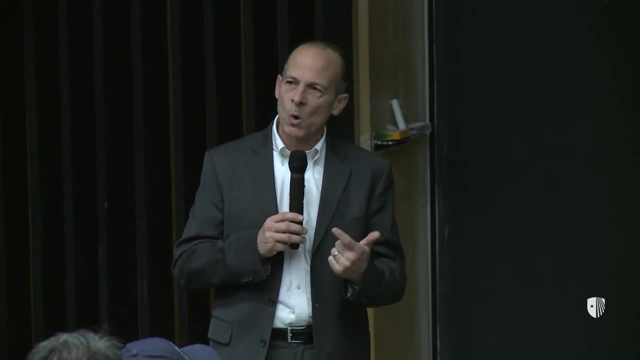 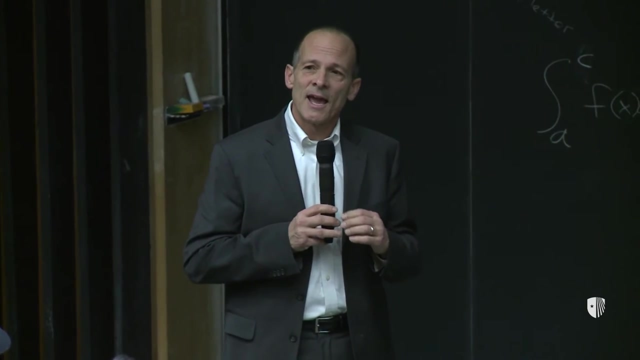 States. But actually for me, Darwin Day, Darwin Day is about much more than the celebration of a man or even the tension and battle between science and religion over the origin of species. For me, Darwin Day is at its core about scientific illiteracy and denialism. 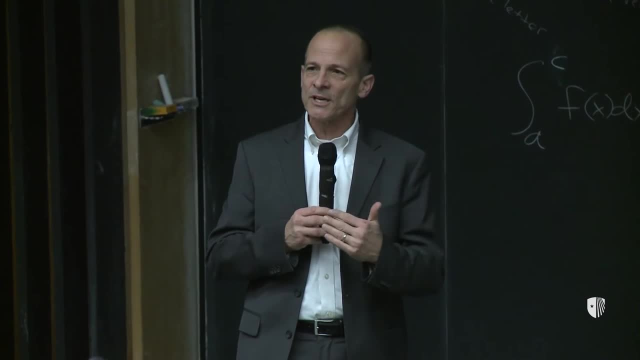 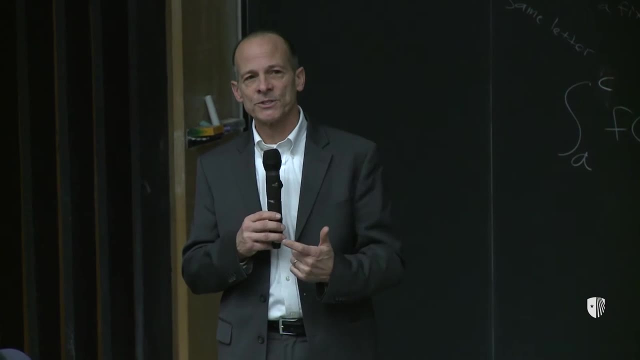 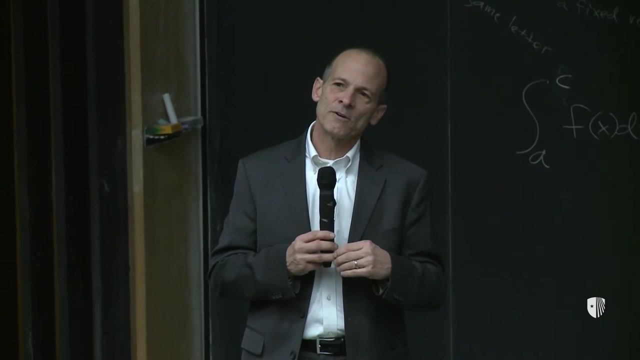 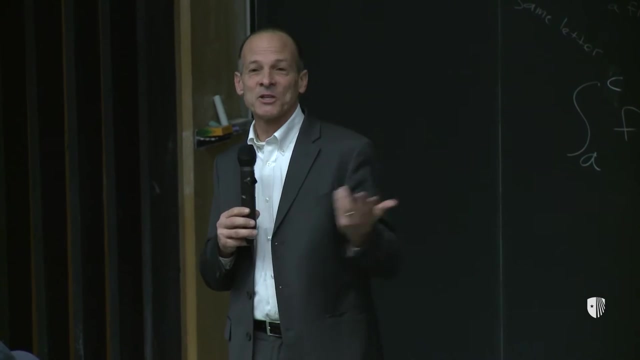 And You know, We as a country and globally, as citizens, do a terrible job of teaching scientific literacy and are surrounded by denialism of very, very fact-based facts like global warming. And, in fact, although I'm very interested in hearing tonight's speaker, but my intuition 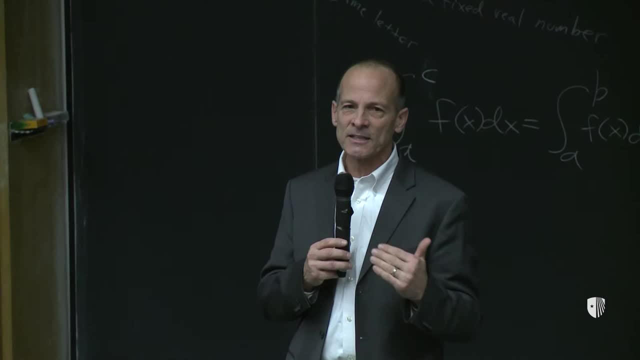 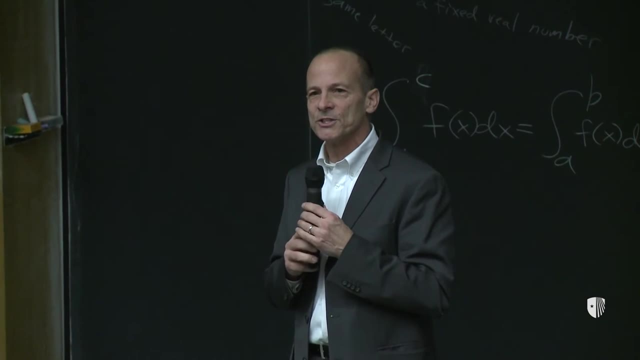 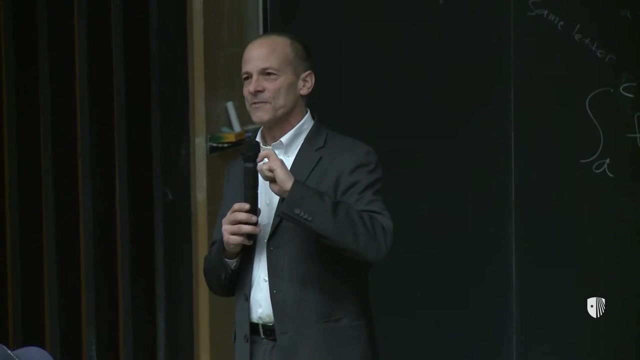 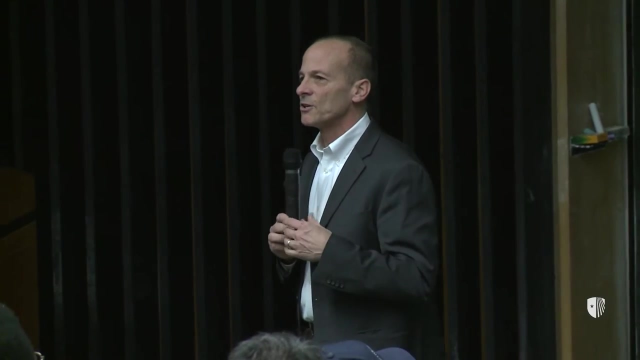 is that it's actually Scientific. denialism probably poses one of the greatest existential threats to us as a species, So I'm really looking forward to hearing tonight's talk, and I'd like for all of us to think of it in the context of how we can do a better job at scientific literacy and confronting. 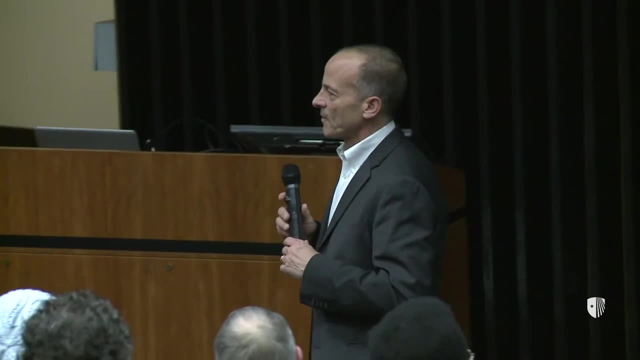 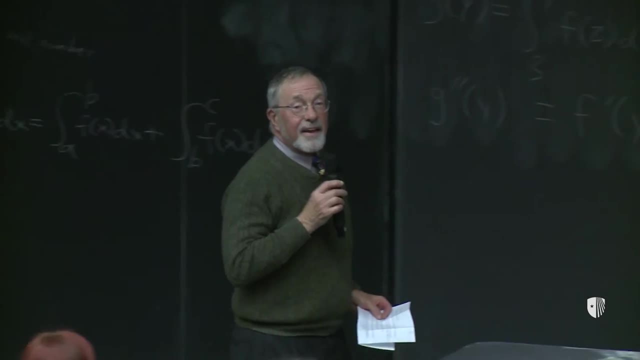 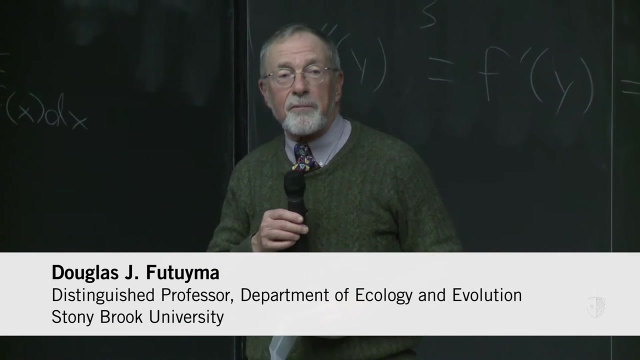 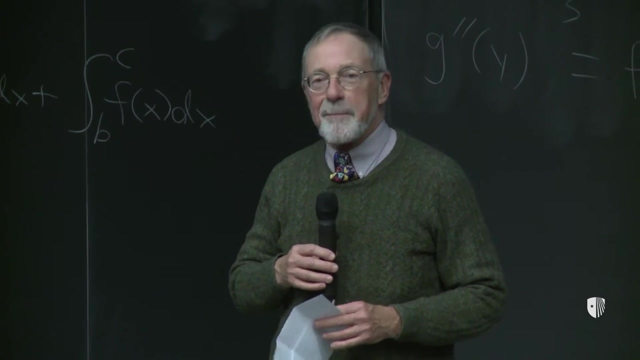 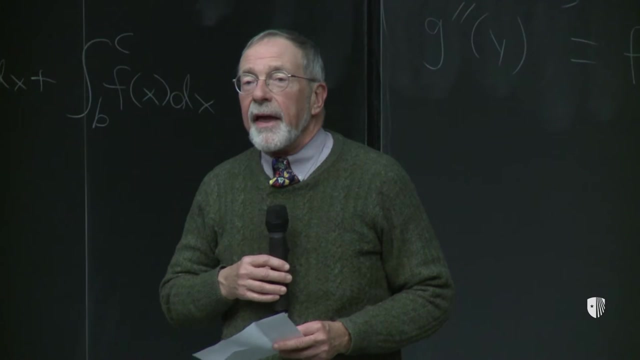 scientific denialism, And so it's my pleasure to introduce tonight's speaker. I'm Douglas Futuma. I'm a faculty member in the Department of Ecology and Evolution, and I was happily appointed as sort of the organizer of this year's Darwin Day. 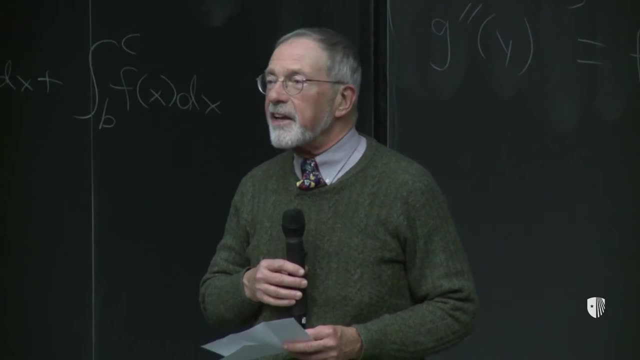 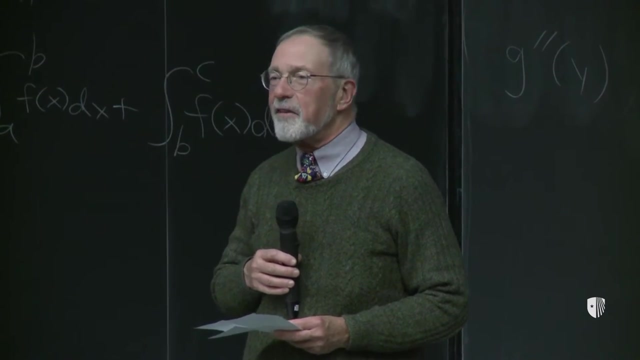 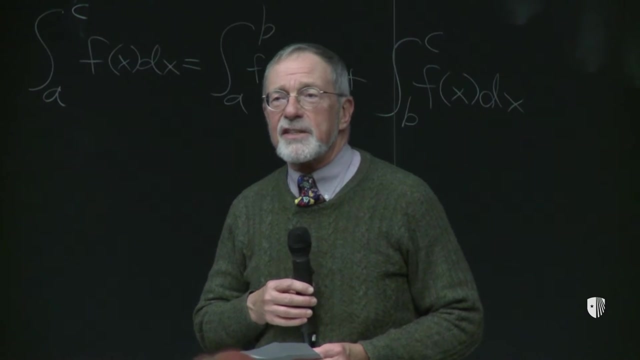 And And We. We have quite a variety of speakers for Darwin Day, but possibly none who paints as big a picture as tonight's speaker, David Jablonski. Many of us who study evolution are content to work with fruit flies, or perhaps to trace. 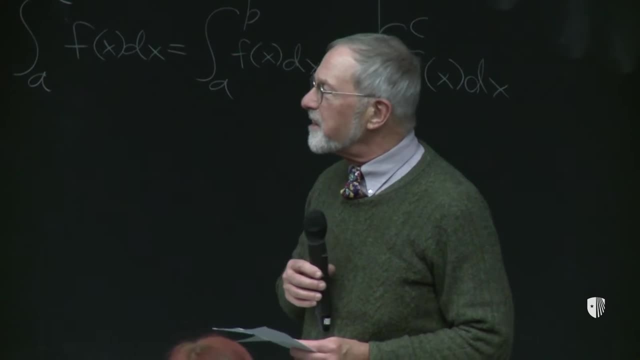 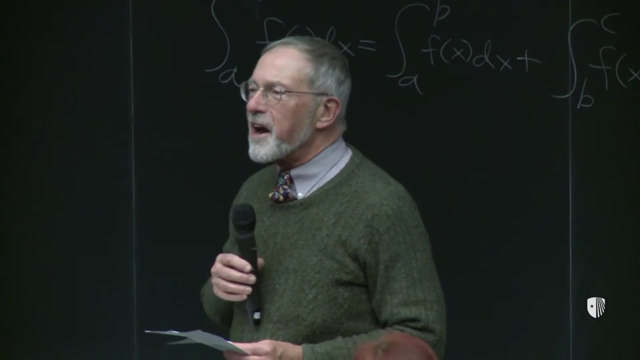 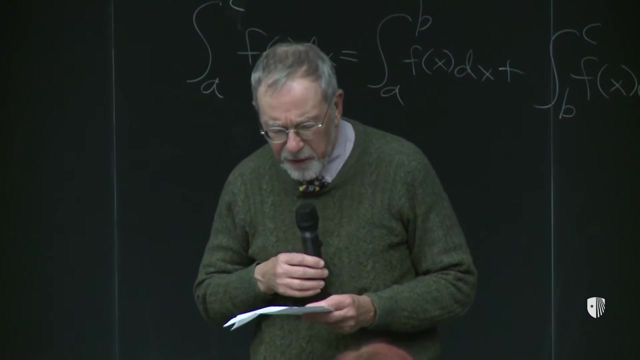 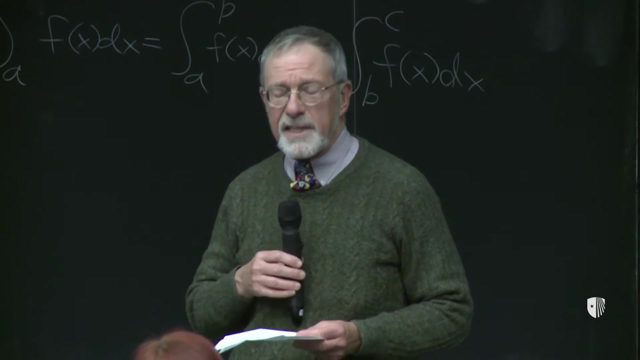 the evolution of microbes over the course of a decade or whatever, but David takes the last 540 million years as He's a person for the big picture indeed. Just a few words about him. His position is he is the William Canon distinguished professor in the Department of Geophysical. 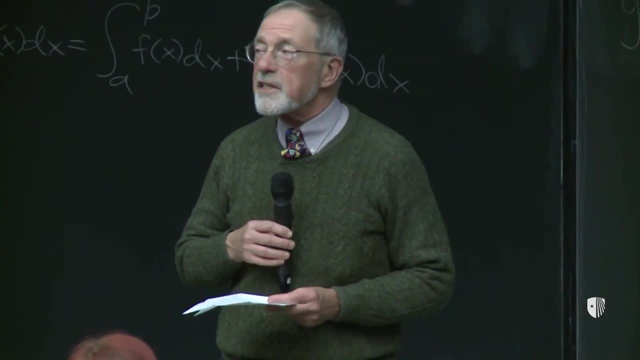 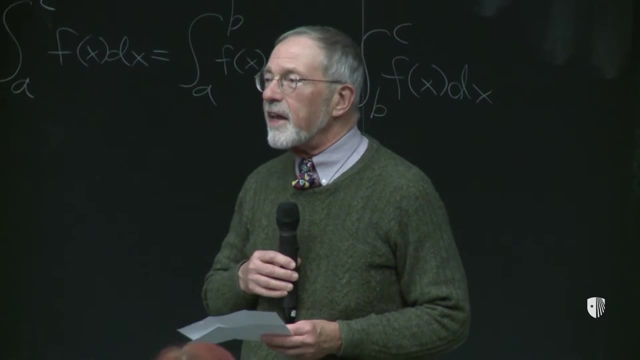 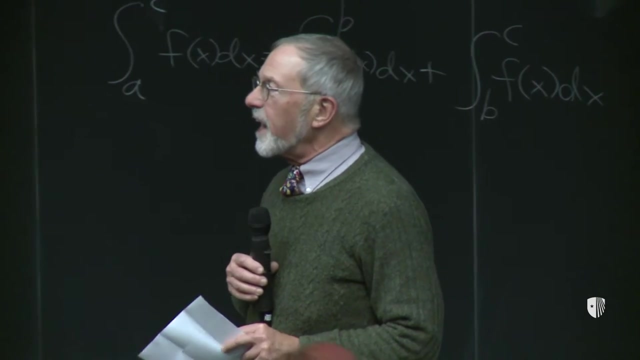 Sciences at the University of Chicago, And his personal history, very briefly, is that, like many of us, he grew up in New York City, where he apparently started at a very young age going to the American Museum of Natural History and looking at exhibits and becoming totally entranced with fossils and of 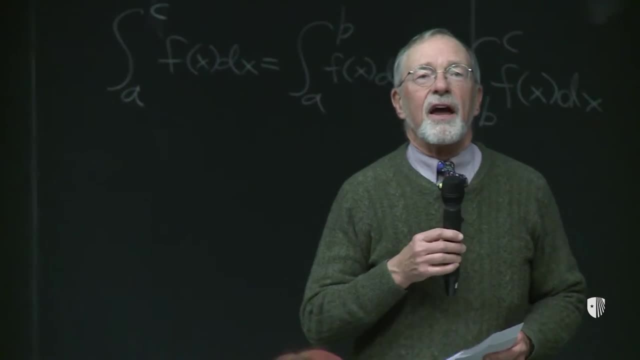 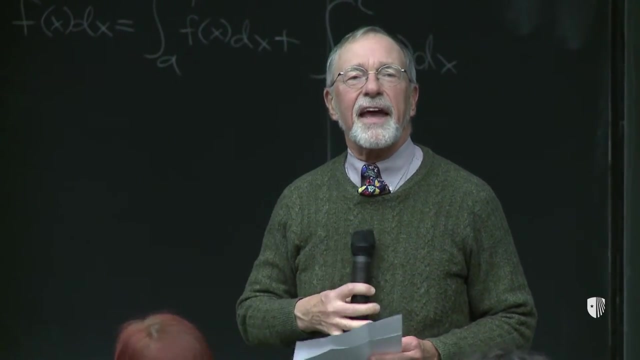 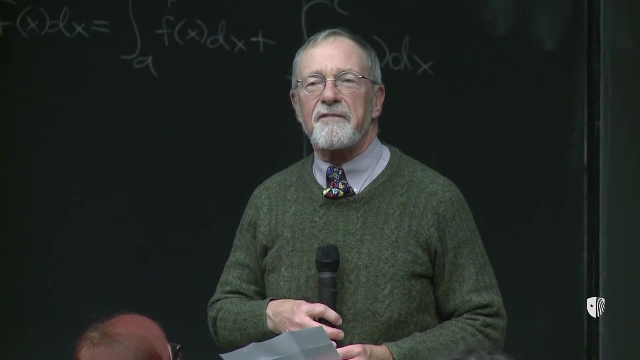 course he liked dinosaurs as a kid. well, unfortunately, this micro microphone isn't connected to the speakers, the loudspeakers, but thank you for telling me. so the point is that as, as you know, as a grammar school kid he got intrigued with fossils. this led him in high school, to actually become engaged with some of 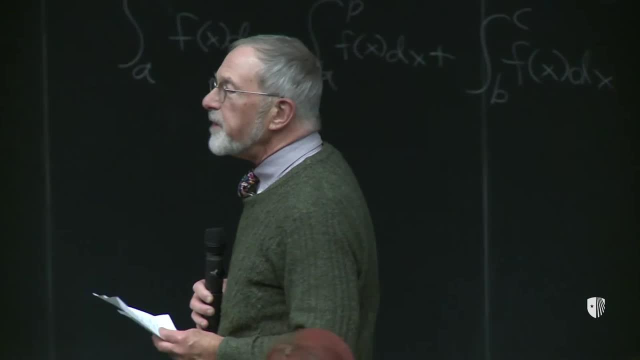 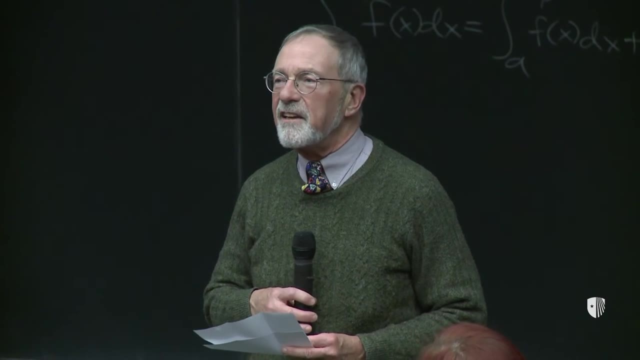 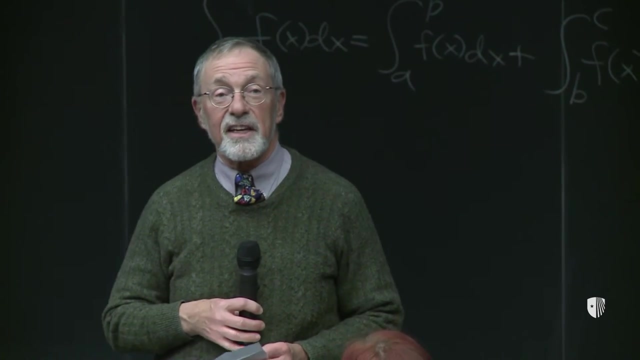 the researchers at the American Museum of Natural History. he then went to Columbia University, in part because there was a program of work-study- the urban core that was initiated by Lyndon Johnson- that enabled him to go to a, an Ivy League school. from there, he got his PhD at Yale and then, after some time, at 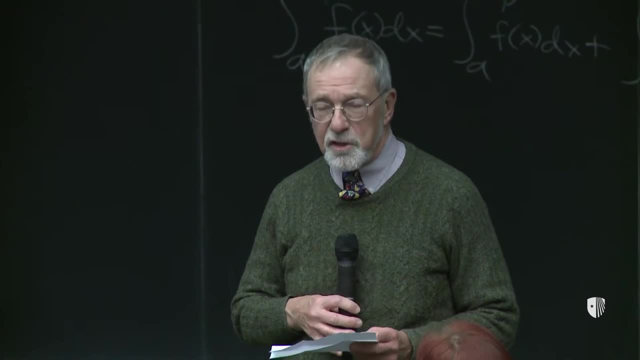 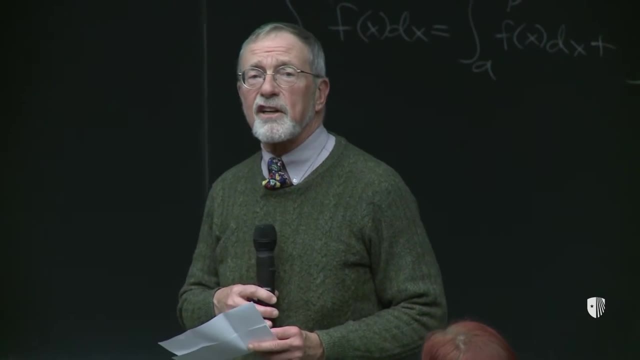 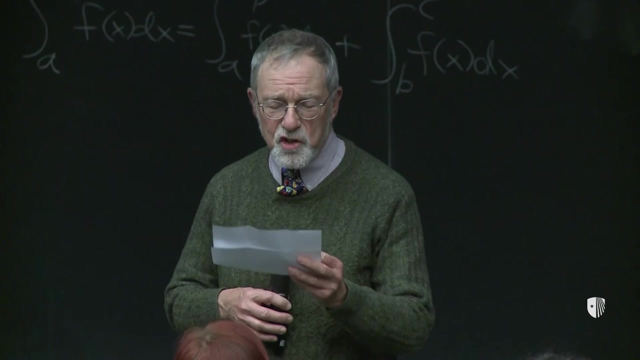 Berkeley and the University of Arizona, he went to the University of Chicago, where he is today. David has many awards and many honors, including election to the National Academy of Sciences, which is about as big an honor as you can get in science, short of Nobel Prizes and that sort of thing, and he has written about 150. 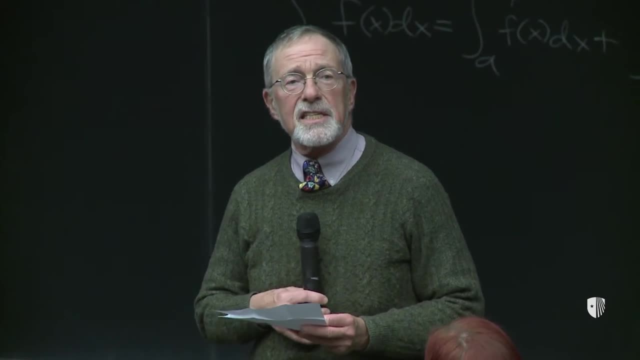 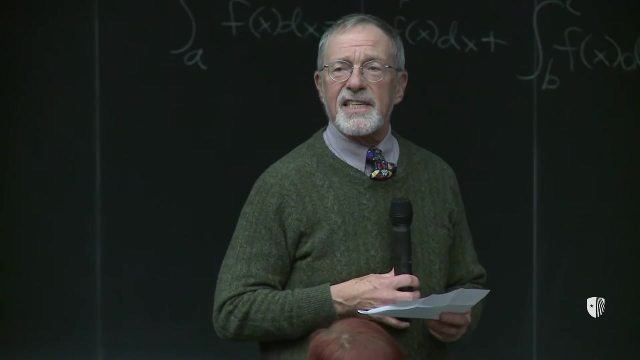 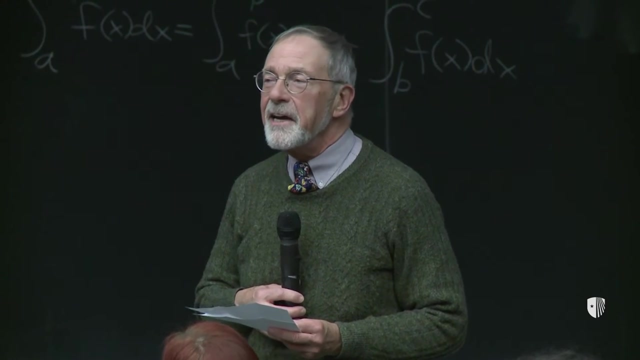 articles, scientific articles based on his knowledge, especially of a highly diverse group of organisms, namely bivalves, clams and oysters and scallops and things of that kind, and I suspect we will hear something about bivalves tonight. in the course of this work he has taken, handled and taken spec has. 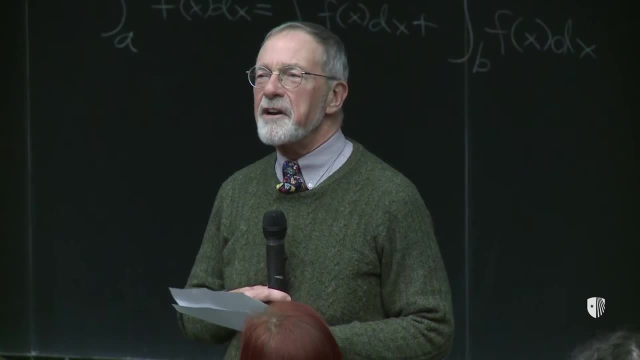 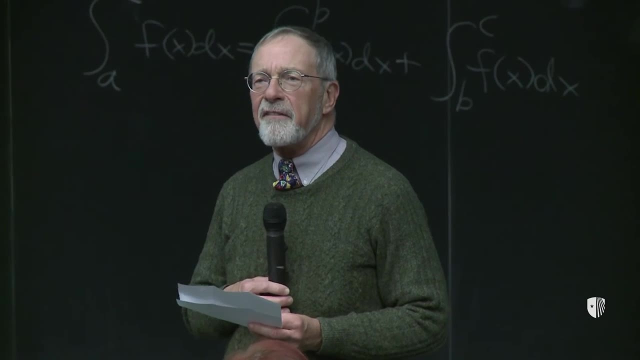 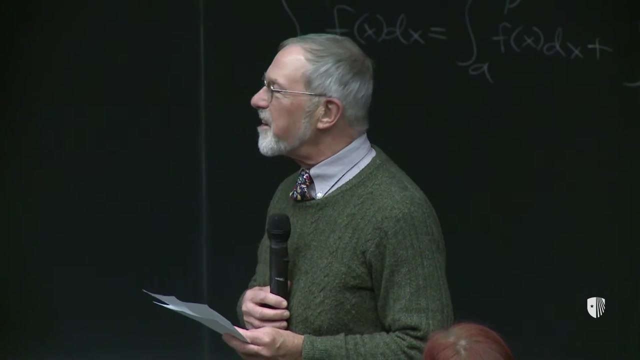 taken data on. he guesses about a hundred thousand specimens of fossil bivalves, and this is one of the things you can do with fossil bivalves. you can't do with with dinosaurs is you won't find a hundred thousand dinosaurs throughout the muse, the collections of the entire world, and you can't lay them out in. 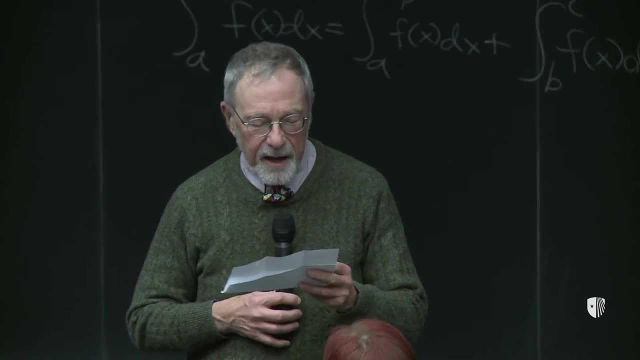 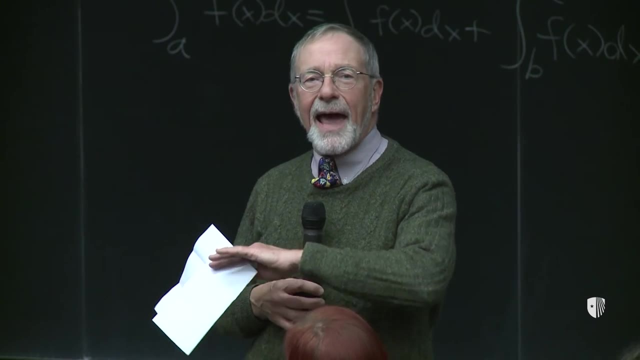 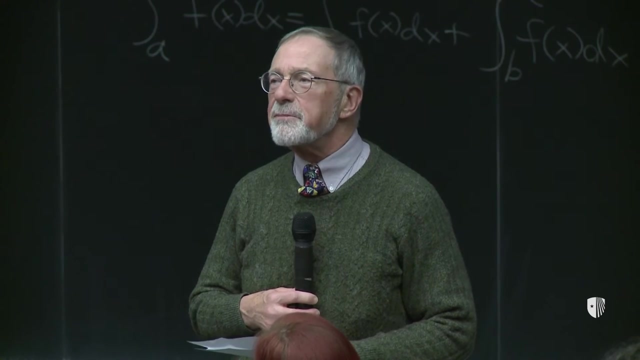 front of you and compare them to one another. so he is. he's published on many, many topics having to do with evolution and ecology as it has changed through evolutionary time, through geological time, and he is possibly the world's leading authority on the topic of mass extinctions, which is his topic tonight. 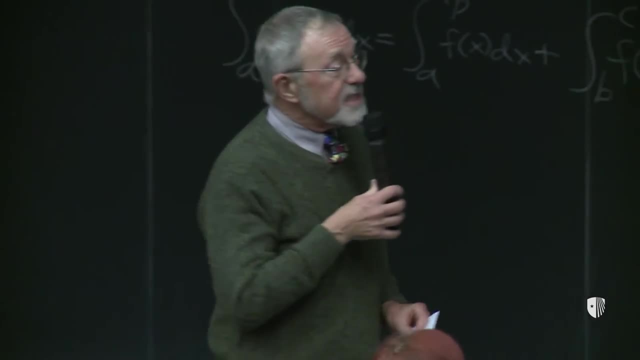 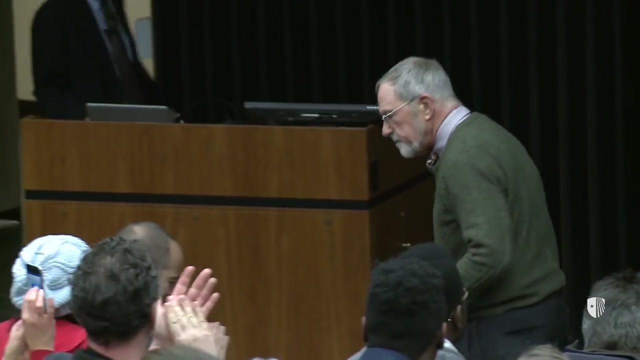 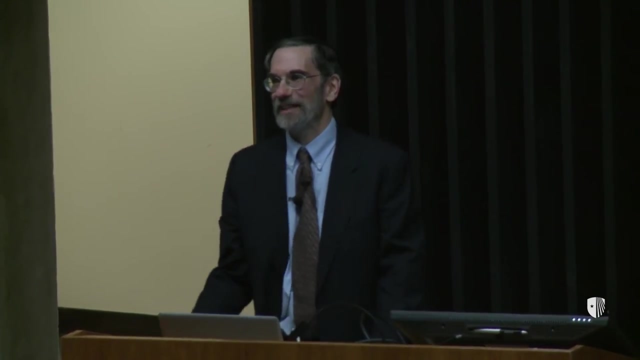 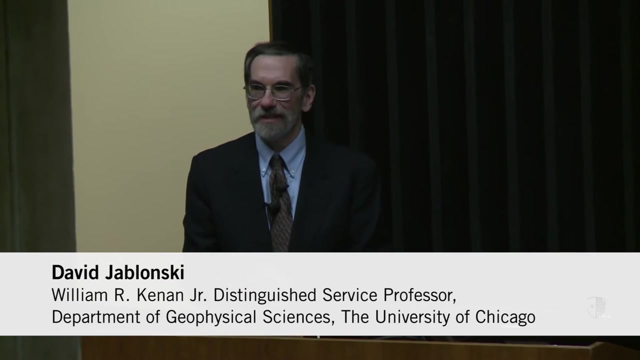 and so he is going to talk about mass extinctions and evolution, what we've learned since Darwin. David Jablonski, Thanks, Doug, and thanks everyone for braving the cold today to come to this talk. It's a real pleasure to be here to talk about Charles Darwin and his contributions and to 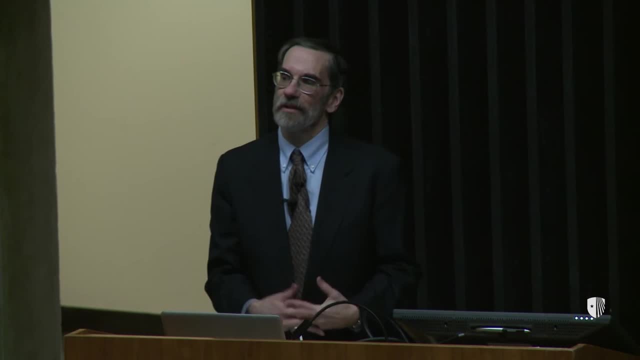 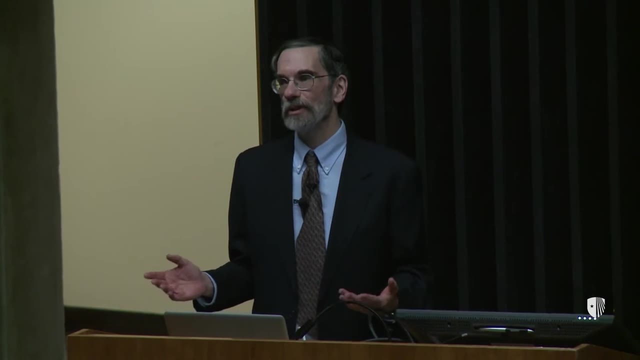 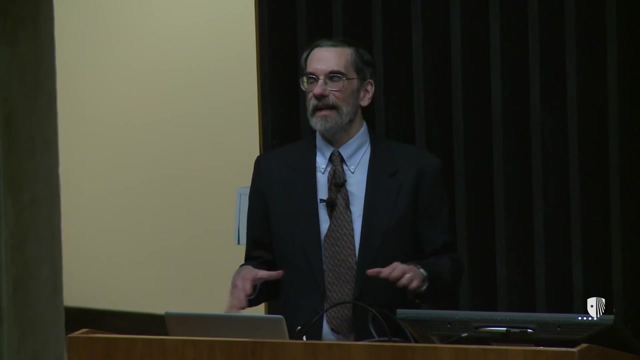 celebrate him on Darwin Day and to talk about Darwin's amazing and many contributions to understanding about how the biological world works, And also to talk about what we've learned since Darwin's time and how we can extend what Darwin laid down as a foundation into the 21st century. 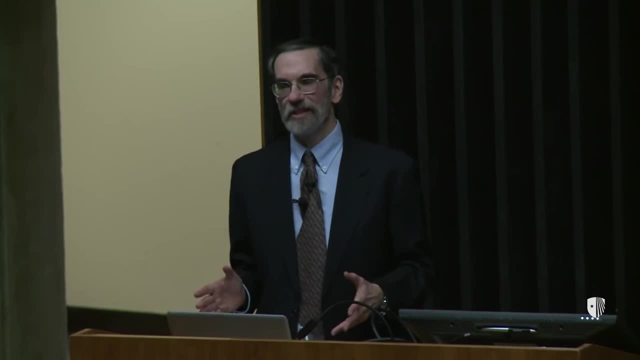 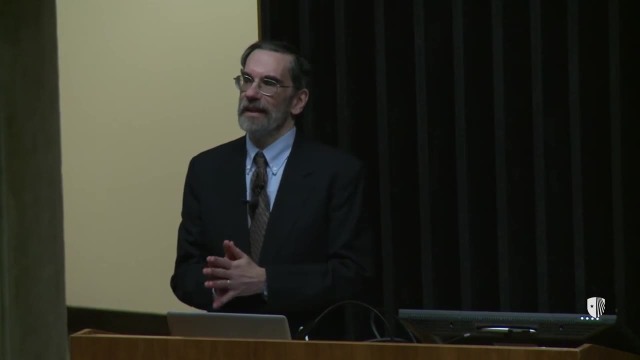 And that's what I want to talk about today, specifically about mass extinctions and what we've learned since Darwin. Now, Darwin knew about extinctions. He knew from looking at the fossil record that there were species that had existed on the planet that were gone. 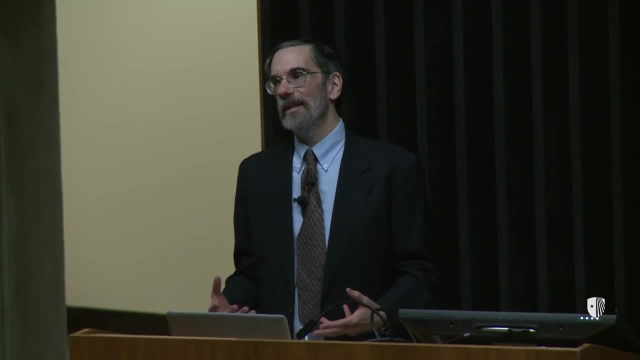 And what he wanted to think about was how that folded in to his larger picture. And what he wanted to think about was how that folded in to his larger picture, And what he wanted to think about was how that folded in to his larger picture. 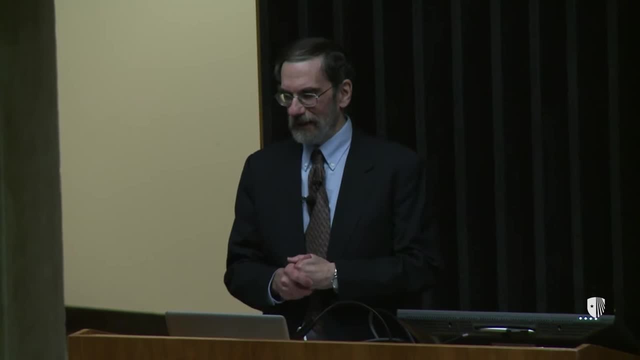 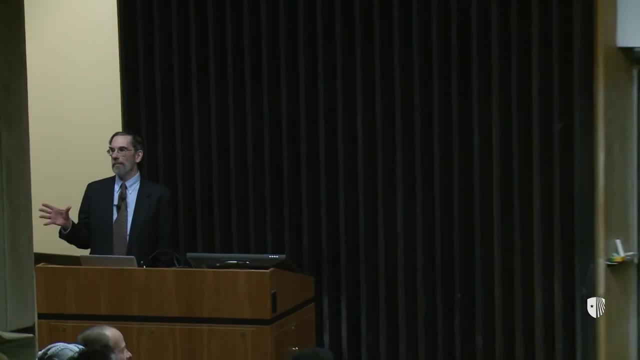 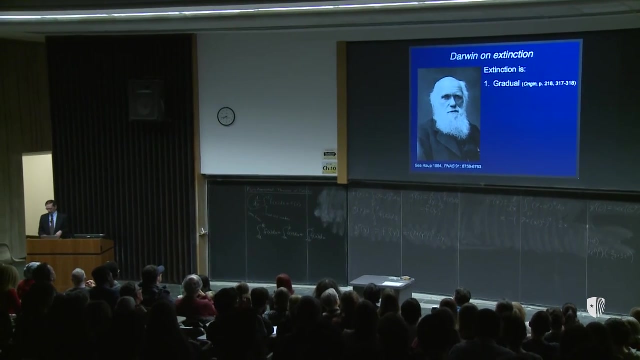 And his larger theory of life, And he made several points. He first argued, first of all, that extinction was gradual. It didn't happen abruptly. It tended to be a long dwindling of populations of species until they finally disappeared into oblivion. 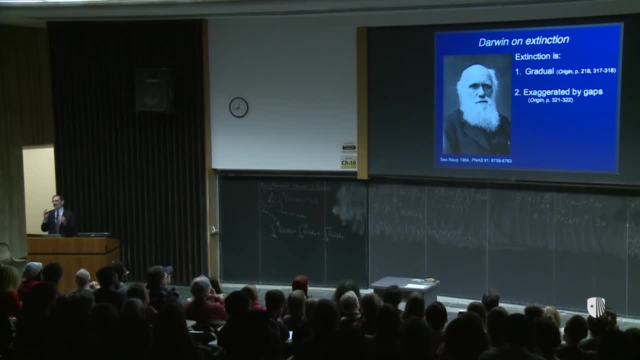 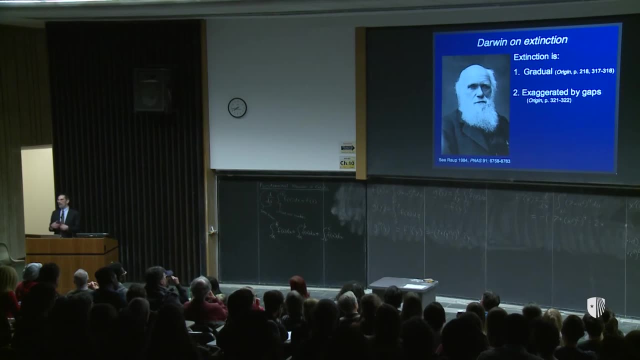 That the extinction we saw in the fossil record was exaggerated by gaps, That is to say, the fossil record he felt was full of discontinuities And, as a result of this, the apparent, The apparent extinctions that we saw in the geologic record were concentrated into narrow 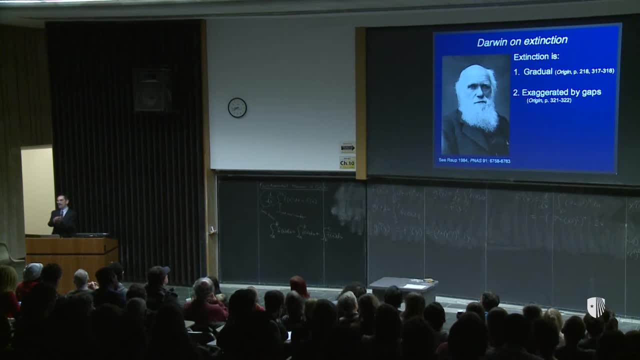 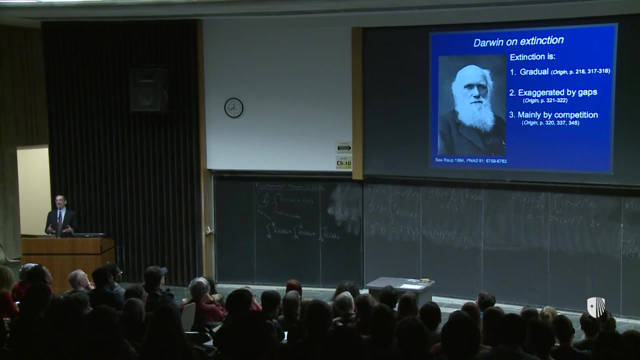 bits of geological time that were deceptive in their apparent abruptness and severity. He felt that extinction was mediated mainly by biological interactions, specifically competition, The competition for resources that could lead to the demise of individual species on a piecemeal basis. And, finally, he felt that competition, that extinction, was actually a vehicle for evolutionary 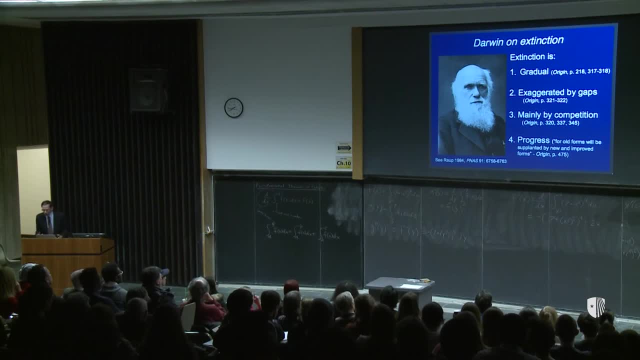 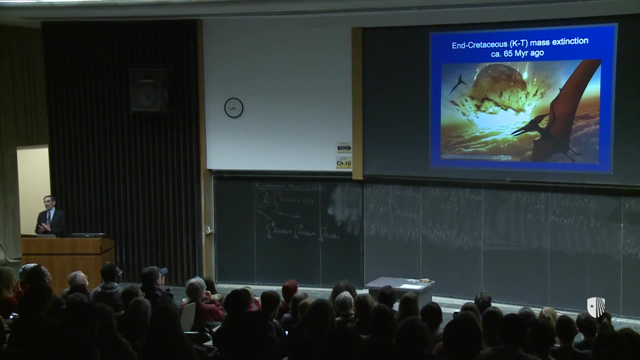 progress, That it was a vehicle by which old forms were supplanted by new and improved forms. So Darwin had a very specific view of how evolution worked. What he didn't know about were the big mass extinctions- The end-Cretaceous mass extinction, for example, which is going to be the main topic of my 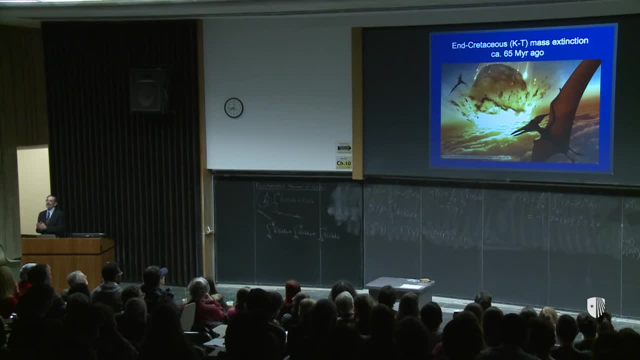 lecture today took place about 65 million years ago. It eliminated roughly 50% of the living species on Earth, both on land and in the oceans. as you can see here, It eliminated the large flying reptiles, the pterosaurs. 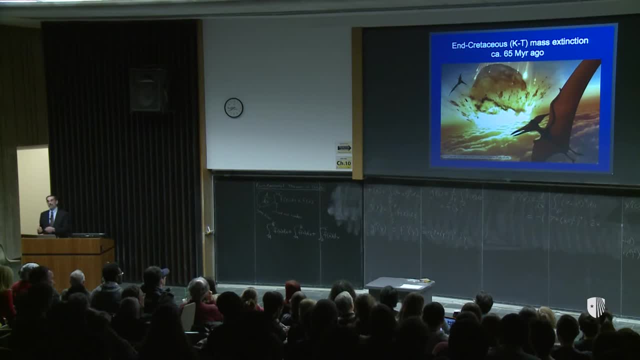 It eliminated the dinosaurs, aside from their living descendants, the birds, and a very wide array of different kinds of organisms in a geologically very brief period of time. And so the question is: what does this mean for the process of evolution? It turns out that there were multiple mass extinctions. 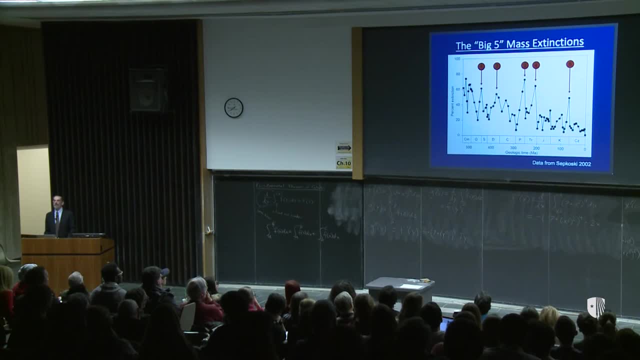 Not a lot, But The paleontologists affectionately call the big five mass extinctions. And what you see here is a geologic time scale from boy- the parallax here is spectacular- From over 500 million years ago to the present day, and this is the percent extinction in. 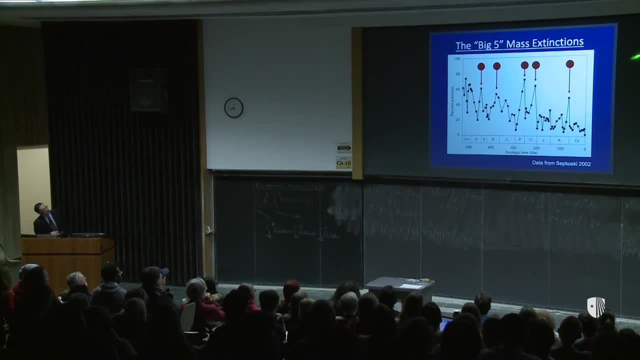 any one geological time bin. You see, on the top I've labeled in red the five big mass extinctions, with the last one right here being the end-Cretaceous mass extinction, a real spike in the intensity of extinction and then dying down to what we know today. 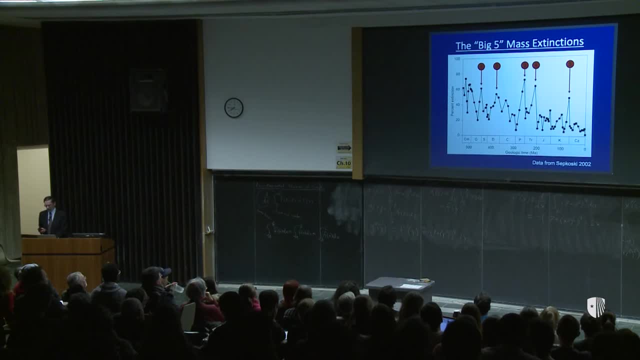 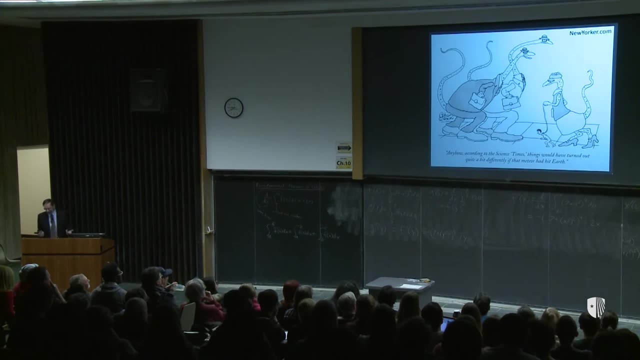 And then dying down to what we call background times of extinction. What did they mean? Well, here's one idea, As you can see here the cartoonist said. anyhow, according to the science times, things would have turned out quite a bit differently if that meteor had hit the Earth. 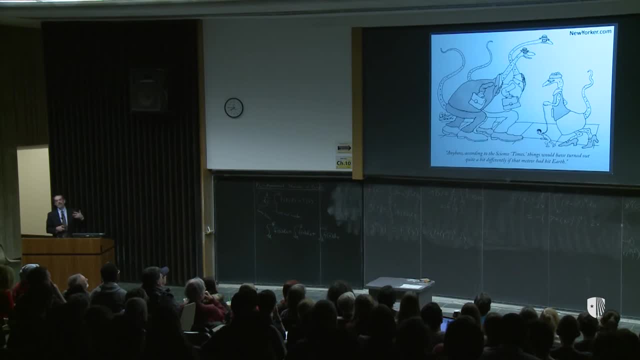 So that's one alternative history, And of course, there's multiple layers to this joke, Because, of course, what you see is, though, although the dinosaurs are now in charge and the human is on a leash down there, at the same time as you can see, what happened was. 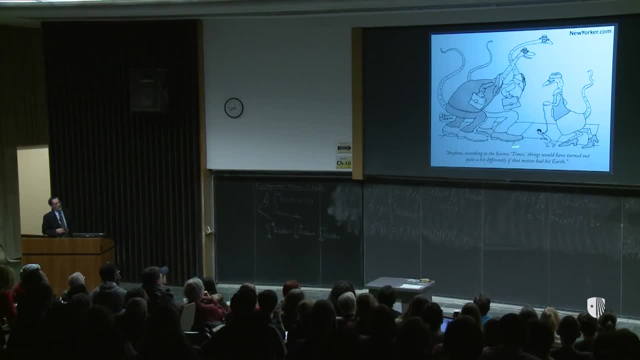 you ended up with shoes and briefcases and fedoras and of course naturally the New York Times. So that's a really funny cartoon. but how do you really address a claim like that scientifically? How do you approach this sort of counterfactual sort of playing of a game in a way that actually 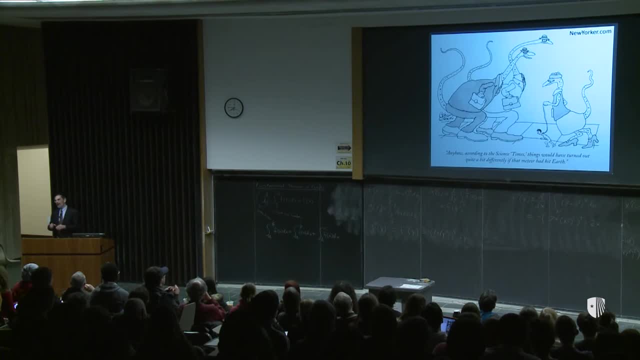 is analytical, And that's what I want to talk about. I'm not going to claim that I'm going to answer exactly what the world would be like if that meteor had missed the Earth. What I want to do is talk about how do these extinctions redirect the course of evolution. 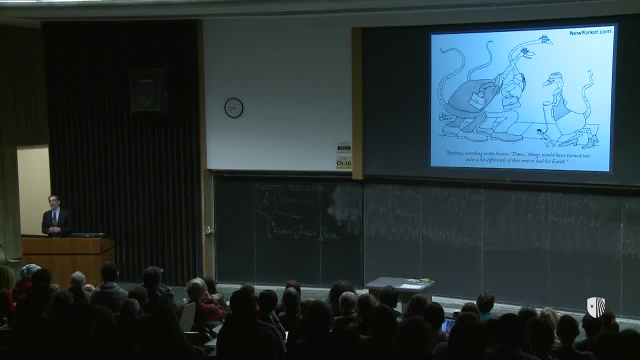 if they do Right. One possibility, of course, could be that extinctions, as Darwin thought it, the big mass extinctions, just a matter of turning up the extinction intensity dial for a little while and then turning back down again, Or maybe it's more than that. 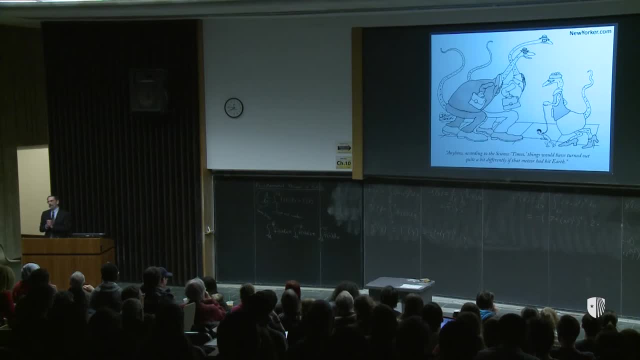 And that's what I want to talk about and explore that issue today. Now, as Doug sort of alluded to, you can't really do that with dinosaurs. In fact, this is the last one, This is the last picture of a dinosaur you're going to see in this talk. 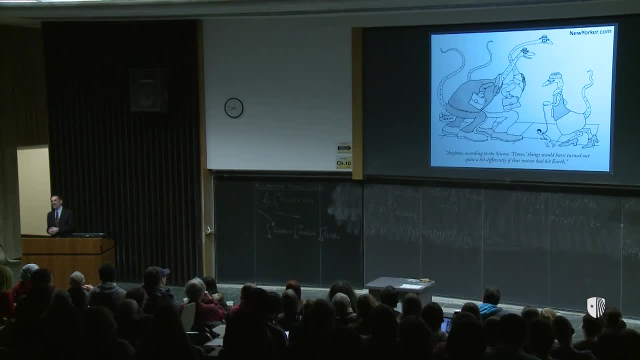 What you need to do is tackle those kinds of questions with a fossil record that is far richer than the fossil record of dinosaurs. Most dinosaur species are known only from the original locality from which that species was discovered, And that's not the kind of data that we need to understand how we got to where we are today. 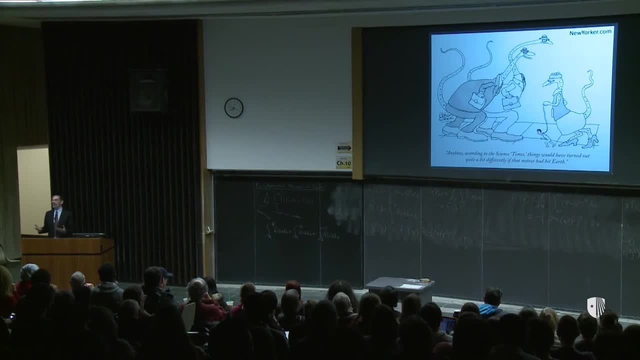 from 65 million years ago. If we want to understand how extinction is going to affect us, we need to understand how we got to where we are today from 65 million years ago. We need to understand how extinction took place, why it took place, why some groups 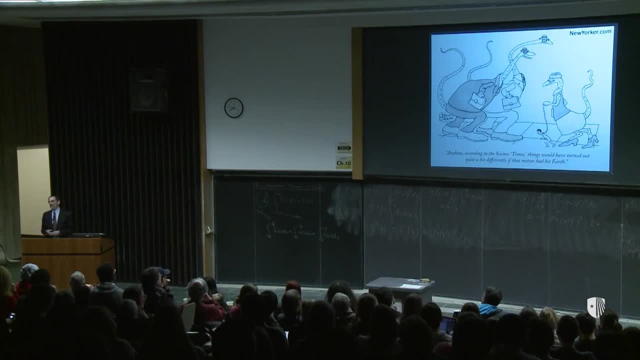 survived and why some didn't. What we need is a far richer fossil record, and that's where we turn to the marine invertebrates that have a very rich, very solid fossil record that will allow us to ask statistical questions. So what is even worse- and luckily the doors are closed so you can't get out all in a rush- 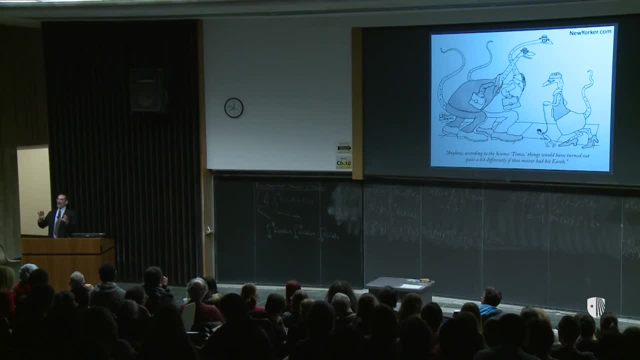 what that means is now, I'm not going to show you a lot of dinosaurs, but I'm actually going to show you a lot of graphs, Because it takes this kind of statistical thinking- Okay, Believe it or not- to answer the kind of question that's posed by that fantastic cartoon. 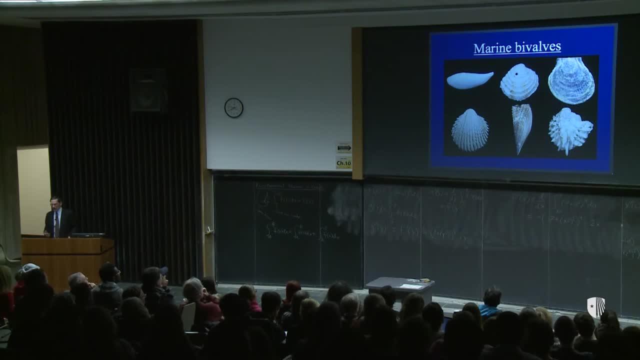 And what I'm going to do is I'm going to work with, as Doug said, marine bivalves. I'm going to look at, as you can see, here there are scallops and cockles and pen, shells and mussels and oysters and all the rest of it. 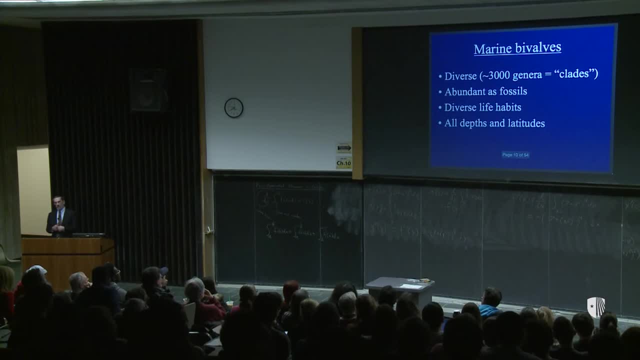 And why you ask marine bivalves, That's because they're actually the perfect evolutionary laboratory to study the big picture of extinction. unlike the dinosaurs, They're diverse. There's about 3,000 genera, that is to say, groups of species that are in the technical 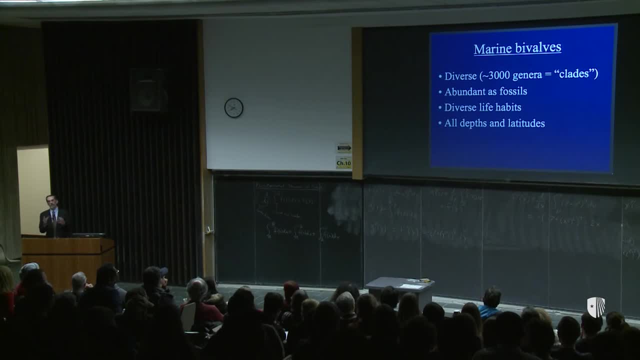 sense what are called clades- And I'll need to use that word later on, so I'm going to define it now. Clades are groups of closely related species that exclude all that include all the descendants of a single particular ancestor, And a genus is simply one of those little groups that is ecologically and in terms of. 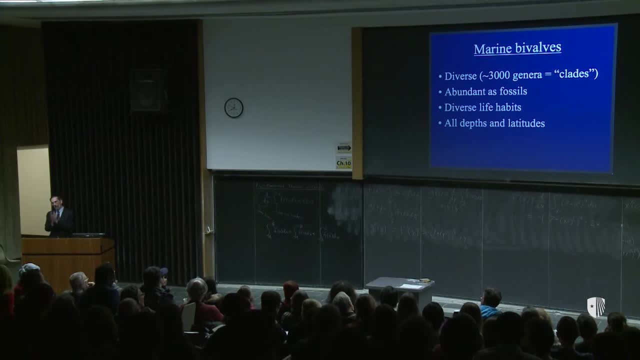 its biological form quite homogeneous. They're all. They all look approximately alike, with minor variations, and they're all doing about the same thing. They're a clump of closely related species. So I'm going to talk about clades. They're ridiculously abundant as fossils. 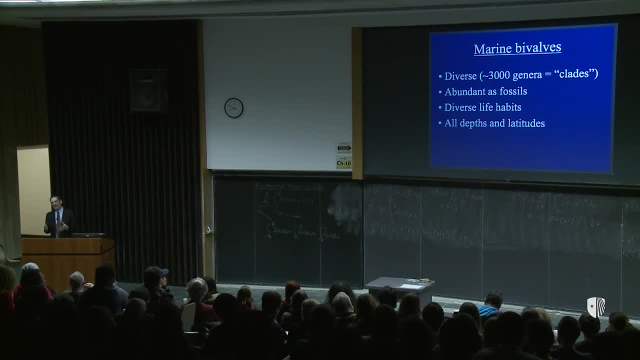 In fact, when I was doing my dissertation, they actually used the fossil oysters that I was trying to study as road metal, as armoring the roads in the back roads of Texas And, I've got to say, a trauma that I have yet to fully recover from. 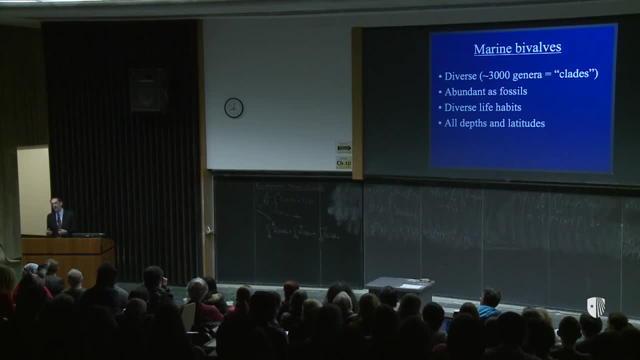 But they're really abundant and that means you can really ask questions about their form, about their species, Spatial distributions, about their abundances and so forth. It's a great system. They have very diverse life habits, So they attack, they cement to rocks, they bore into rocks, they burrow into the sediment. 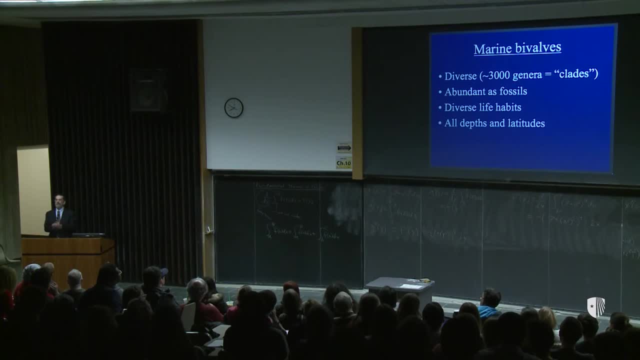 They have. actually they have photosymbiotic algae, some of them living in their tissues. They act like little corals. There are others that have chemosymbiotic bacteria living in their tissues, so they can actually live at great depth and exploit the chemicals that are in the sediments. 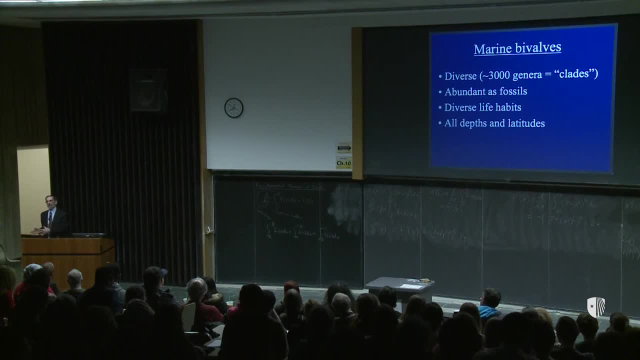 Some of them are herbivorous. Some of them are even carnivorous, So they can actually live at great depth and exploit the chemicals that are in the sediments. Some of them are herbivorous- An incredible range There are parasites. 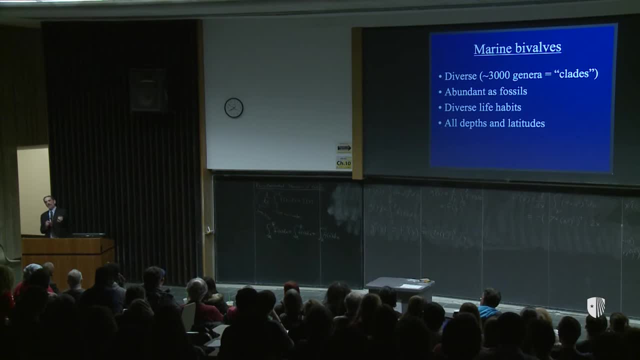 There's even a mosquito-like one that slides a little tube between the cell walls of other species of invertebrates. They're an amazingly diverse group And of course they live at all depths in the ocean, from the intertidal zone down to the 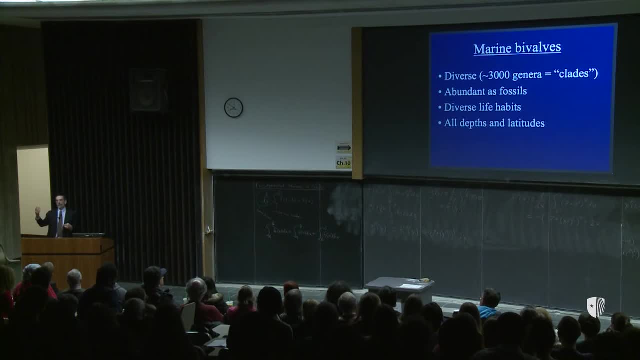 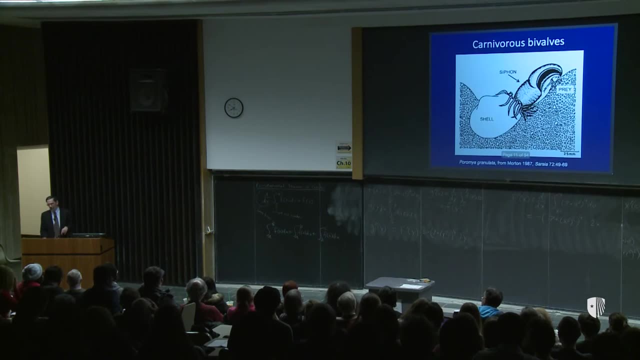 deepest deep sea trench, live at all latitudes, from the polar oceans right down to the tropics. They're a great system And, yes, I have to say really, they really are carnivorous. And here's a carnivorous bivalve. 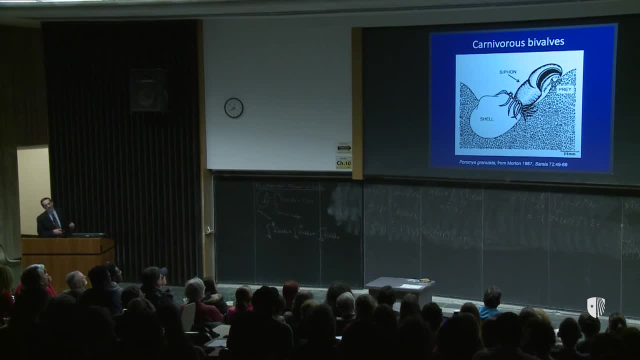 You can see here. There's the shell, There's the tentacles by which it detects its blithely approaching prey, There's an amazing modified fleshy tube called a siphon, And there is the hapless prey about to be engulfed. 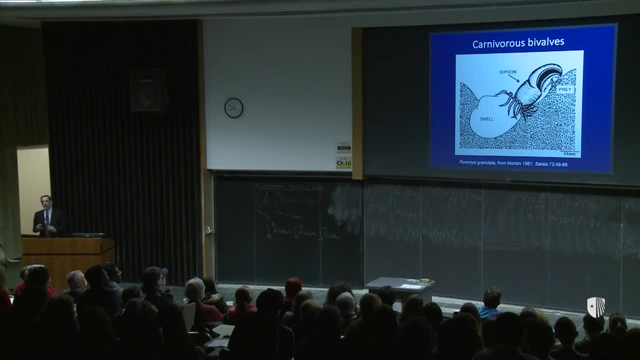 So they really are active predators. It's amazing. And before this puts you off ever going back into the ocean again, please notice the scale: 2.5 millimeters, So that's not so bad, But you have to admit that's pretty impressive. 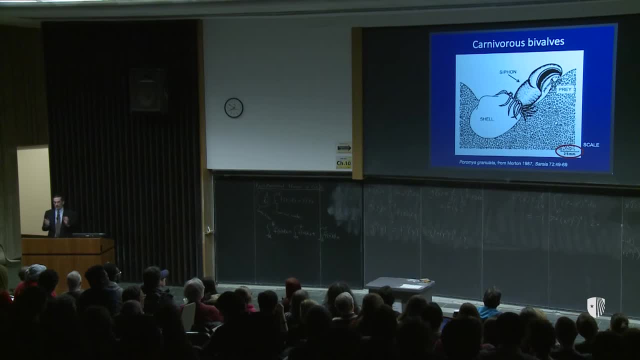 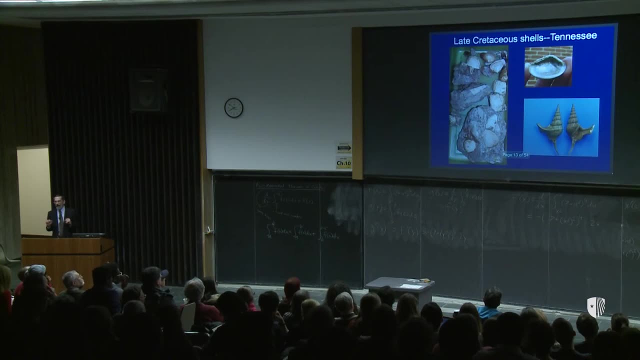 The size is really, really, really big for an animal that doesn't even have a head. That's really good. So they do a lot of different things for a living, And so what we can do is start looking at their fossil record. 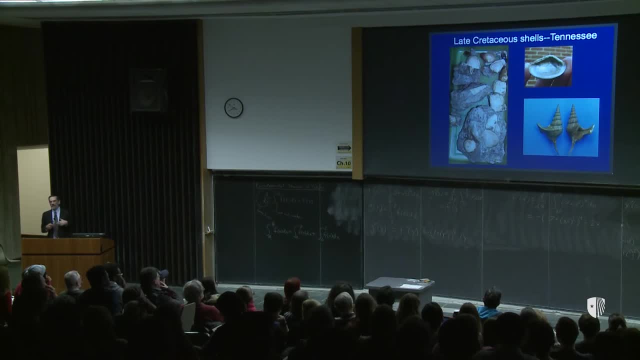 And what actually got me started in all this work was work in the late Cretaceous period, the 20 million years just before that big and Cretaceous mass extinction, where I collected fossils from New Jersey all the way down to Texas And you can see they're beautifully preserved. 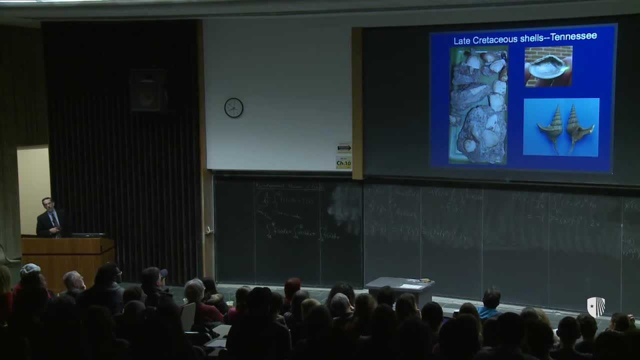 You might have picked them up on a beach. And here, for example, you can even see the original mother of a lion. the mother of a original mother of pearl is still lustrous in those fossils, Beautifully preserved snails and so forth. Indeed, the Tennessee state fossil came from my field area. You can see. 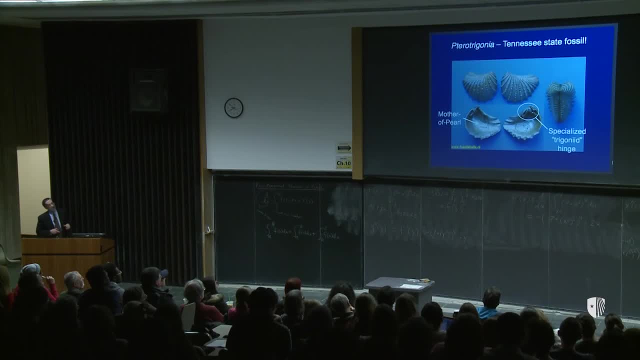 again the beautiful mother of pearl there- And this very complicated- which we'll get also further in our story later- this very complicated hinge structure where the two valves fit together, the two parts of the shell, the two shells fit together so the animal can open and close that shell in a very careful and precise way And that very 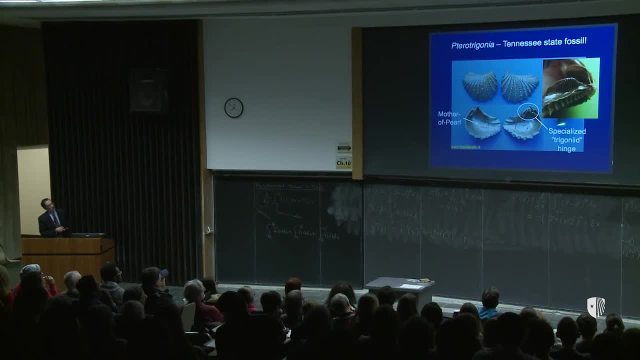 fancy hint is just in this particular group. the so-called trigonia is beautifully designed and very complex indeed, And the preservation is so good that you can not only see those grooves there, but with the scanning electron microscope you can even see there are grooves. 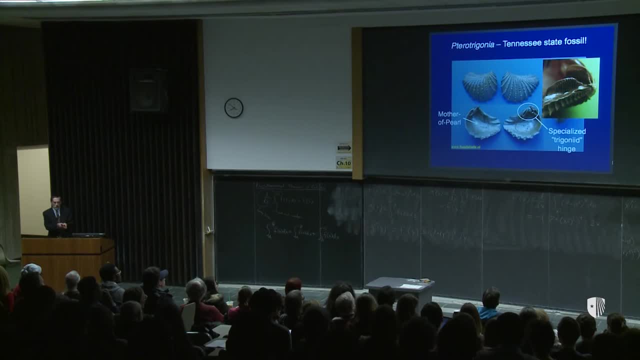 upon the grooves, upon the grooves, perfectly aligning that shell so it can open itself very wide, so they can burrow and then shut down tight if there are predators around. So preservation is exceptional. Subtitles by the Amaraorg community. There are also some very strange bivalves in the Cretaceous fossil record that are no. 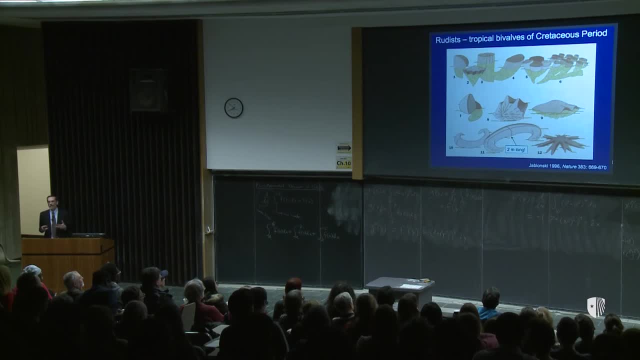 longer with us, A group called the rudis that lived in tropical waters that actually essentially evolved to become like corals. They were large. You can see this one here is two meters across. Many of them lived half buried in the sediment, as you can see there, Some of them lived just. 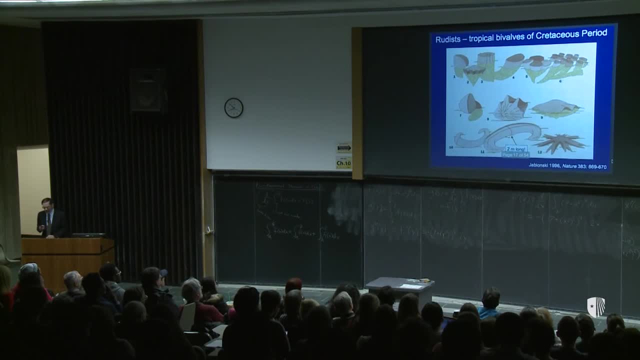 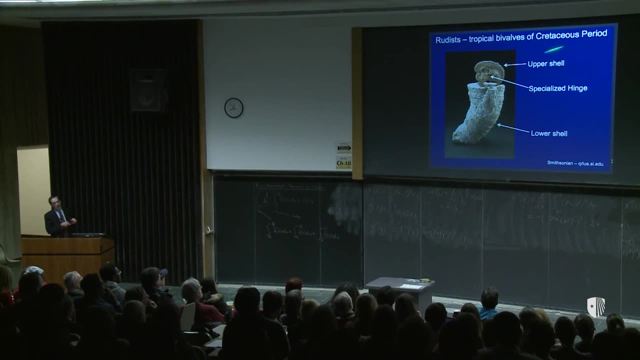 lying on top of the sediment And they and they again had a very complicated, novel sort of hinge structure that allowed- yes, one shell is down there And one is like the little lid on the ice cream cone that allowed them to build these. 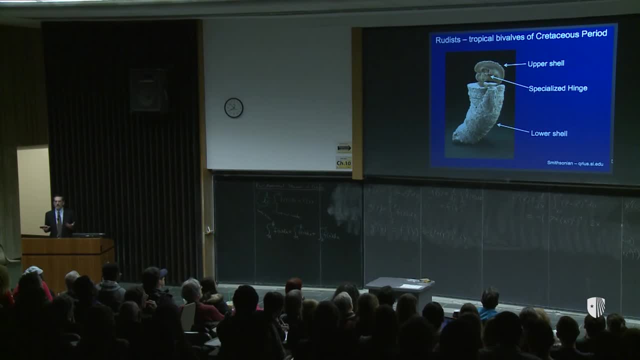 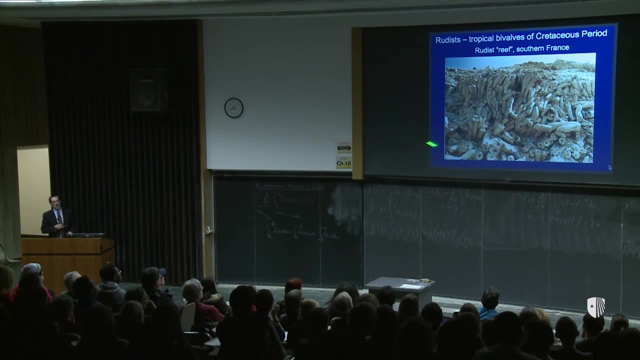 very complicated structures and inhabit what seems to have been the equivalent of a reef habitat in the Cretaceous period, And what you can see here is the very dense associations that they find, that you find throughout the tropical oceans of the Cretaceous period. 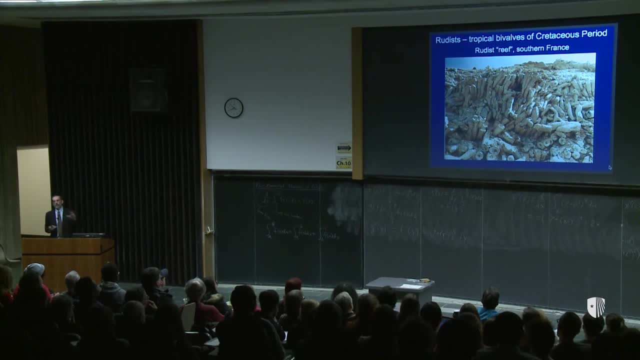 If you've ever been to the, you know on a boat in the Mediterranean and you've looked at the white and yellowish cliffs along the Mediterranean coast. that was these guys making their reefs 70 million years ago in vast, dense numbers. So the bivalves are a really 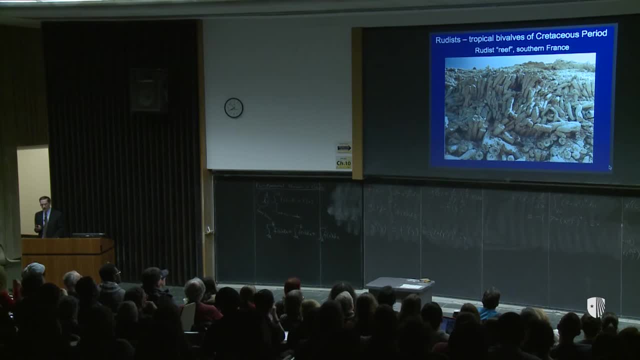 cool system to go after these kinds of big questions, And so what we can do using these bivalves is we can start asking questions about what extinction was like first, leading up to the Zan Cretaceous extinction, which, to be perfectly frank, was actually my dissertation. 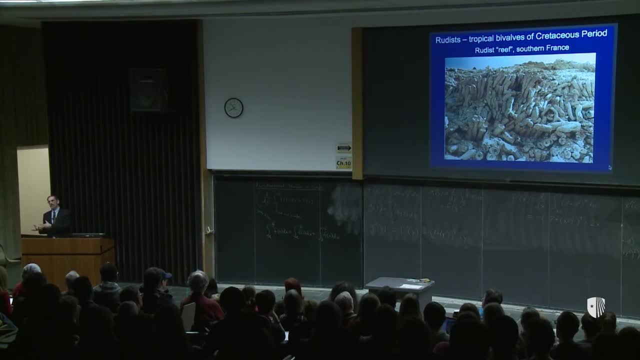 What was extinct, what governed rates of the origin of new species and the extinction of existing species? And so what we've done is we've looked at different species during so-called background times, during normal times, and then sort of this blinding flash of realization I realized. 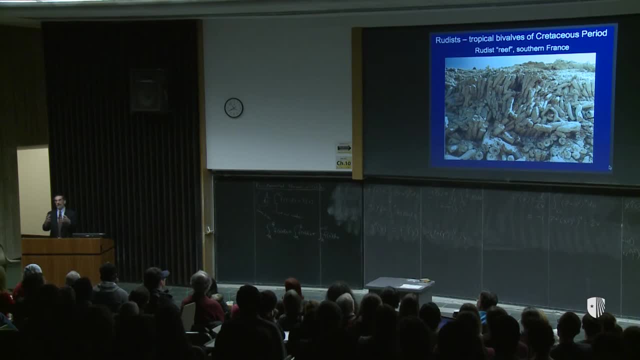 that, as the ideas were coming out about this asteroid impact, this meteor impact that might have driven the extinction, I realized I was perfectly positioned to compare what happened at that apparently razor edge of a geological moment in which the extinction took place to the 20 million years before it. 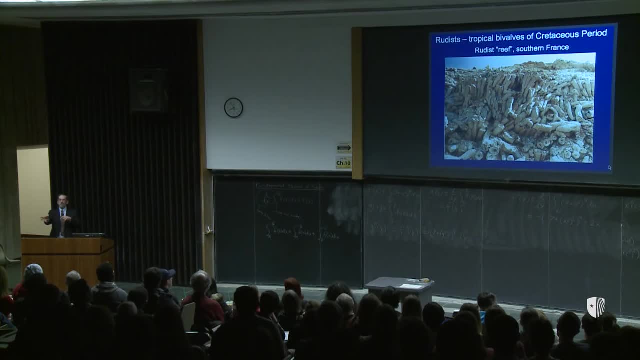 If it really was just turning up the extinction intensity dial or if something really special had happened. And so I was beautifully positioned for that, essentially by luck, by the fact that I started working in one system and realized I was ready to work in another one and ask a whole set. 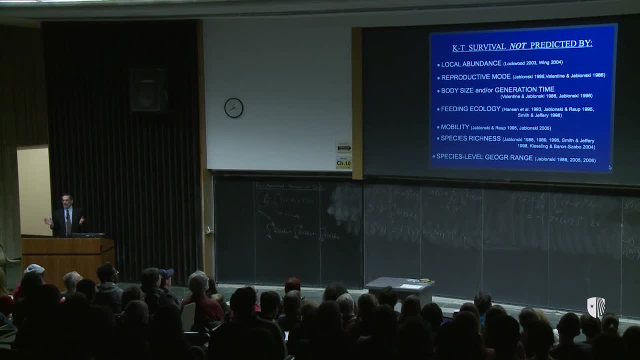 of new questions. And it was amazing because the survival across that encortatious mass extinction interval, what paleontologists call the KT extinction- was not predicted by any of the factors that I, or actually since me, my students and others- have found to have been important in the time. 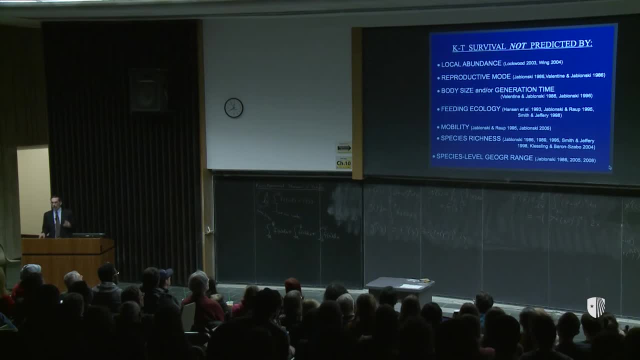 leading up to it and, for that matter, the time after it. But during this mass extinction time local abundance had no effect. Usually abundant things avoid extinction Modes of reproduction, the kinds of larvae they had no longer had an effect. Body size or generation time- important during normal times, not during the mass extinction. 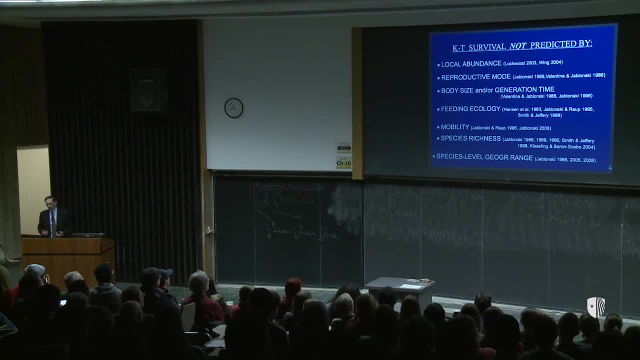 Feeding ecology the kinds of food they ate? no effect. Mobility: Whether they were cemented to hard bottoms or they could burrow around in the sediment- no effect Forever. evolutionary lineages: the number of species in the lineage really important. 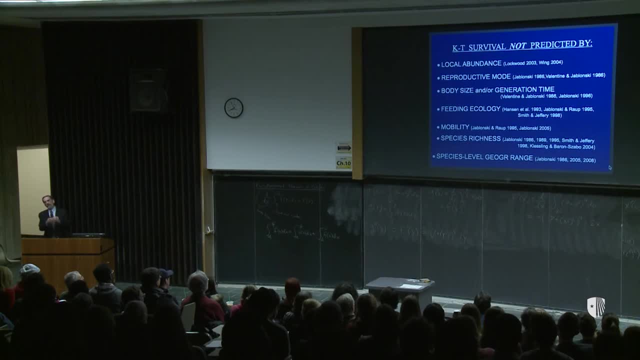 during normal times gone, And even the geographic ranges of the species within those clades right, the genera that are my analytical units- had no effect at all. It all went away. It came back a few million years later, but during that moment in time, that blink of. 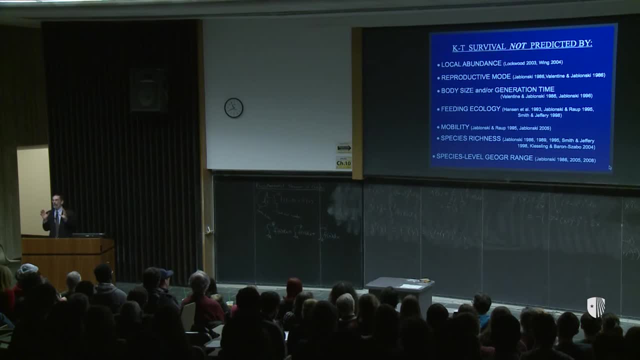 a geological, Of a geological, Of a geological lie. there was no measurable effect of any of those factors, And that was sort of stunning to me. That was kind of shocking. It wasn't turning up the extinction intensity dial, Something else was going on. 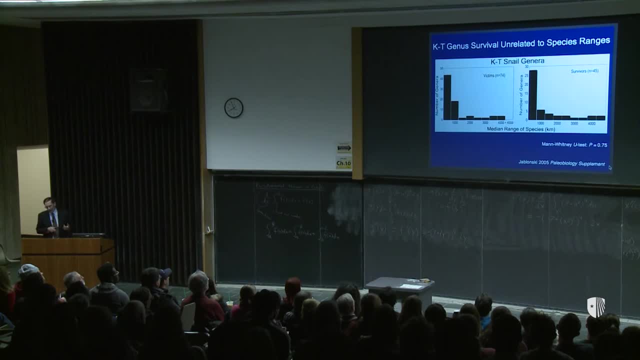 And just to show you that, with the unrelated to species ranges, what I simply did was I plotted the geographic ranges of the species within the victims and within the survivors of the mass extinction and there was no statistical differences between those distributions. There was no effective geographic range size. There was no effective geographical range. There was no exact size of the species. It was gone. A factor that had mattered for millions of years had been erased. Even the interactions among different kinds of traits fell apart. During normal times, the widespread lineages with lots of species did the best. 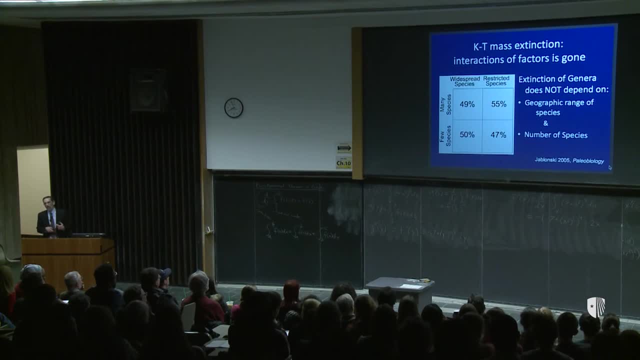 The ones that were narrowly restricted, with only a few species, did the worst, but then, when I went to this big mass extinction, those percentages are, statistically speaking, identical. So not only were the individual traits different, but they were also different. So not only were the individual traits different, but those percentages also were different. 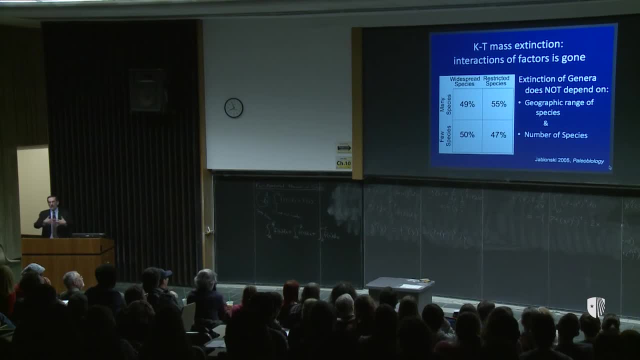 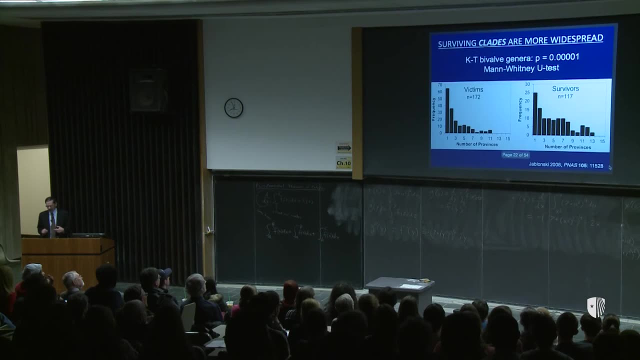 traits erased as having an effect, but in fact their interactions were gone too. There was no reinforcing effect of one or the other, So that went away too. But I did find a pattern. It wasn't sheerly random, which is what I was beginning to think. It turns out that 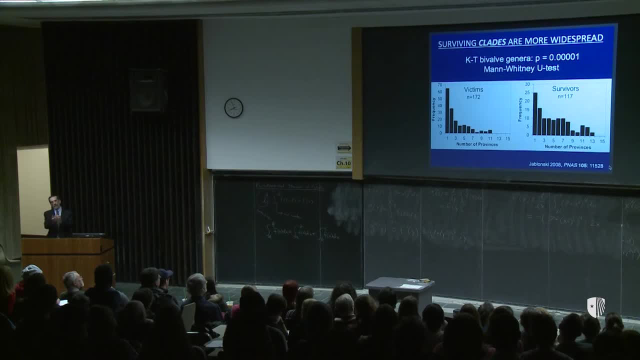 surviving clades are more widespread. The geographic ranges of the species within them didn't matter, but whether a clade was present in many what I call provinces here, that is, many distinct regions around the globe, that had a big effect. So the survivors shown 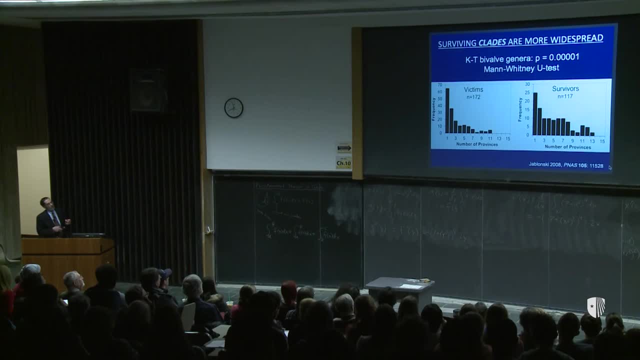 over here were, statistically speaking, much more widespread than the victims, which were much more localized. So you can see here out here they're a much fatter tail to this distribution, with the ones that occupied many more provinces, many geographic regions, Whoa. 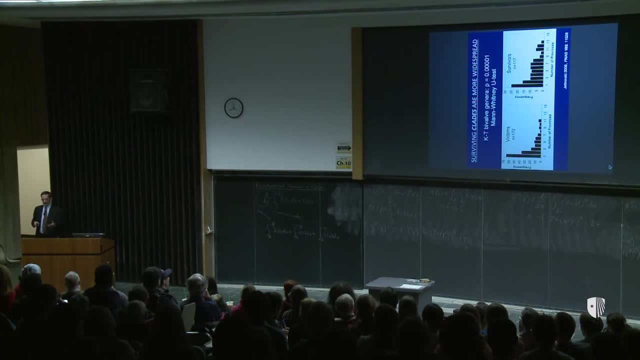 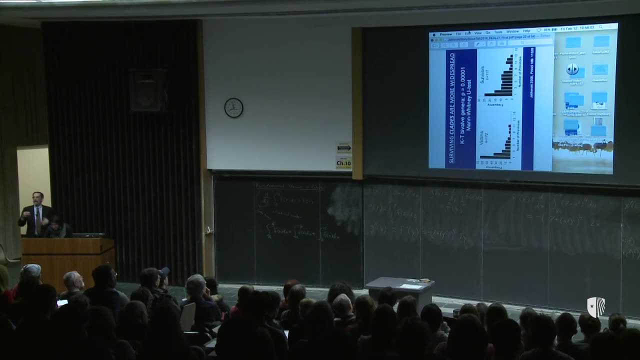 how did I do that and how do I get out of it? I'll let you fix that, And so what I want? in fact, I've revisited this question several times at different times in my research, going to a different set of museums, and we're almost there, going to. 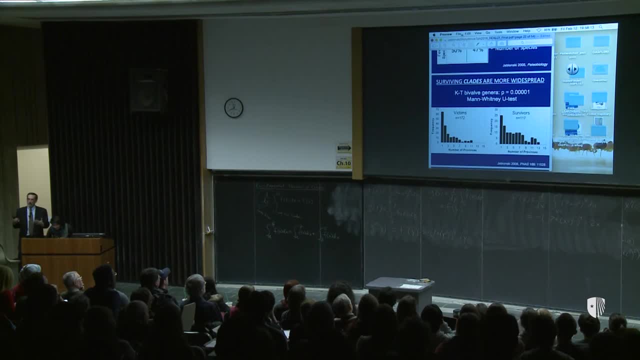 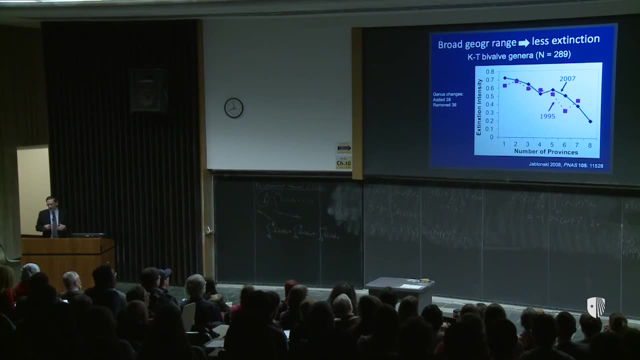 a different set of museums. So I actually, if you like, repeated the experiment. So the slide that's about to come up is going to show. thank you very much. is going to show. actually, two studies done 10 years apart. The first study, done in 1995, shows the relationship. 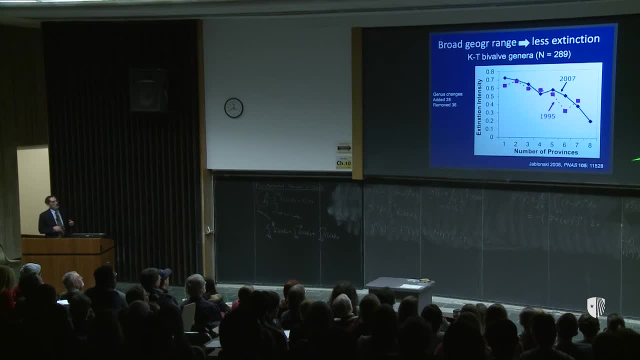 between the extinction intensity. The extinction intensity is the proportion that was lost versus the number of provinces. So which, as you can see, there is that lineages that were found, clades that were found in only one province had about 70 percent extinction, Lineages that were found in four or five provinces. 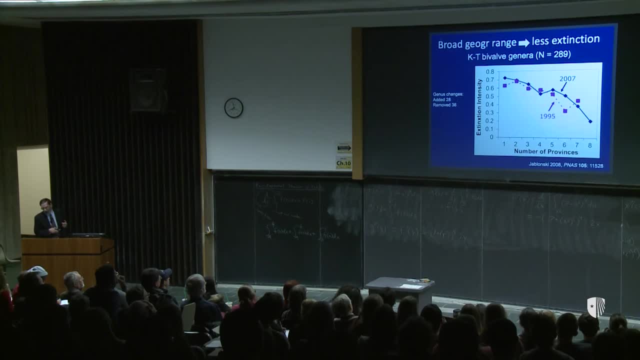 had about 50 percent extinction. Lineages that were found in eight provinces had only 20 percent extinction. 25 percent extinction. All my work in the natural history museums of Europe gave me a lot of great new data, but it didn't change that pattern whatsoever. 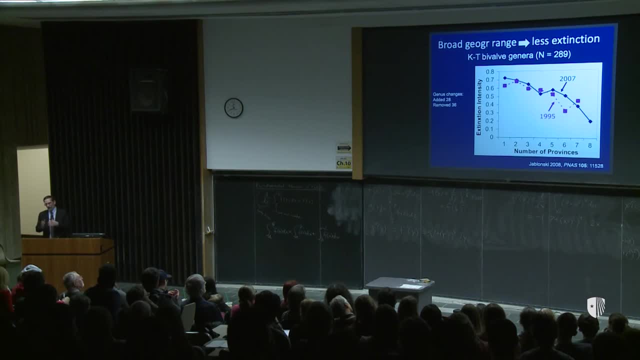 The widespread lineages had relatively low extinction. The geographically restricted lineages had had greater extinction. In fact, as you can see, the patterns got even stronger when I got more data. So it's 75 percent extinction, those very restricted lineages, versus 25. 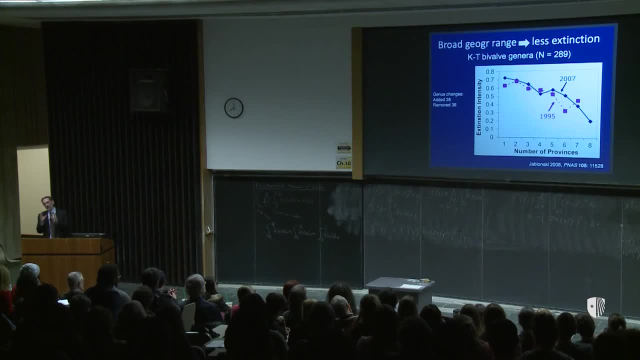 percent of the widespread, But I guess the one thing I want to say is the reason why I was able to do this is that the museums of the world contain an unbelievable wealth of information of biodiversity in the drawers that are tucked away behind me. 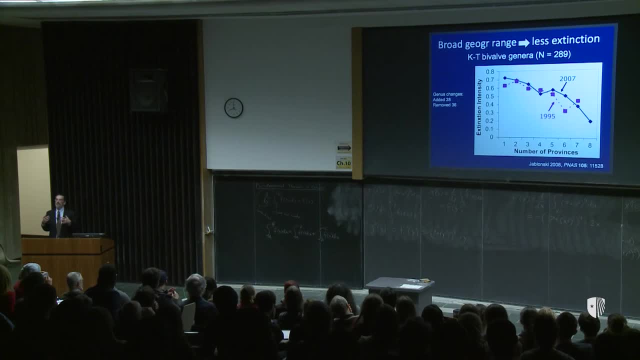 The museums of the world contain an unbelievable wealth of information of biodiversity in the drawers that are tucked away behind me. The museums of the world contain an unbelievable wealth of information of biodiversity in the drawers that are tucked away behind me. The kinds of research that you can do using those museums is mind boggling, And those museums 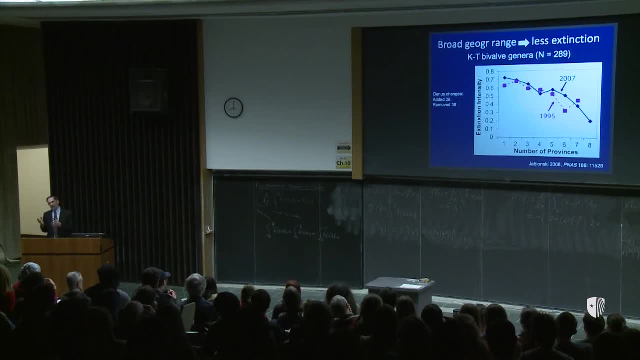 are wildly underexploited for this kind of research, And what I was able to do by going to these museums was I was actually able to improve the data significantly by comparing specimens among the many drawers, among the many collections from the many places that we had there. 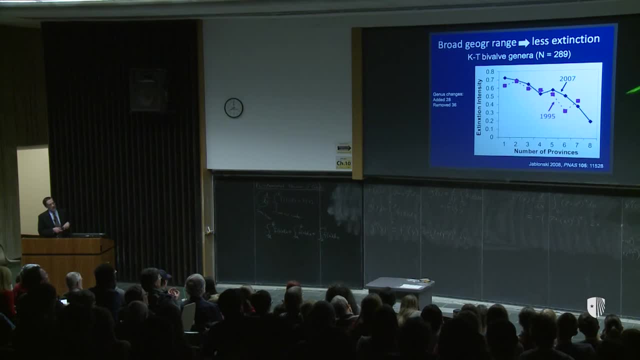 Now, just to make it clear. that's definitely lower extinction, no question about it. but 25 percent extinction of the most widespread lineage on Earth, that is still a serious business. Think about it as if you wiped out all the squirrels or all the sparrows. 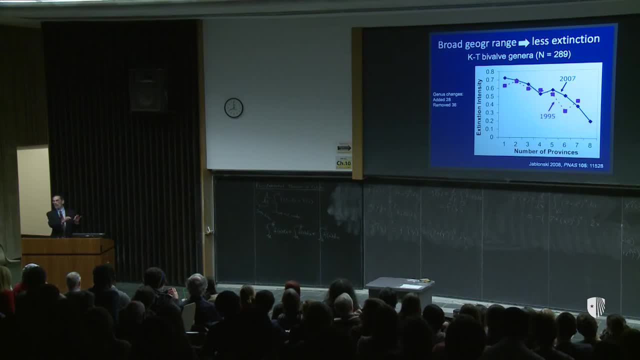 or all the pigeons in the world. It's not just wiping out the small localized guys, it's wiping out the really widespread ones, 25 percent of them gone. That's a major dent in biodiversity. And then, once you know to look for this pattern, it starts turning up. 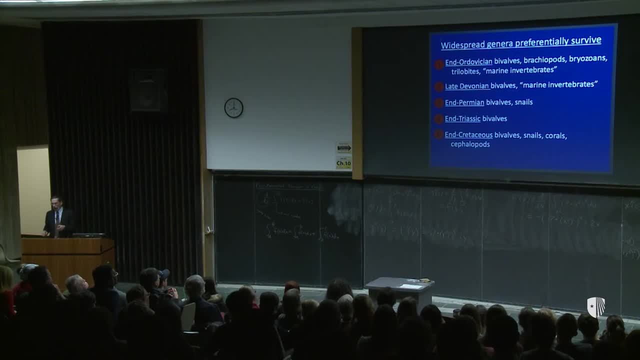 everywhere. And so here what I've done is I've simply listed all five of the big five mass extinctions in chronological order, and the names don't matter so much, but the point is that different groups- yes, the bivalves, but also other groups like other shellfish, like the bracket pods- 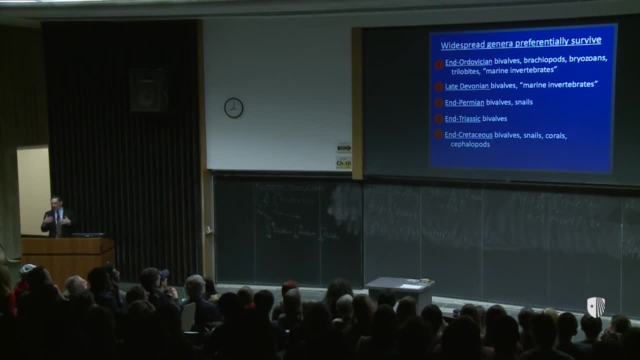 the trilobites, marine invertebrates in general, all show the same pattern that widespread genera preferentially survive. Every one of the extinctions- one, two, three, four and five- all show this pattern among different groups in different places. And that's what 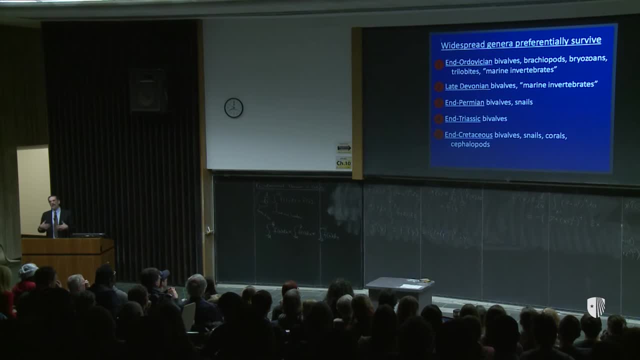 I've done. So. what happened to the ones that survived and which ones didn't? So we started to look at this from the diet of the geological core And we found that there were very few that survived much before the extinction of the first brown trout, who also only survived. about three times, three times, four times three times. but the second time they survived about four times three times, four times three times, and the third time they survived about one year. So that's a very interesting battle. And that's a great example of why genus ranges matter to mass extinctions, when species ranges do not necessarily translate into broad tolerances. I'd always figured that if a species was widespread, found over a very broad area, that it must be really tough and able to withstand all. 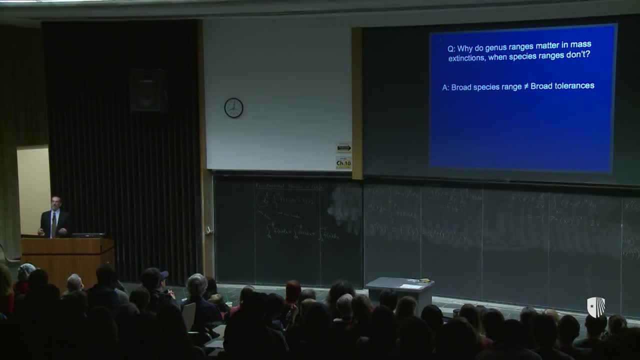 kinds of different temperatures or all kinds of- for marine organisms- different salinities, how salty the water is, or all kinds of different nutrient levels. But it turns out that's not necessarily true. It turns out that many widespread species are widespread because they're actually 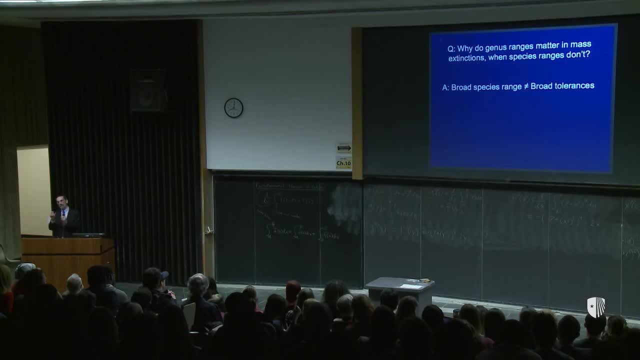 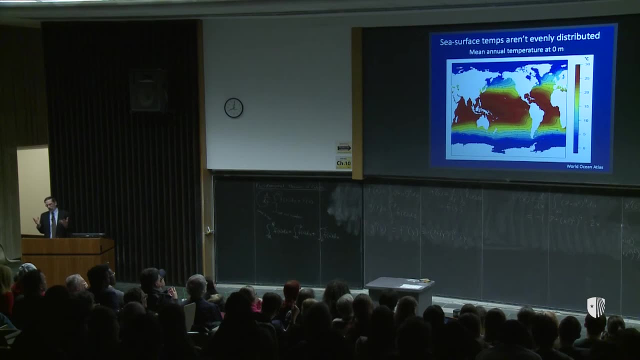 tracking widespread conditions Instead, say, a particular temperature. they're tracking over broad areas. So if you look at today's world and you look at the temperature distribution in today's world, one of the things that immediately jumps out at you is: there's this enormous 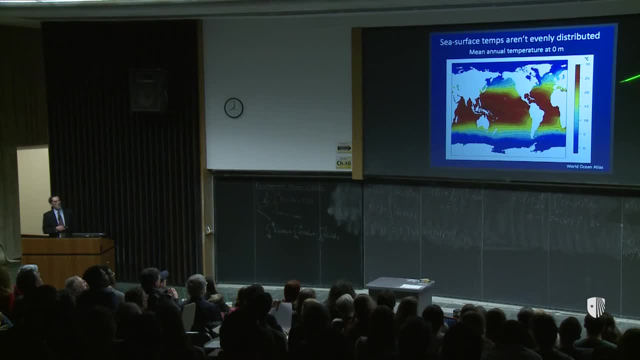 pool of warm water in the tropics And if a species is in that pool it could track over vast areas without ever leaving that very warm water. And that actually turns out to be really important Subtitles by the Amaraorg community. And the way we figured out that this actually was important for living organisms was we. 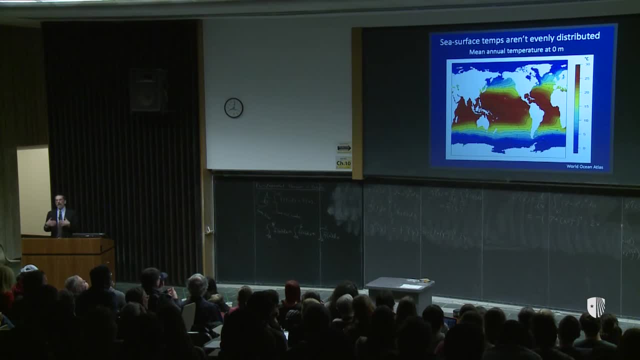 tested it using a sort of against a random pattern. What we did is we took the same geographic range sizes in the real species and then we used a computer to drop them at random on the surface of this globe. And then we asked for the ones that have been dropped. 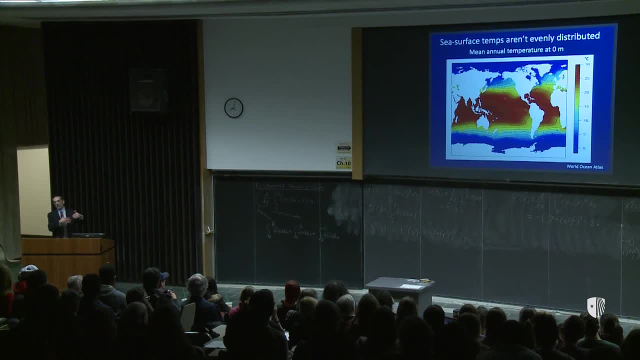 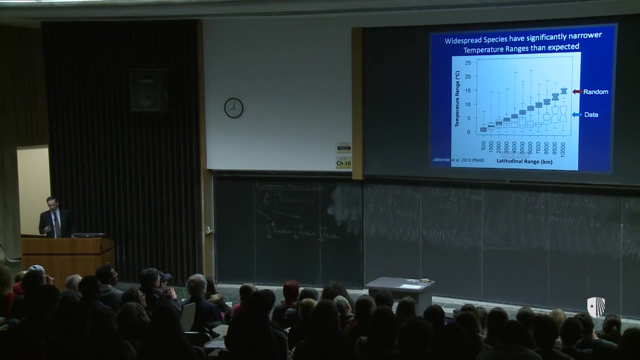 at random. what amount of temperature do those geographic ranges encompass? Because that told us what would happen if species simply were scattered across the globe without tracking special temperatures. And then we compared that to the real world And this is what we found. Here's the random pattern. What we do is- we did it 10,000 times to look. 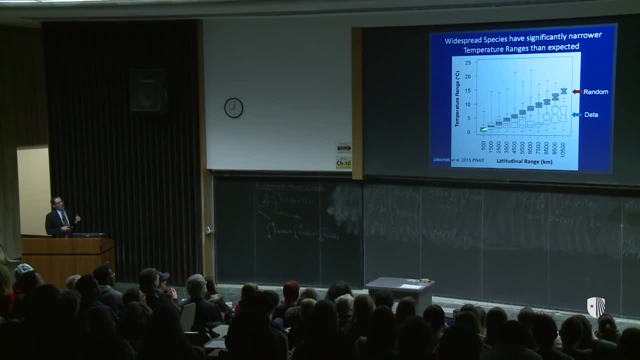 at it statistically And you can see the more you're geographically widespread, the more temperature shown against the vertical axis here compared to your geographic range. What blew me away was the more exactamente gesamal filter walls were turned off, that's. 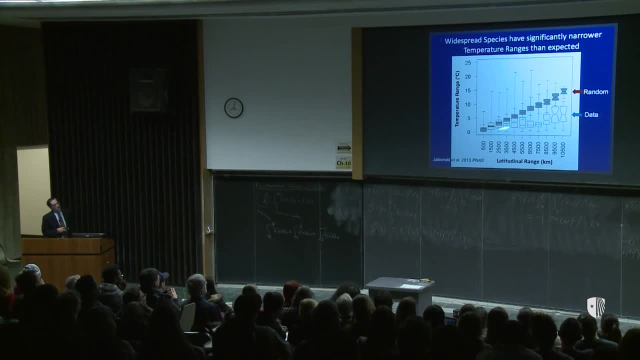 was the real data are much more restricted in the temperature ranges they encompass, even though they're very wide spread, So wide here. let me just show it more clearly here, For a random data, a species is found over 6,500 kilometers. encompasses about 8 degrees. 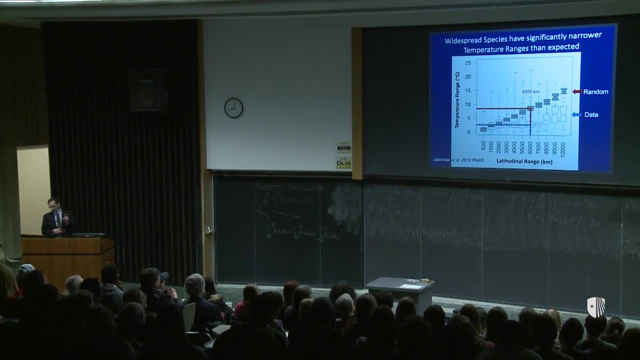 of temperature, But a real species that encompasses 6,500 kilometers only encompasses about two and a half degrees of temperature. They're much more restricted in their temperature tolerances than you would expect given the enormous breadth of their geographic ranges. And that's really interesting Under normal circumstances, those broad geographic ranges. 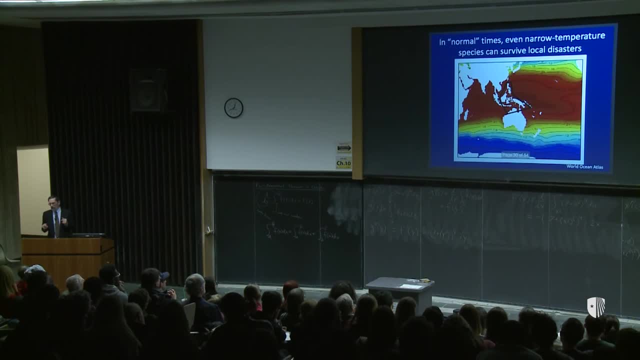 even if they're not tolerating a lot of temperature, will still, in fact, encompass an awful lot of territory. So here's a species that's found from the Philippines to the west coast of Australia. Dr David Shulman, PhD, Out across the world. 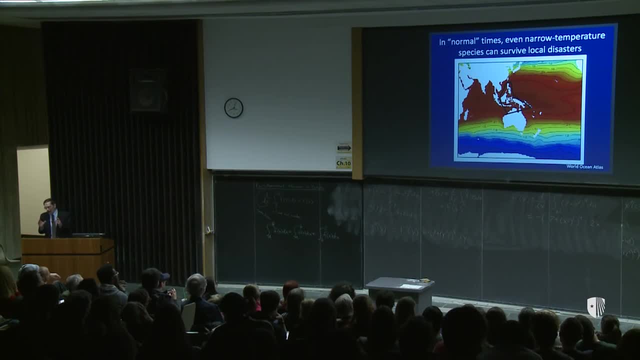 Dr David Shulman, PhD, Across New Guinea to the Marianas Islands Very broad, without ever leaving that 27 degree C temperature envelope, So that if a typhoon comes through and clobbers the reefs on the northern end of the Philippines, that species still has. 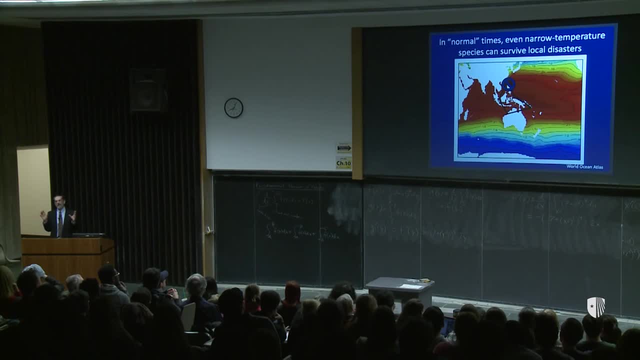 plenty of populations that have never been touched by that typhoon. So for many situations, under normal circumstances, broad geographic range, even if you don't have a lot of temperature tolerance, will get you out of a lot of jams. Dr David Shulman PhD, If you're very localized, that typhoon might just completely 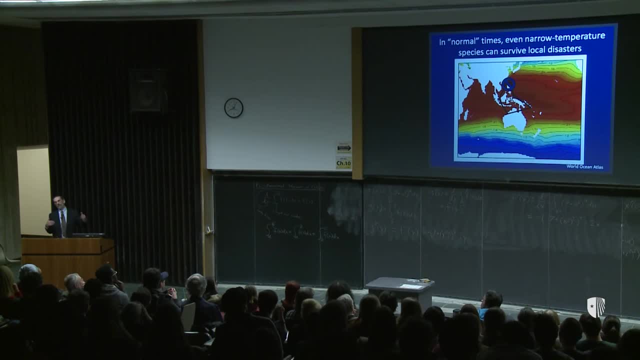 obliterate your habitat, But if you're widespread it's cool. You can handle that. Even if you entirely wipe out the Philippines populations, you've still got that Borneo population, the Java population, the Australian population, the New Guinea population to carry on. the. 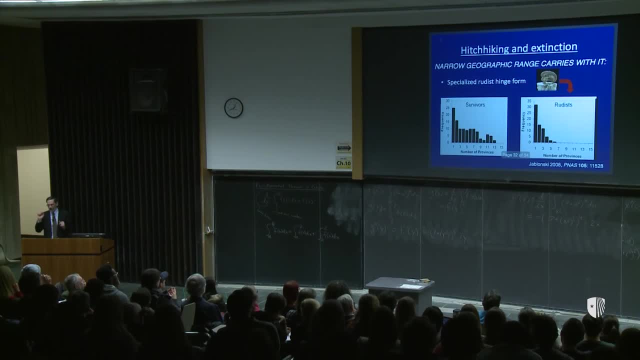 evolutionary lineage, But during a mass extinction. that's not likely to be true, right? If you drop a rock out of the sky and completely change, Dr David Shulman PhD- the composition of the oceans, completely change the global. 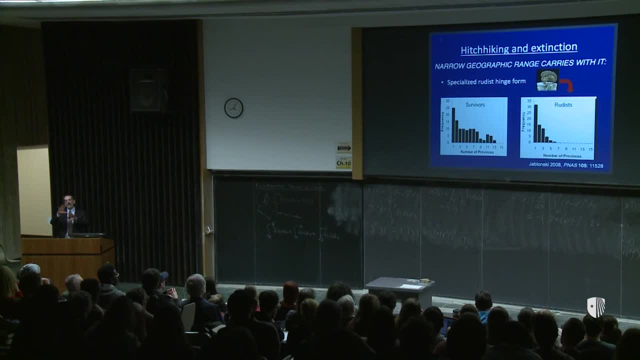 climate, then you've got a problem which only scattering your evolutionary lineages across many areas will get you through. But if geographic range is the key to survival, that means that it can carry with it many other lineages, many other properties that Darwin actually would have thought would have been very important and were very important. 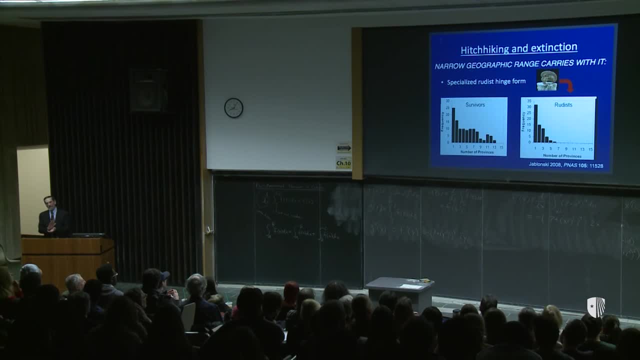 during normal times, Dr David Shulman, PhD, For example. remember that fancy hinge that I showed you for the reef-like bivalves that I called rudists. Turns out that rudists, which are completely lost at the mass extinction, have an unusually narrow set of geographic ranges. So the chances 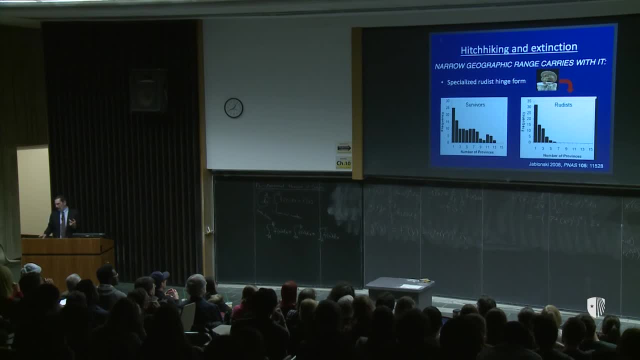 are that that exquisite adaptation of their hinge structure was lost not because of a bad idea, not because it was maladaptive on a day-to-day basis, but because it happened to be linked to a property narrow geographic range that set them up for extinction when 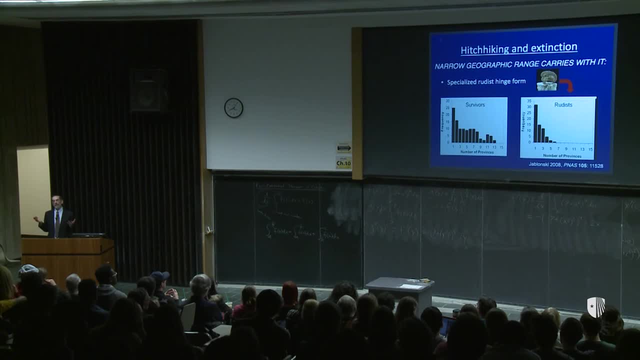 the rock fell out of the sky and the rules of extinction and survival changed, and the chances are that many adaptations that are exquisite in their normal context were lost that way by hitchhiking on geographic range size, So that, for example, remember the specialized 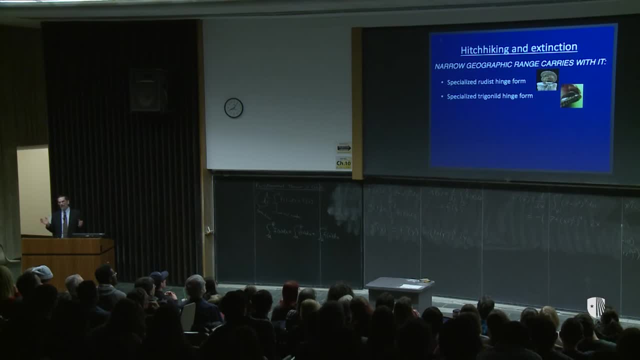 trigonian hinge that I showed you, the Tennessee State fossil. They don't quite go entirely extinct but they were global, Dr David Shulman PhD, global before the mass extinction and they've bottlenecked down to a handful of species. 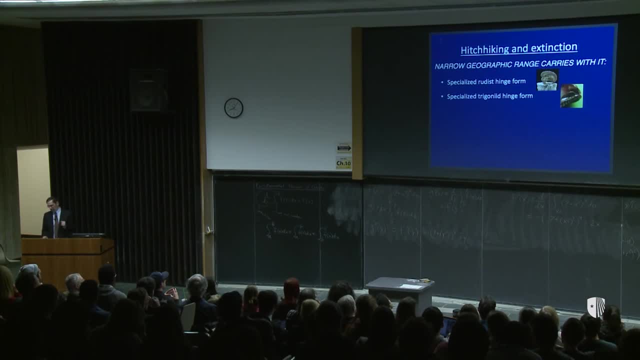 around Australia. So it's not quite gone, but almost complete. almost gone. Turns out that the complicated suchar's encephalopods, that is to say the ammonites, with their very complex internal walls compared to the pearly nautilus, which is very simple walls, it turns. out. the ammonites have very narrow geographic ranges just before the mass extinction, whereas the pearly nautilus' ancestors had very broad geographic ranges. So there's probably nothing wrong with those very complex suchars, those very complex walls inside the ammonite shell. 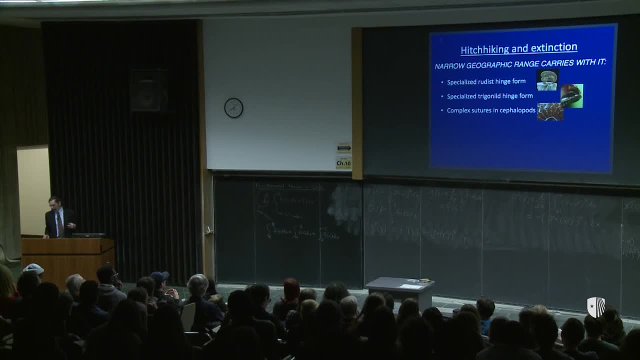 but those beautiful structures were linked to the wrong geographic range size. Turns out that complex colonies in Bryozoans, a small colonial group that builds complex architectures of colonies, the complex ones happen to have narrow geographic ranges, The simple ones tended to have broad geographic ranges, And you can guess what happened to. the complex colonies. during the mass extinctions of the Paleozoic They disappeared and apparently re-evolved from the simple colonies millions of years later, when they reappeared in the Mesozoic, And even speciation rate- rates of production of new species is, in fact, related. 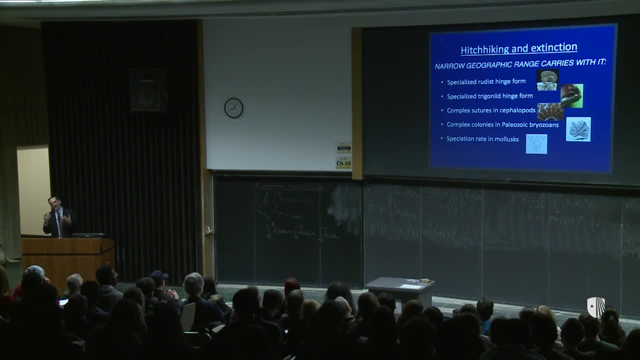 to geographic range size, which means, of course, that if you lose lineages according to their geographic range size, you'll actually change the originality of the species, And that's what we're going to talk about today. It's a combination rate of the biota, Not because there are adaptations, specifically. related to high speciation rates that are disadvantageous, but it's because that property is linked to geographic range size. So all these properties actually can get lost, not because they were poorly adapted, but because they were connected to a trait that spelled: 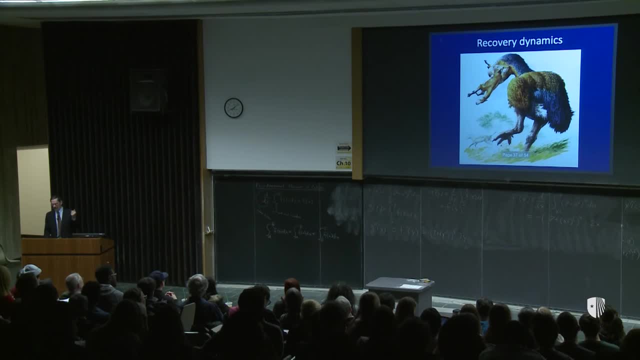 essentially doom for lineages that had those traits. But what about recoveries? I always use this slide to remind me, to point out that there are a number of properties that are linked to high speciation rates, And I'm going to point out that recoveries are not. 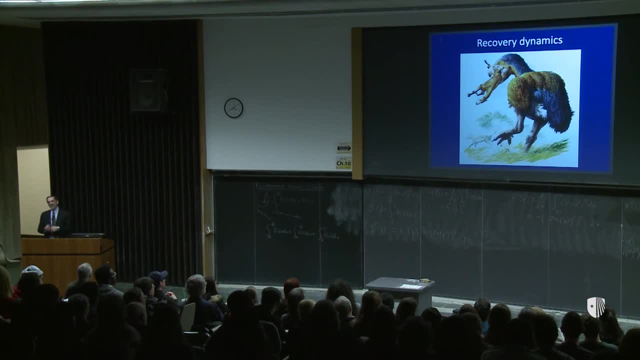 as simple as you might think. The cliché has always been: the dinosaurs go extinct, the mammals are handed the world on a silver platter and then off they go to fame and fortune and ultimately us. But it was more complicated than that because in fact, as 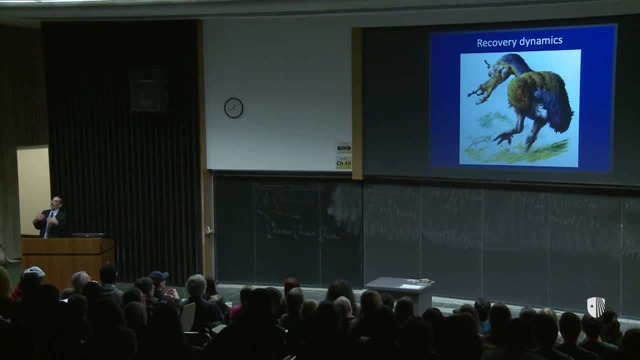 you can see here for the first 10 or 15 million- in fact more like 20 million years of the Cenozoic era, the aftermath of the dinosaur extinction. birds- flightless birds- were the top predators of the Cenozoic world after the end of Cretaceous mass extinction And 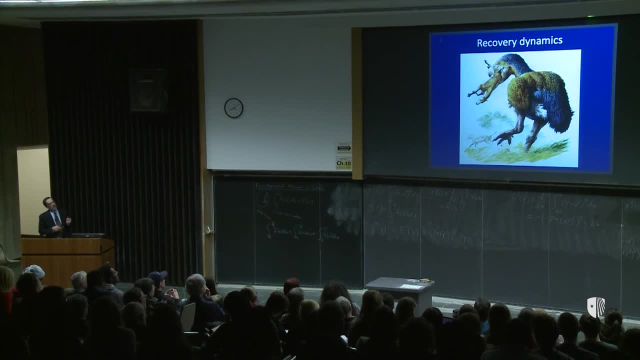 I love this drawing because, of course, what you see here is this roughly two meter-tall flightless predatory bird- that's actually related to cranes, of all things- is actually grabbing up one of the very earliest ancestors of horses. You can see the artist very carefully. 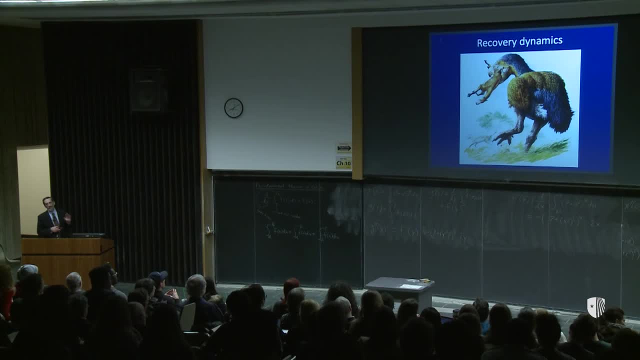 drew how the horses still had these toes when it was running around in eohippist style before the horses got bigger and evolved there, And it still does that to this day. There may have been some蜌蜖 people in the past who made their race a whole lot. that time, What will? 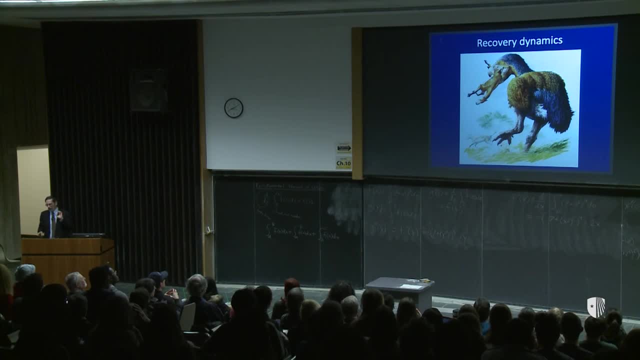 their and evolve their individual hooves. So recoveries are actually more complicated than we've given them credit to, and they're clearly an important part of the evolutionary dynamic, But we don't understand much about them at all. They've been really neglected. 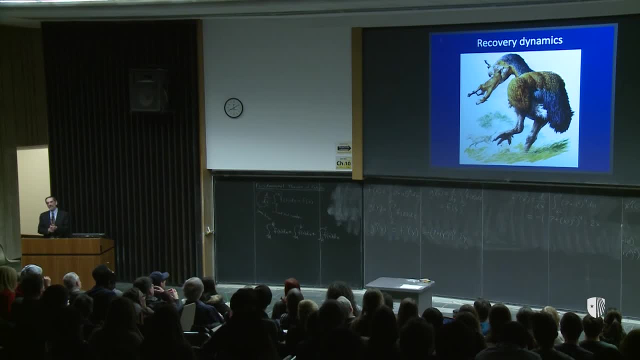 compared to the study of the bottlenecks, the big extinctions that come and then cause this pattern of differential extinction and survival. And so what my lab is actually doing now is we're starting to work on recoveries, We're starting to work on what happens when. 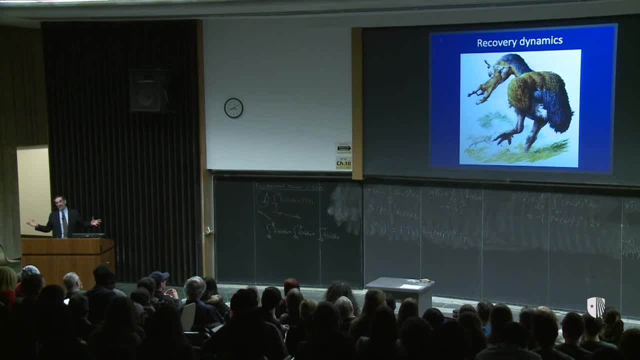 the world is partially emptied. 50 percent extinction, that's a pretty big deal. and after that partial emptying, evolutionary lineages begin to diversify again in the rebound And this in particular, this part of the talk in particular, is really going to be a progress. 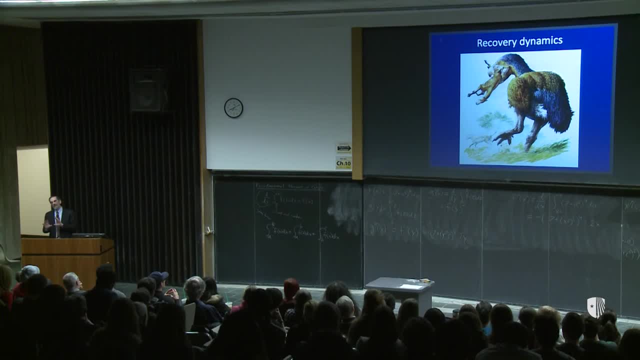 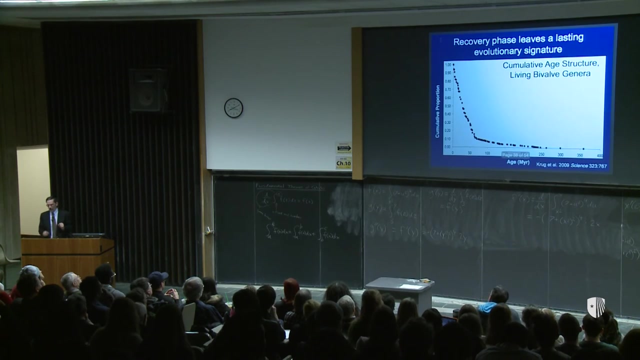 report, because we're still very much embroiled in trying to sort out even what the really major questions are And how to pose them in a way that are answerable, are not really just metaphors for how the world might work in some general conceptual sense. So the first thing I want to point out is: 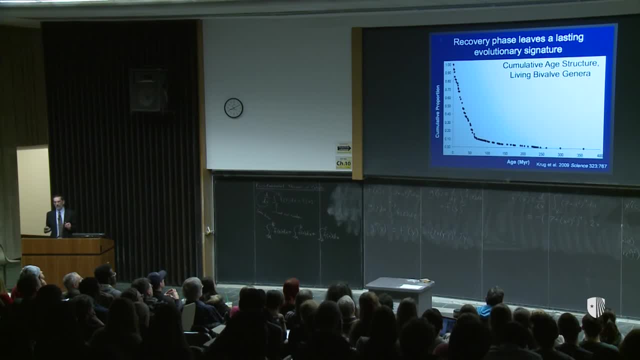 that the recovery phase leaves a lasting evolutionary signature. What I'm showing here is the age structure of living bivalve genera, the ones that are alive today. That is to say, this shows that 100 percent of the genera are alive today. 90 percent were alive 10 million years. 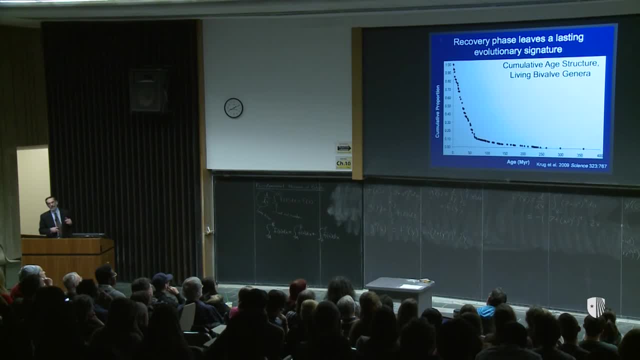 ago, 50 percent were alive. further back and so forth down the line. It's like a census of all the people living in a town. You know some of them are very young, some of them are middle-aged, some of them are quite ancient and the shape of the curve of this cumulative 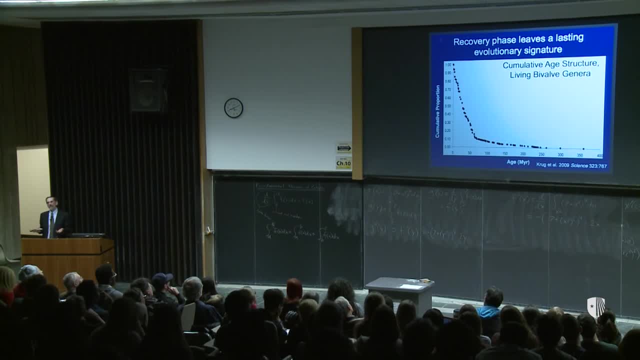 curve tells you something about the birth rates in that population, Right? so of course, we have this big bulge of baby boomers that show an acceleration of birth rates during a certain part of history, And what you see here is that you see an acceleration here too. That's actually a statistically 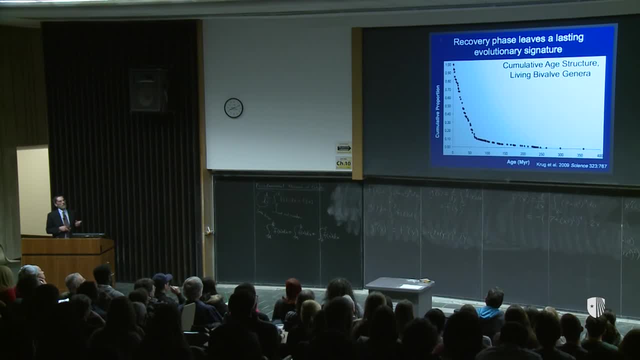 significant kink in the curve. It's not just some kind of simple exponential increase that goes into a constant doubling phase. That's actually a break in the curve, and you've probably guessed where that is. That's at the end-Cretaceous mass extinction. 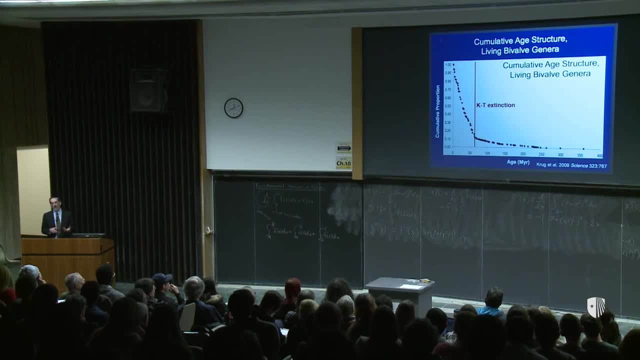 What happened after the mass extinction is that there really was an acceleration in the production of new evolution, And what's remarkable is it hasn't really died down all that much. There's actually a slight downturn there. that represents the end of the really most massive recovery phase. 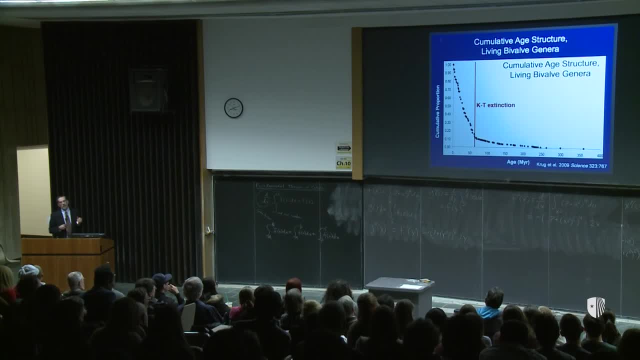 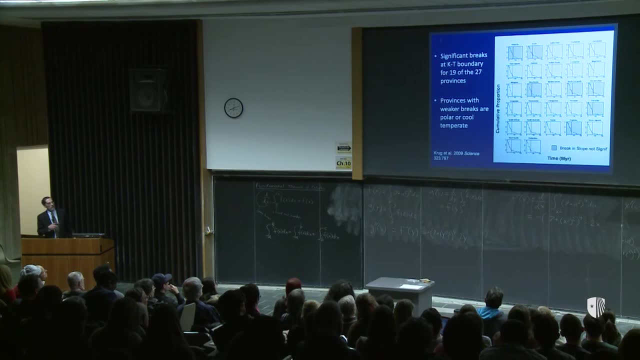 But what's remarkable is that effect carries all the way through to the present day, And what's even more remarkable is that you can see it all over the world. This is simply plots of the same kind that I showed before. It's broken down according to the large geographical areas, the biogeographic provinces throughout. 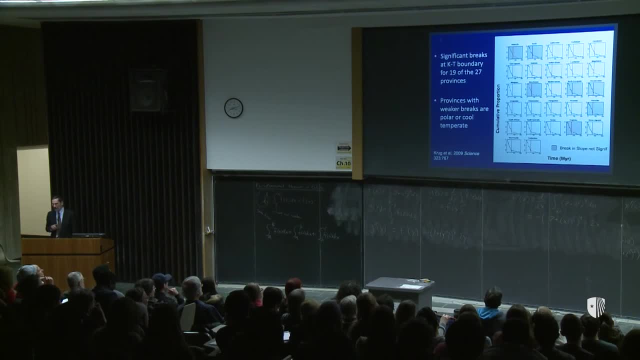 the globe, And all the ones that are white instead of shaded show, statistically speaking, that same kink. What that means is, if you go anywhere on the planet, you go to virtually any lagoon, any bay, any continental shelf. if you look at the ages of the lineages, that 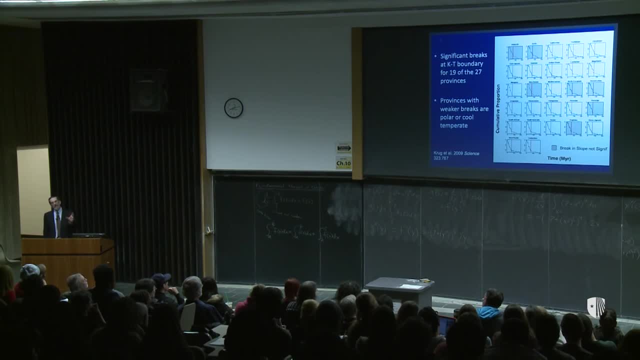 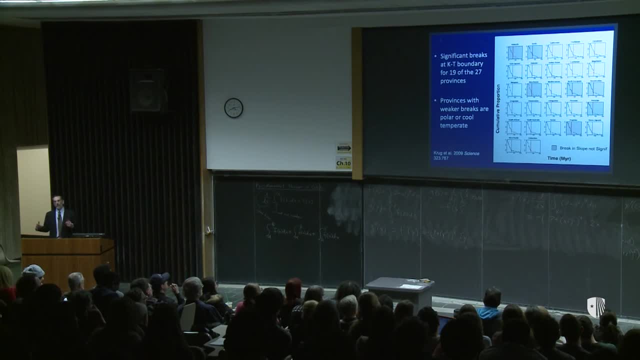 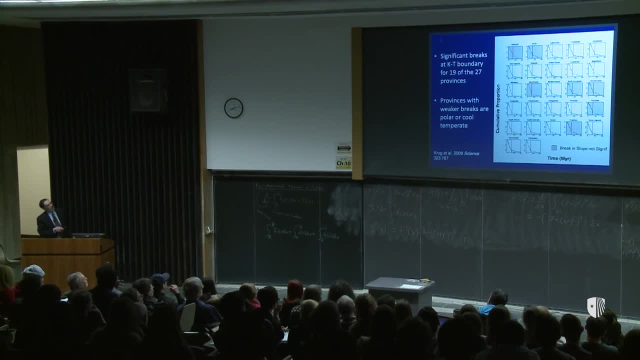 Dr James Bell ability to perceive that pattern. But even there you can see that, although it's not statistically significant, a number of those in fact do show the same kind of kink. just the numbers are lower and it's been blurred out by that effect layered on top of the mass extinction. 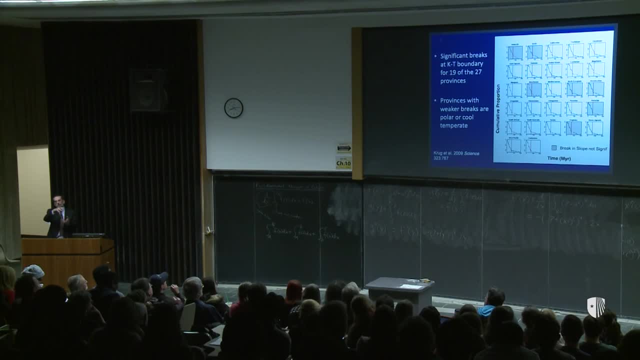 of the consequences of making those poles so cold that most lineages can't persist there. A lot of them have not died out, they simply shifted their distributions closer to the equator. Not all survivors, however, are winners, And I call this phenomenon dead-clayed. 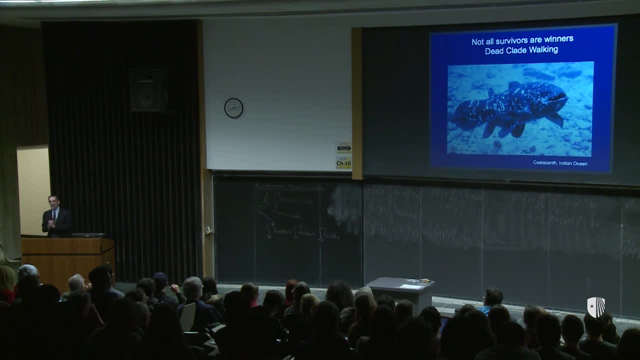 walking after a wonderful movie with Sean Penn and Susan Sarandon, And what I mean by that is that some lineages survive the extinction but never go anywhere after that. That's very puzzling, right, Because if what we think happens after a mass extinction is as I said, 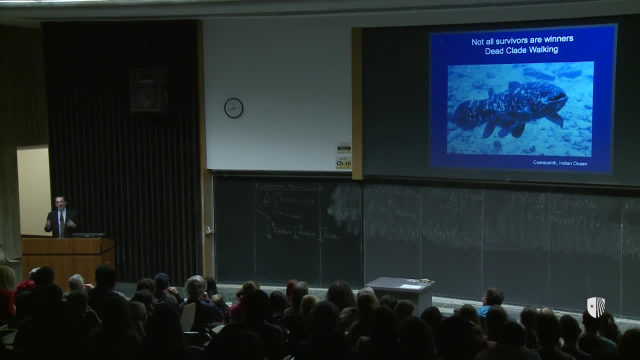 the survivors come sort of blinking out of the smoke and wreckage and they're handed the new world and they're going to die. But I think the reason why this is so important is because there are some linesages that in the future will continue to live on a silver platter. There are all these open ecological 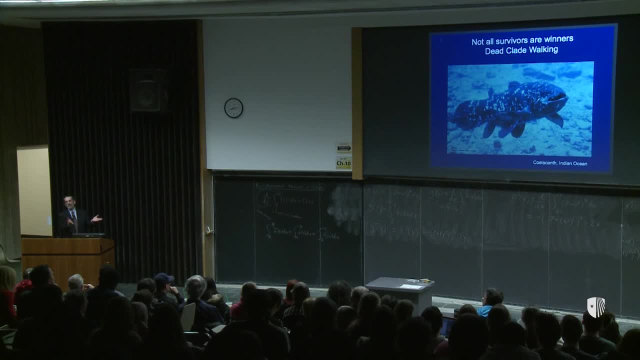 niches. the dinosaurs, birds aside, are gone. The rudas are gone, so the carls get to come back into the carl reefs. It seems as if there should be just boundless opportunity, But it doesn't actually work that way, apparently. Some lineages, of course, do indeed go on. 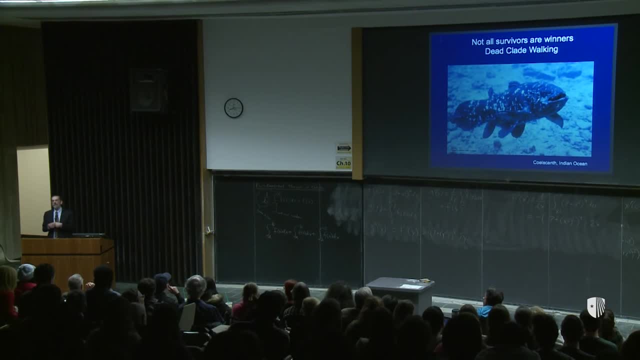 to fame and evolutionary fortune. But other lineages remain marginalized, Some of them 15 or 20 million years and then sort of pathetically dwindle off into ultimate extinction- Probably sort of collateral damage from the original mass extinction event, and that they somehow 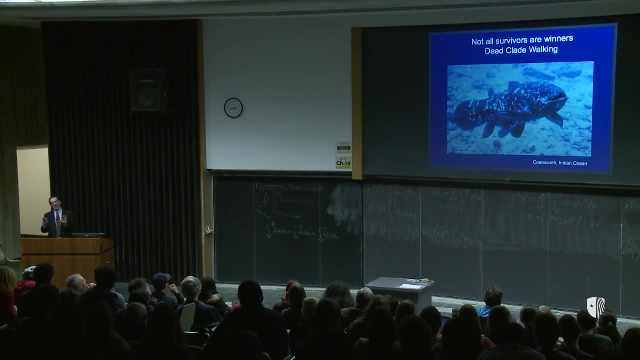 managed to hang on a little bit longer, but couldn't hack it. On the other hand, some lineage that we call living fossils, some of these so-called dead clay walkings. they actually make it to the present day. We call those living fossils And coelacanths like 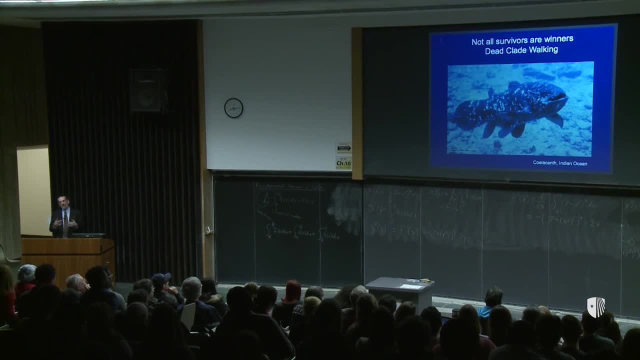 the one I showed here is a great example of that. They were very diverse, very widespread in the Mesozoic, but ever since the extinction, as far as we could tell, they've been confined to deep water in the Indian Ocean, and just one or two species at best. And of course, 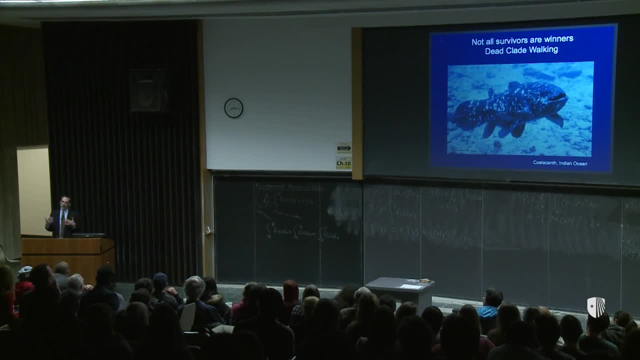 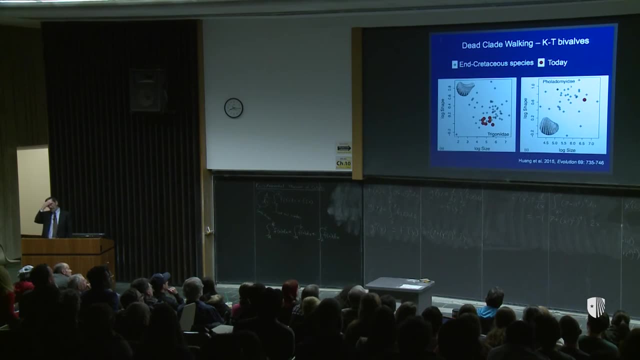 in the long run, one or two species are ultimately probably doomed to extinction- just statistically, if nothing else, let alone further environmental changes. What's interesting about this dead clay walking phenomenon? there's not only the fact that there's a number of species, but it's also the kinds of forms they exhibit. So I plotted. 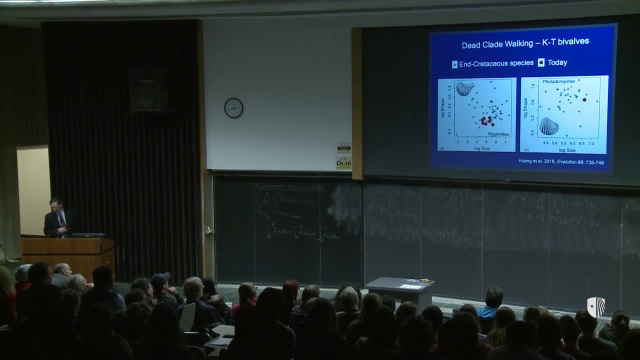 here two simple axes: size on this axis and then a measure of shape on this axis. And what you see here, there's my trigonians with the fancy hinge. What you see here is the full range of sizes and shapes that they occupied just before the mass extinction. And what 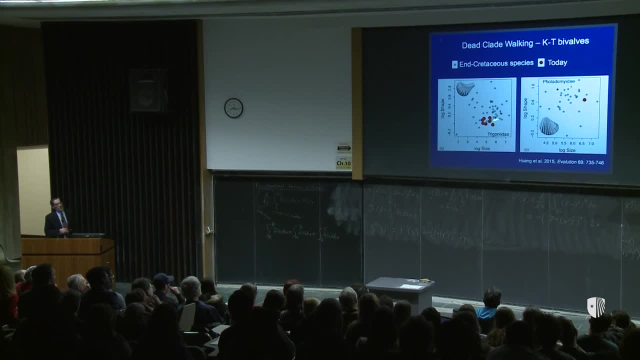 you see, here is the range of shapes and sizes they occupy today. See what happened? There used to be a flourishing, very healthy clade, very widespread, not only in space but also according to the sizes and shapes they exhibited, And they've just been crunched down to this narrow little range. 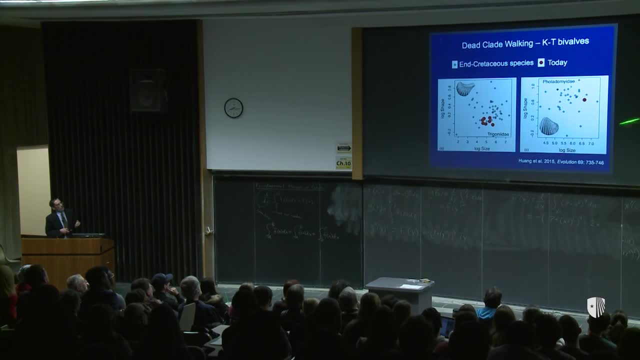 and never come back. Similarly you can see- here's another group again. size and shape. You see, they're very widely distributed in that size-shape space, but they've dwindled down to a single pitiful species. now One little spot in that very broad space just. 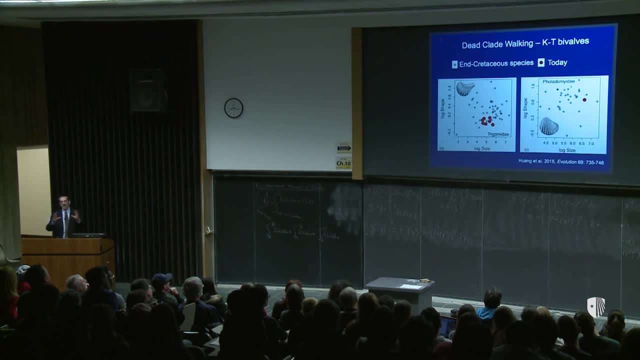 a mere shadow of their former selves. They've been, they were doing very well, you know, five minutes before the asteroid hit, but as far as we can tell, they've just dwindled down and they've never been diverse ever since. So clearly these. there's two kinds of lineages in these mass extinction. 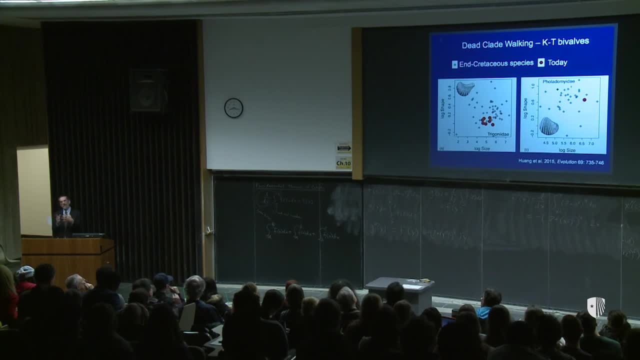 situations. They're the ones that survive and then rebound quickly to flourish, and ones that never get traction again. And I'll say flat out: we don't know why, We don't know why. To me that's one of the really interesting next generation of evolutionary. 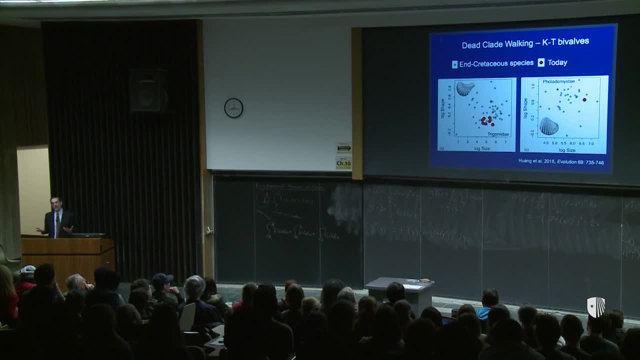 questions And we've tried many different hypotheses to test these and none of them have really panned out. It's really interesting, it's really challenging, So that, for example, remember how I said that during normal times, as presumably these post-extinction intervals, are lineages with lots of species fare better, right, Just think about it. they're buffered against random events that might knock out a few species here and there, but with many species present they can survive. But that's not true across the mass extinction boundary. 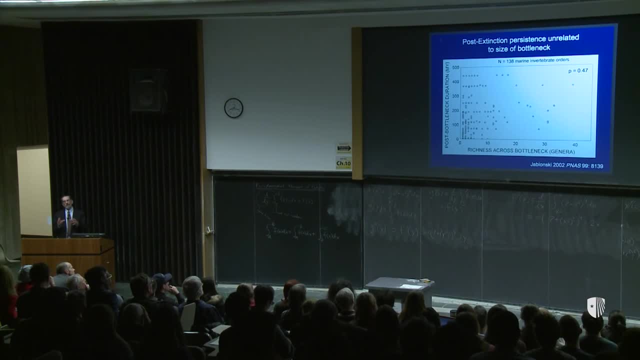 So you can see here this is the size of the bottleneck across all the mass extinction boundaries through the history of life, across the big five plotted by the major evolutionary groups, what I call the marine invertebrate orders, which are higher groups like sand. 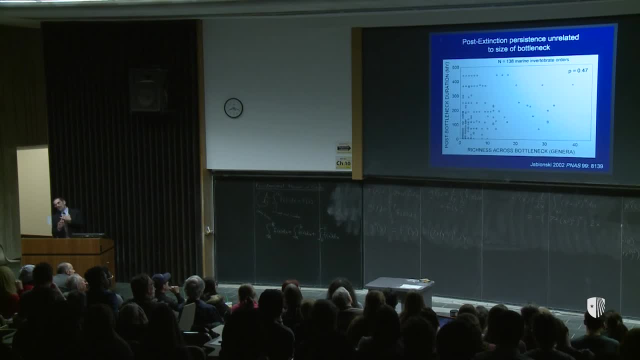 dollars and brittle stars and hard urchins and reef-building corals, the really major groups, And what I did was I counted how many of their lineages got across the boundary, Because a really obvious hypothesis would have been that the lineages that got through relatively unscathed, perhaps because they were more widespread. those guys would have preferentially then rapidly rebounded, And the ones that just barely eeked it through, those are the ones that would have just gone down in the post-extinction scramble for recovering. 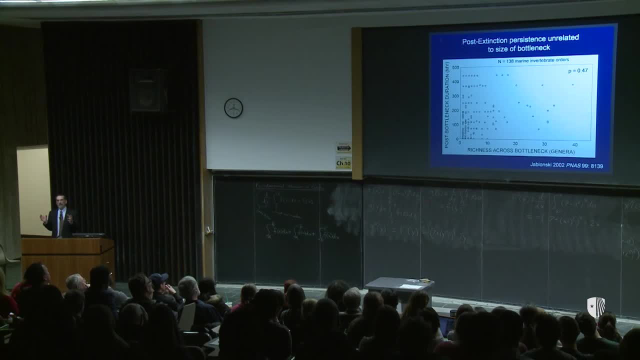 for evolutionary recovery. But it's not true. This is a shotgun blast of data points, just a scatter. a scatter of points that have no statistical pattern whatsoever. It's not often that you get to publish in a fairly august journal a plot that is a shotgun blast with. 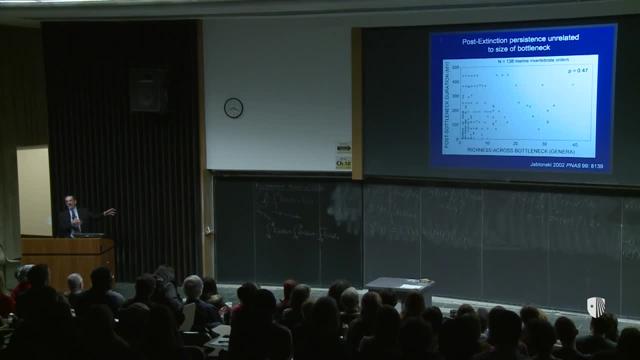 no statistical significance whatsoever. So in many ways I feel this is quite a triumph to actually find biological meaning in a result that involves no statistical correlation whatsoever, Because that failure to show a statistical correlation shows that our simple scenario for how the dead-clade walking phenomenon 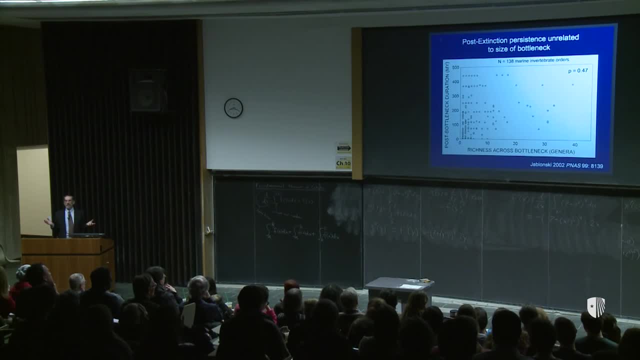 could work. it turns out that's not true. In fact, I guess I've got a minute, so I'm going to tell you one personal anecdote about that. I actually got from this august journal a pushback about the term dead-clade walking. I was told by the editors that it was too. 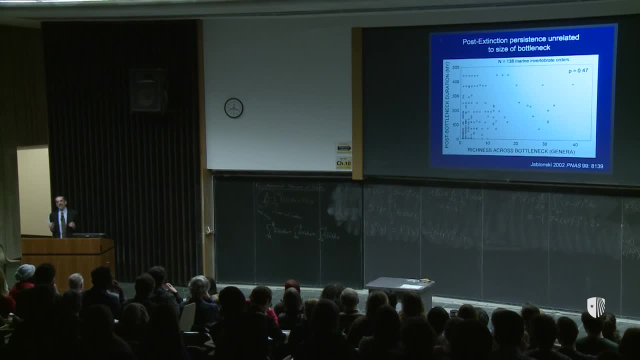 irreverent for the sage pages of this particular journal, And I then pointed out to them that they were publishing papers about the evolution of fruit flies that used that named a mutation that removed the, that destroyed the heart of the fly, Tin Man from the Wizard of Oz. 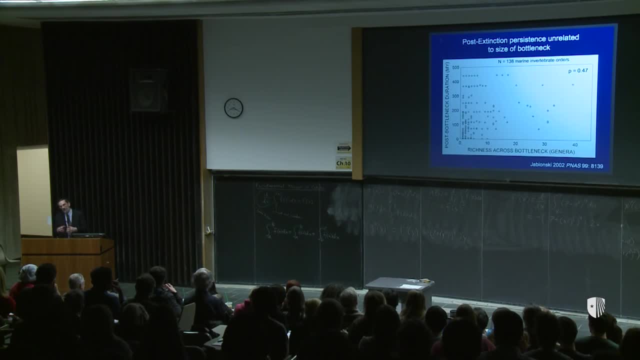 They used, another they used. there was another mutation that was called Bagpipe, because of the way, because of the way the fly larva was deformed And I don't want to tell you what the fly larva looked like for the mutation that was called Hedgehog, And of course not. 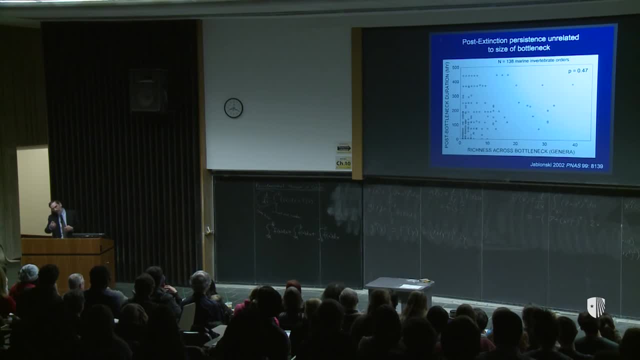 only that, there were even. there were even mutations of Hedgehog, called Sonic Hedgehog, after the cartoon character. So I said: you're telling me you're publishing papers about Tin Man and you won't let me use dead-clade walking. And so in fact they actually relented. 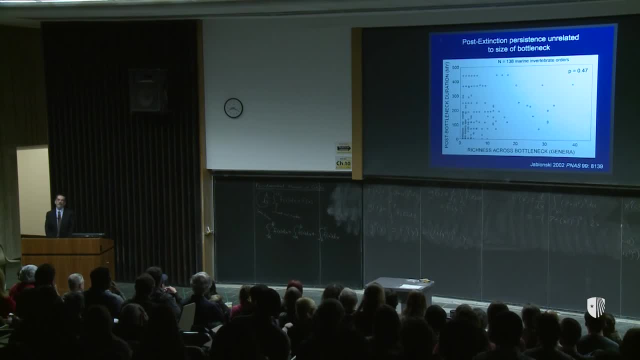 And that was actually. although that's a funny anecdote, it's actually important to remember. Words are very important to scientists And it's very difficult to engage your colleagues in studying a phenomenon unless you've named it, unless you put a name on it and you could explain it in a relatively few simple words. 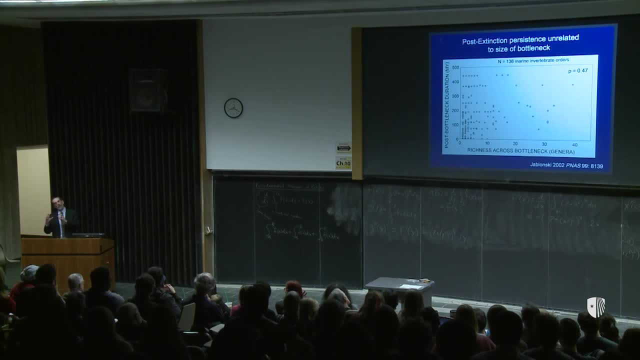 And so what I wanted to do was name this phenomenon, because I thought it was actually really important that not all survivors of mass extinctions are winners, And so I- but I did have to fight with the editors of the journal to let me put the name on, But I'm happy I it it came. 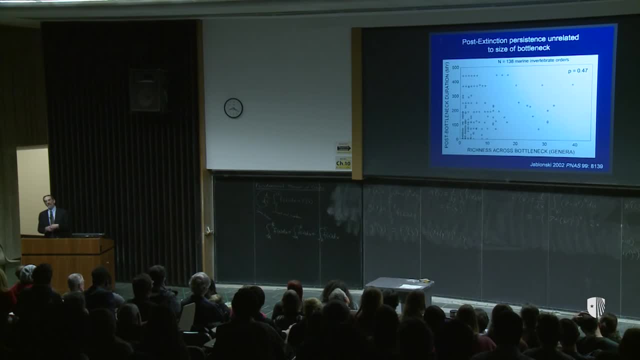 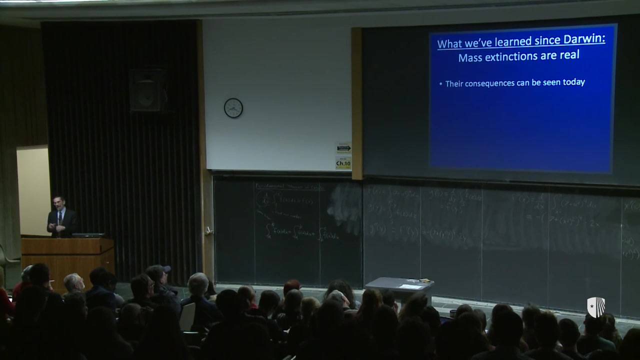 across because in fact there's actually, if you, if you now Google it, there's actually several hundred papers that talk about this general phenomenon, So it was worth the fight. So what have we learned since Darwin? We've learned a lot of things, And I'd like to think: 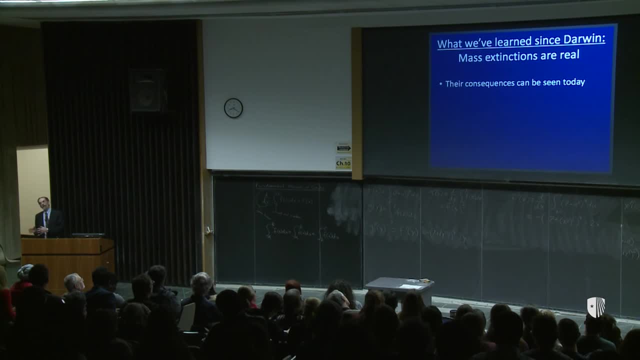 that Charles would be proud that we kept building on his foundation even when we found exceptions to his general observations. Mass extinctions are real things. They're it's been, they've been confirmed so many times On so many different scales in so many different places for so many different organisms that 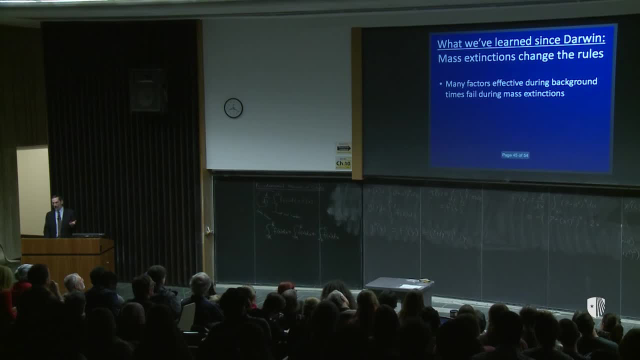 is incontestable And their consequences can be seen today. Many factors that were effective during background times failed during mass extinctions, because mass extinctions change the rules of extinction and survival And that's why they're it's they're so effective. as evolutionary agents. Not only do they bite deep into the ecosystems of the time, but traits that have been important for tens of thousands of years, Tens of millions of years up to that point, are ineffective. And geographic range comes to the fore, allowing hitchhiking effects, so that traits that were perfectly well adapted. 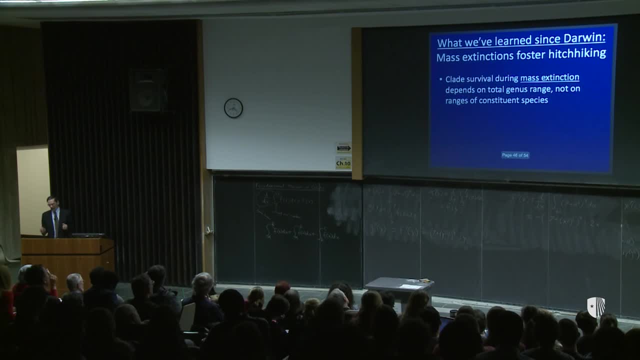 can be lost because they were linked to the wrong scale of geographic range, Because they foster this hitchhiking, as I said, claimed survival during those extinctions. because it depends on total range, not on the ranges of constituent species, and that means that these traits can be lost or survive because of hitchhiking. You can imagine many traits that were less perfect than some of the others that were lost will survive simply because there they were in the widespread lineages, And recoveries are unpredictable- Not all. 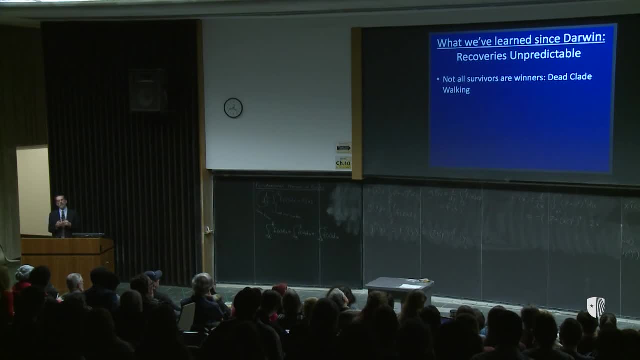 survivors are winners. As I said, the dead clay walking phenomenon is fascinating and it's troubling. It's troubling not just in theoretical terms. right, It's exciting. It's a question we don't know the answer to, and what could be more fun for a scientist than? 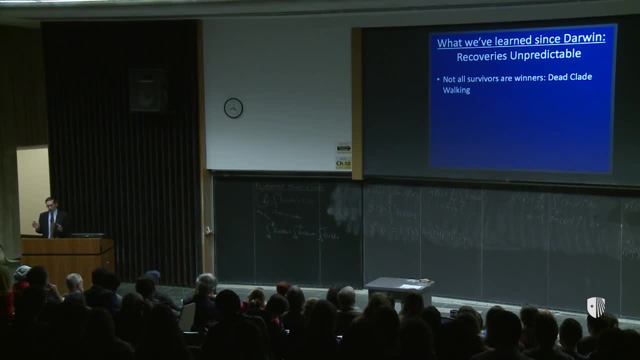 a big question that we don't know the answer to, And it's a question we don't know the answer to, And so I'll enjoy studying this. but it's disturbing for other reasons, Because, of course, if we want to think about what's going to happen to the biosphere today, what's 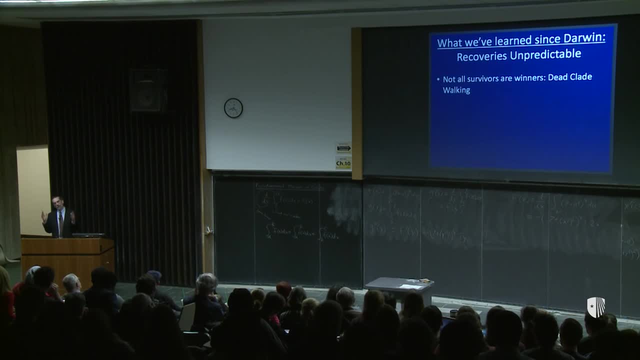 going to happen to biodiversity today, assuming that we could put the brakes on the many stresses that we're imposing on today's biota. it sure would be nice to know something about what helps lineages recover from pressures or bottlenecks, and what is it that makes them recover from. 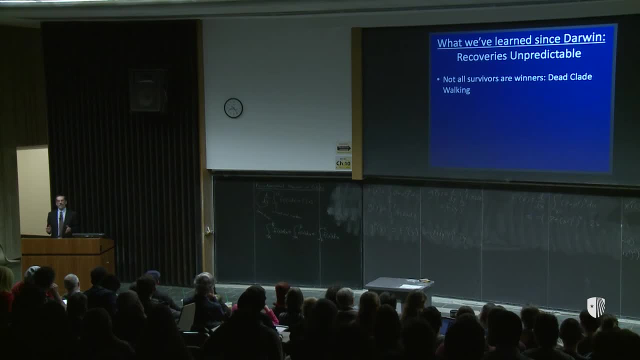 pressures or bottlenecks, and what is it that makes lineages less likely to recover from those bottlenecks? So that means this has not just a theoretical implication, but it really says something about something we really want to know the answer to for the long-term. 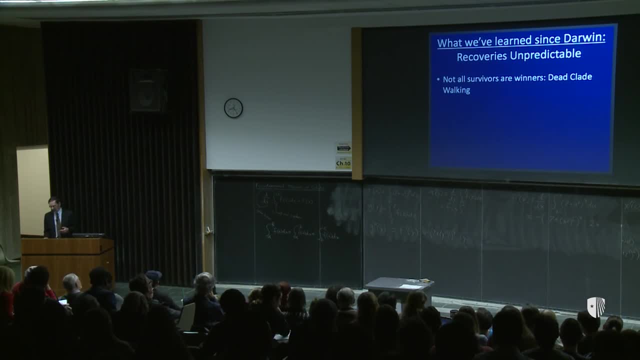 biological health of the planet. And, of course, this post-extinction success not being protected by bottleneck size means that some of the simplest rules that we might have thought were going to work simply don't work. It's an open question. So what we've learned from? 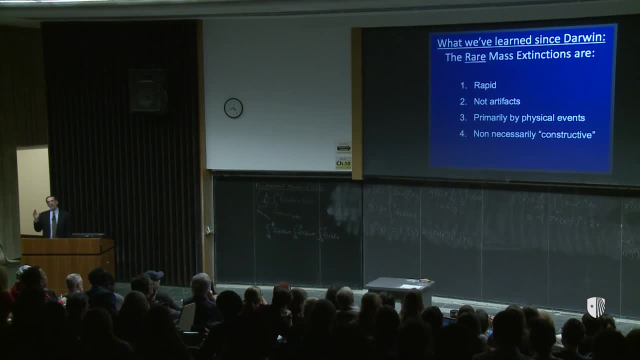 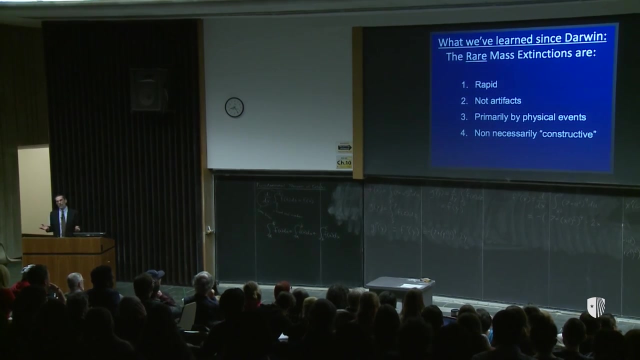 Darwin Since Darwin's times is, although he was almost certainly right about the roles of extinction in the process of natural selection during normal times, under many circumstances- And remember normal times- represent 99.9% of geologic history and in fact actually probably represents. 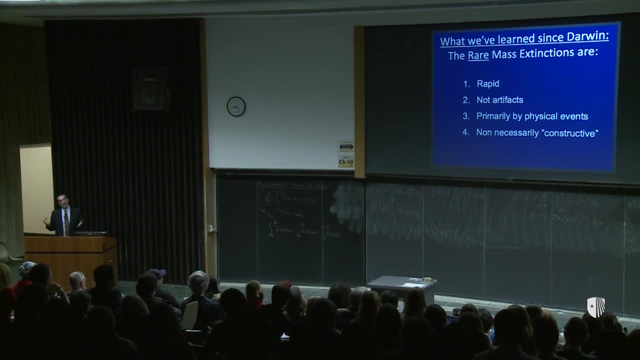 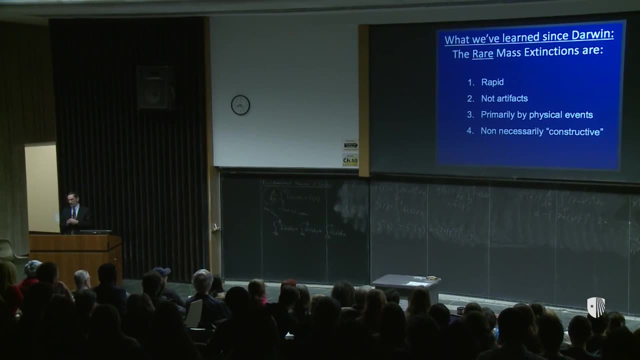 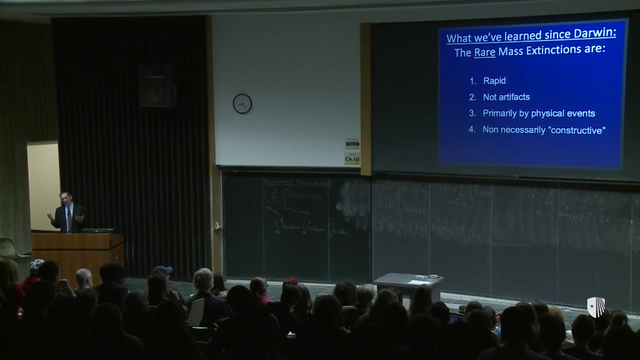 something like 90% of the extinction And yet because of the changes in the rules that 10% extinction, those severe episodes can redirect evolutionary trends. So the rare evolutions were rapid. They're not artifacts. It's pretty clear that primarily by physical 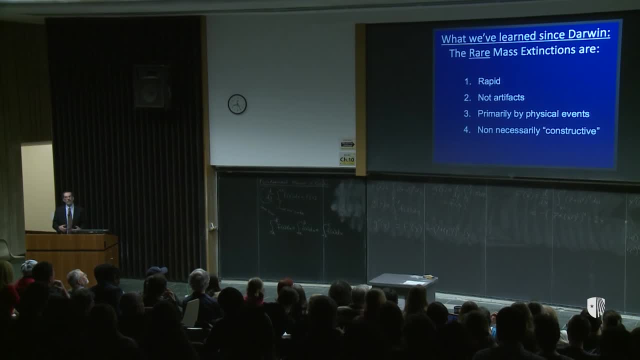 events- rocks falling out of the sky, ice ages, volcanic eruptions, changes in ocean chemistry, changes in atmospheric chemistry- and they're not necessarily constructive. They're selective in the sense that the survivorship isn't purely random, But, as I've said, probably. 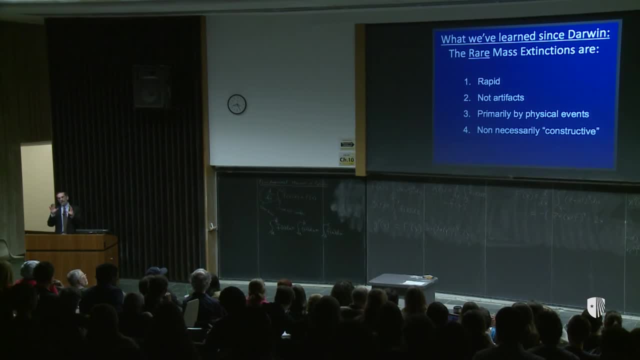 more times. you're probably getting tired of it by now. That doesn't mean that survivors that that are being selected are being selected in any way that that connects to the reasons they thrive during the 99.9% time of geolo, percent of geologic time that we mostly study. 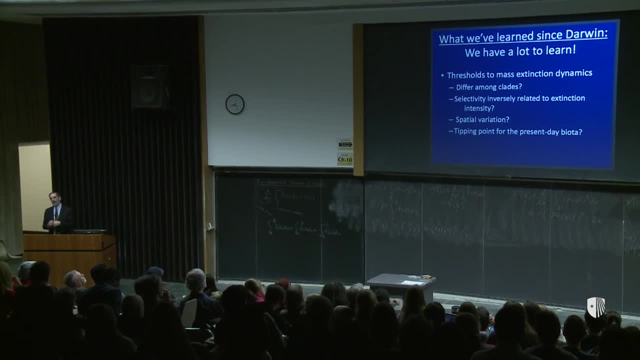 We also have a lot to learn And, believe me, I could go on for hours about what we have a lot to learn. But for example, just to take one little chunk of that, Is it possible- there are thresholds to that- switch from normal extinction times. 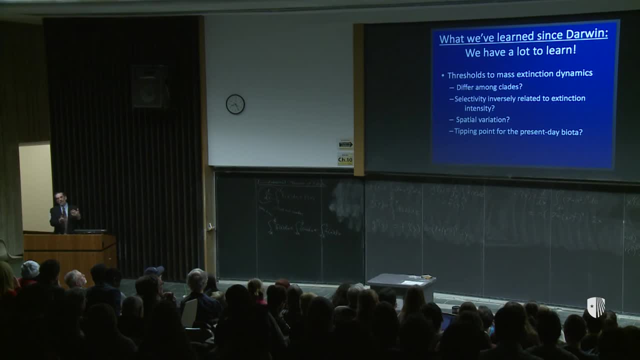 When all those traits that I talked about, like abundance and body size, are important, And mass extinction times, where geographic range of clades is the key factor. Geographic range for clades probably matters all the time, But everything else melts away during these mass extinctions. Does that threshold for melting away differ among clades For? 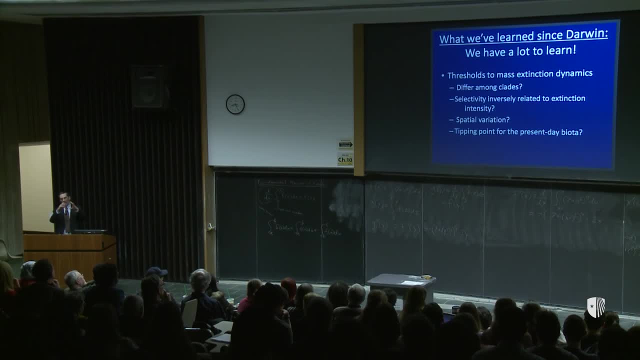 example, it seems that those ammonites, the cephalopods with the very fancy sutures, it seems that if you look at them wrong, they have a mass extinction factor And that's because they have a mass extinction, You know they. they're, on the other hand, the 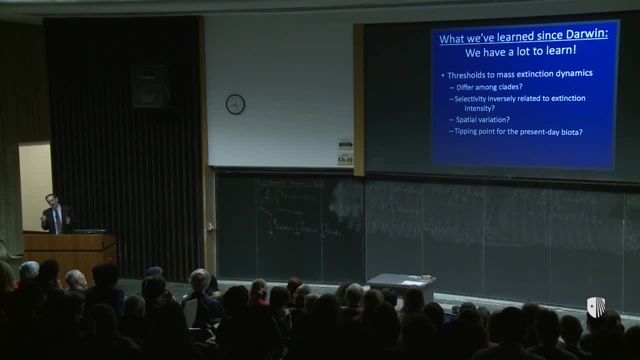 phlegmatic bivalves that I look at just trundle along through most of geologic time, And it does in fact take a 10 kilometer rock falling out of the sky before they even notice. And so there's obviously a difference among clades And that's really interesting. And again, 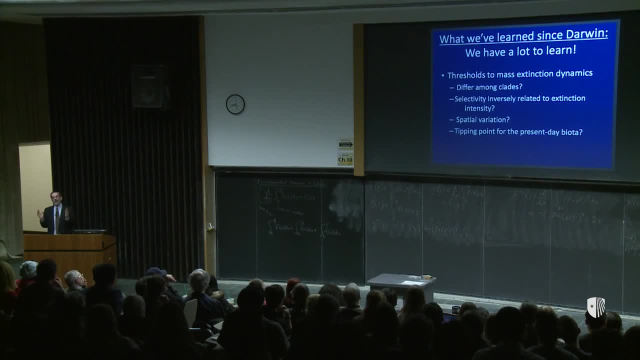 really important for the kinds of patterns that we want to understand in the biosphere today? Is sea activity inversely related to extinction intensity- Maybe the worst the extinction gets. As you go on, you'll get a lot of questions. What's the best way to? 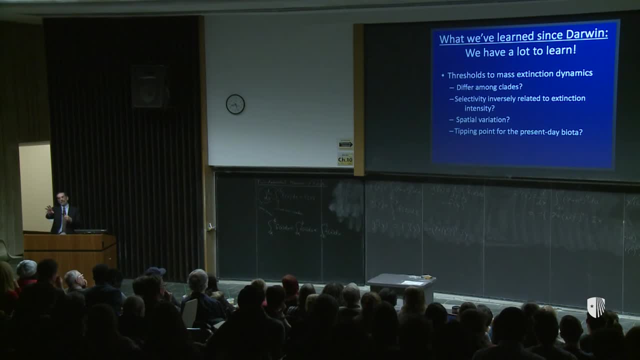 explain that? Well, the best way to explain extinction intensity is to turn up that extinction intensity dial. Maybe that's just a threshold effect. Then you just click over and the other kind of extinction works. Is there spatial variation? Are the tropics hit worse than the poles? Or are there special refugia where, for some reason, some small corner of the world is left in peace during these big mass extinction upheavals? In theory that's one way to explain that broad geographic range effect. I don't think it's true, but you never know for other. 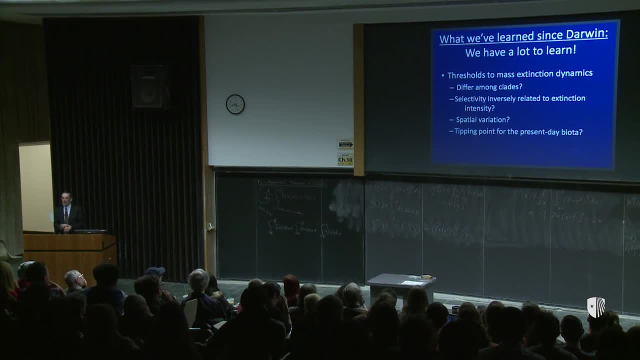 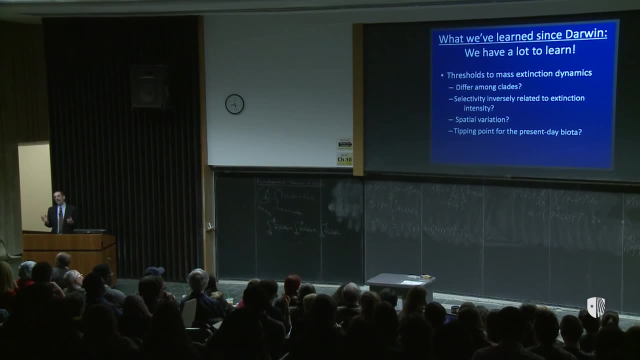 groups. And, of course, the last big question that I'm going to really leave you with is: where is the tipping point for the present-day biota? There's a lot of talk about a sixth extinction And I'm very happy to report that, from a paleontological point of view, we're 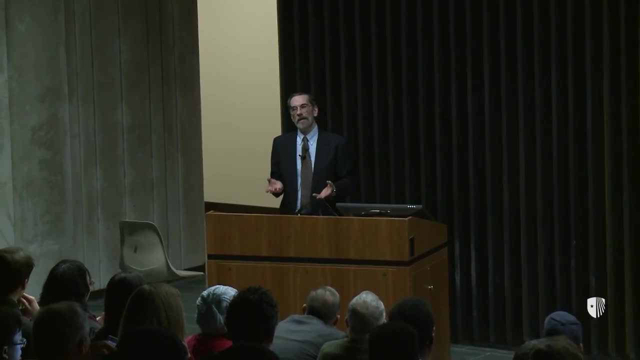 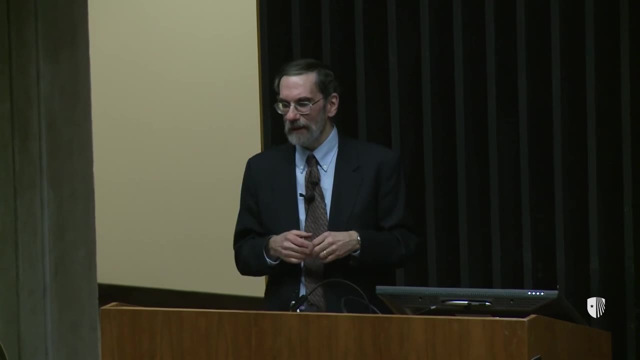 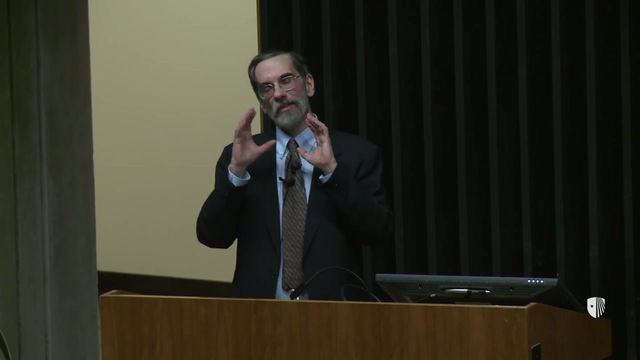 not there yet, which is good news. On the other hand, there are many pressures on today's biota. Just to give you one catalog: Consider the spatial scale of human impacts in the ocean And think about what I said about geographic range size. So you can see that. 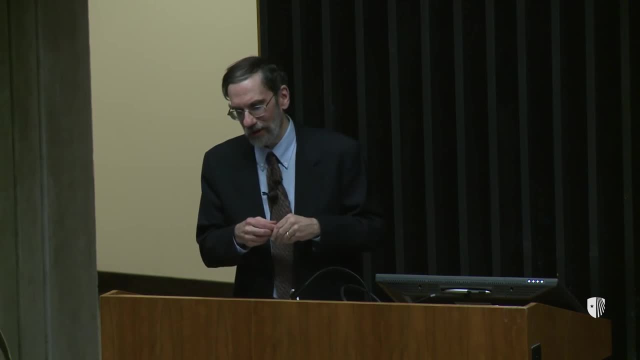 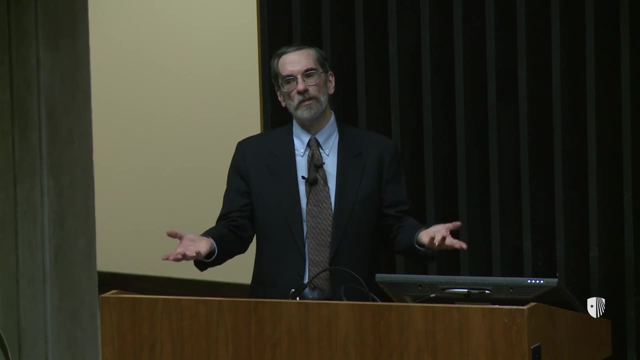 bottom trawling, although relatively localized, is becoming increasingly widespread. Shipping and the shipping lanes that drop invasive species, not to mention diseases, are concentrated in a few areas, but those areas are becoming larger all the time. Ultraviolet changes as relatively minor changes in ozone concentration in the upper atmosphere are actually becoming 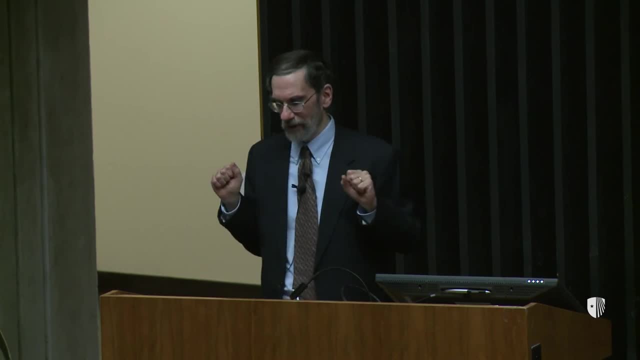 increasingly severe over broader areas of the oceans And, of course, acidifying oceans, in which the pH of the oceans change as CO2 content of the atmosphere changes is increasingly a global pattern. So the question is, when are these all going to add up into the kinds? 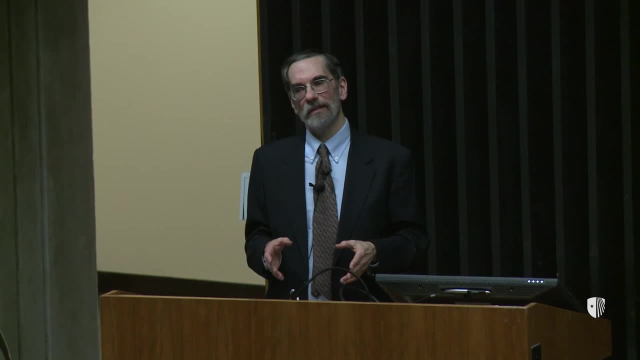 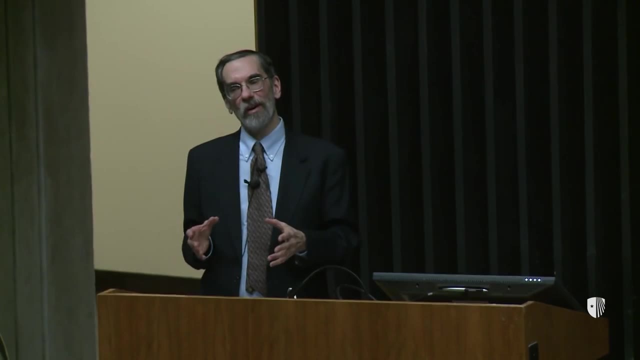 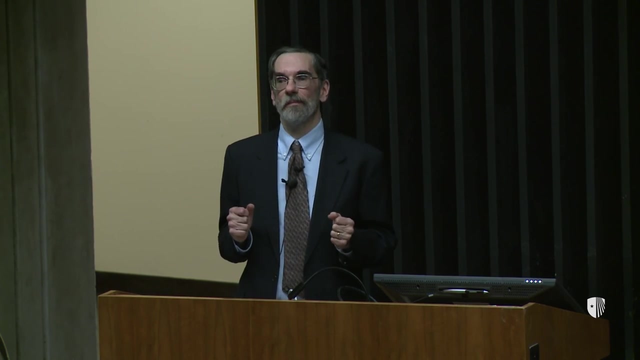 of effects that we saw at the beginning of the world's history, And I think that's a huge question And I think especially we lost that figure in the dicurcinia bịchaucimento breakfast, But at the end of the Cretaceous period, And the real answer is: we don't know yet And frankly, given what I've seen about how extinction works, We don't want to find out. We don't want to be there to run that natural experiment, or I should say that unnatural experiment, Because what's happening now, of course, is we're closing in on that kind of set of conditions. 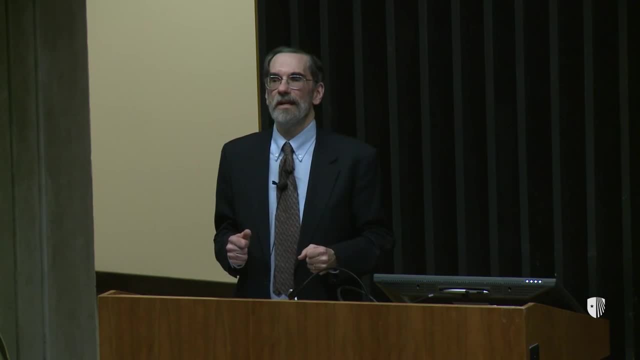 And we don't know where the threshold is gonna be, Because, if it's one thing, the fossil record ecosystems do have breaking points. They're not infinitely resilient And when they do change, they change rapidly and in unpredictable ways, And in ways, evidently, that don't necessarily. 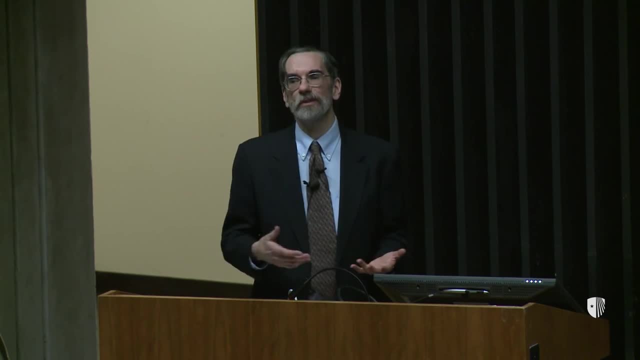 favor the kinds of traits that are favored during the normal times- Just ask the dinosaurs- And so it seems to me that our strategy now should be to minimize the effects, the spatial scale of these, in such a way that lineages can respond to those evolutionarily and spatially. 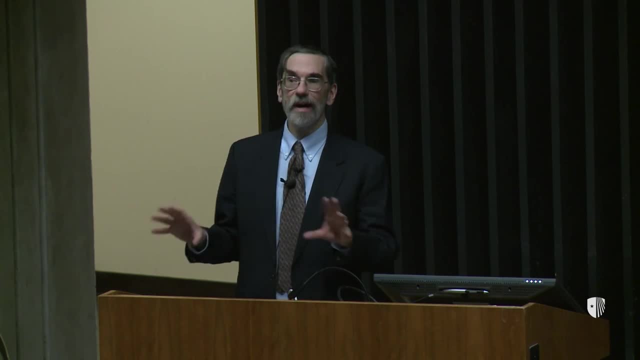 in order to cope with the kinds of changes we're imposing And if we're lucky, if we can start dialing down some of those extreme changes, then that lineages will be able to recover in a way that will actually lead to not just the health of particular species. 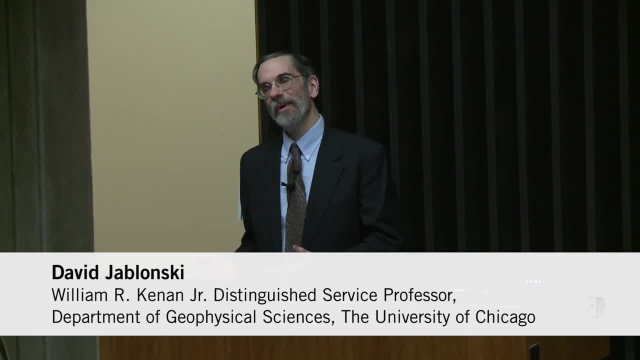 but also to the health of the evolutionary process that Darwin has allowed us to understand in such detail and with such insight. Thank you,